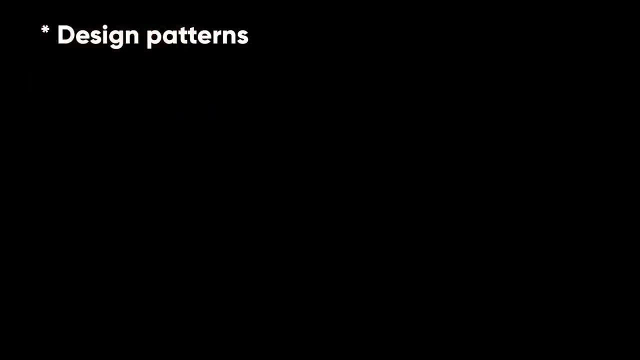 some facts. Angular presents you not only the tools but also design patterns to build your project in a maintainable way. When an Angular application is crafted properly, you don't end up with a tangle of classes and methods that are harder to modify and even harder to test. 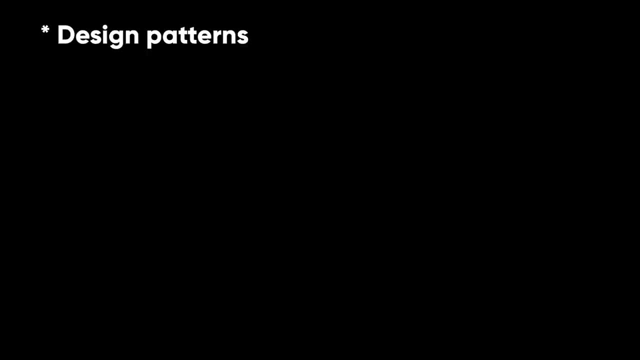 The code is structured conveniently and you won't need to spend much time in order to understand what is going on. It's JavaScript, but better. Angular is built with TypeScript, which, in turn, relies on JS ES6.. You don't need to learn a totally new language, but. 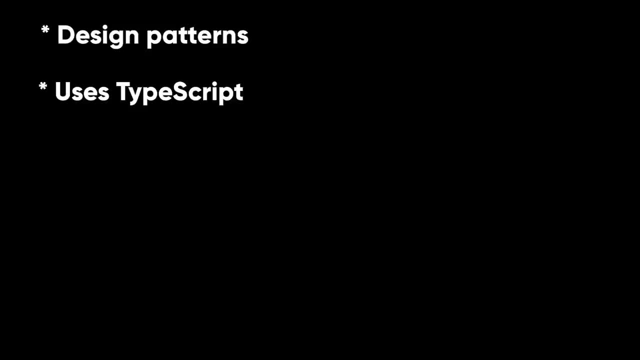 just receive features like static typing interfaces, classes, namespaces, decorators, etc. No need to reinvent the bicycle With Angular. you already have lots of tools to start crafting the application right way. You have directives to give HTML elements dynamic behavior. You can power up the forms using form. 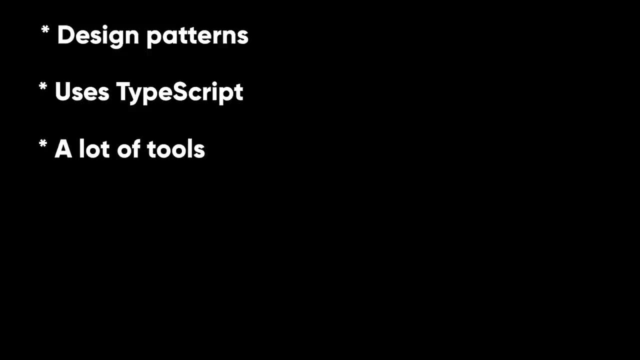 control and introduce various validation rules. You may easily send asynchronous HTTP requests of various types. You can set up routing with little hassle, And there are many more goodies that Angular can offer us. Components are decoupled. Angular strives to remove the tight coupling between various components of the application. Injection happens in Nodejs style. 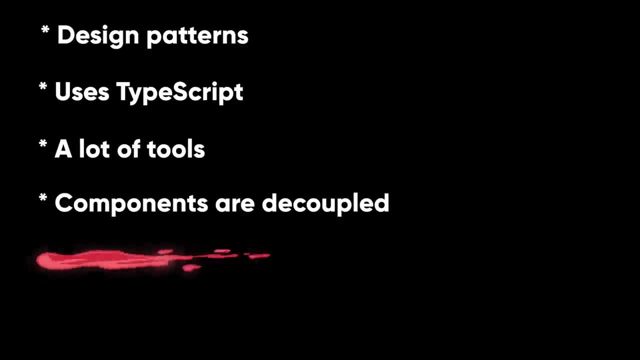 and you may replace various components with ease. All DOM manipulation happens where it should happen. With Angular, you don't tightly couple presentation and application logic, making your markup much cleaner and simpler. Testing is at the heart. Angular is meant to be thoroughly tested and it supports both unit and end to end testing. 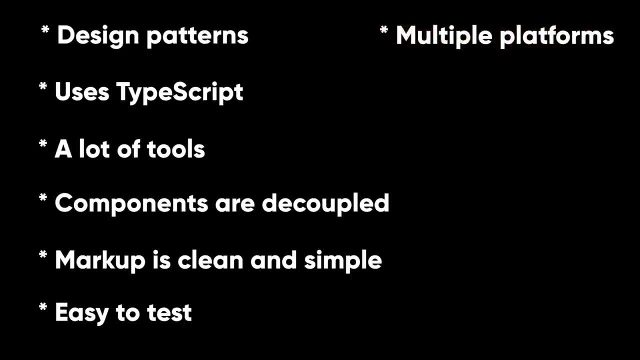 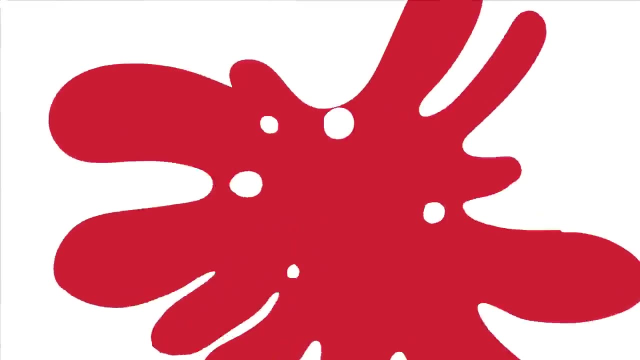 Angular is mobile and desktop ready, meaning you have one framework for multiple platforms. Angular is actively maintained and has a large community and ecosystem. You can find lots of materials on this framework, as well as many useful third party tools. The architecture diagram identifies the eight main building blocks of an Angular application. 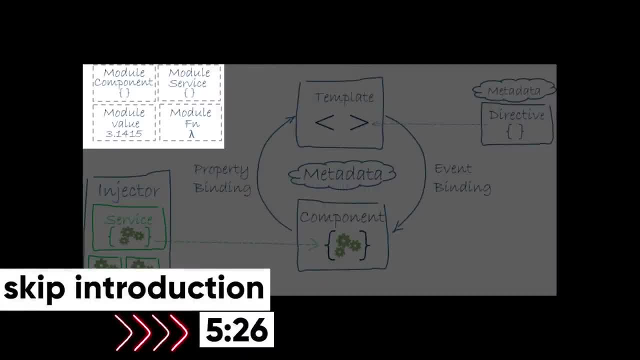 Angular apps are modular and an Angular has its own modularity system called Angular Angular modules or ng modules. Every Angular app has at least one Angular module class, the root module, conveniently named app module. While the root module may be the only module in a 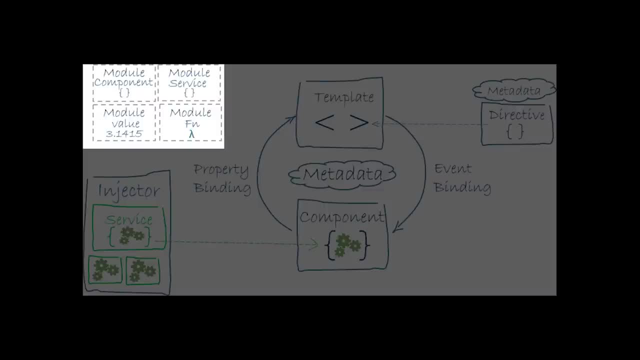 small application. most apps have many more feature modules, each a cohesive block of code dedicated to an application domain, a workflow or a closely related set of capabilities. An Angular module, whether a root or a feature, is a class with an ng module decorator. 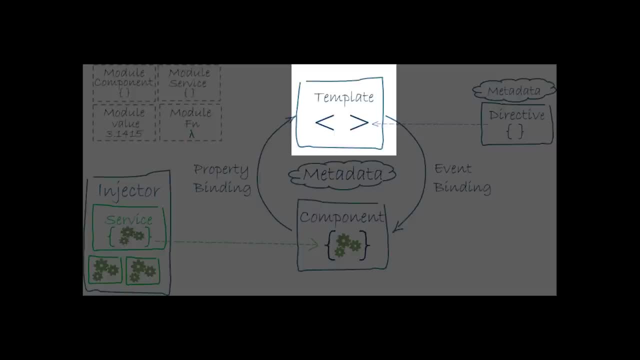 Angular templates are dynamic. When Angular renders them, it transforms the DOM according to the instructions given by directives. Metadata tells Angular how to process a class. Service is a broad category encompassing any value, function or feature that your application needs. Almost anything can be a service. A service. 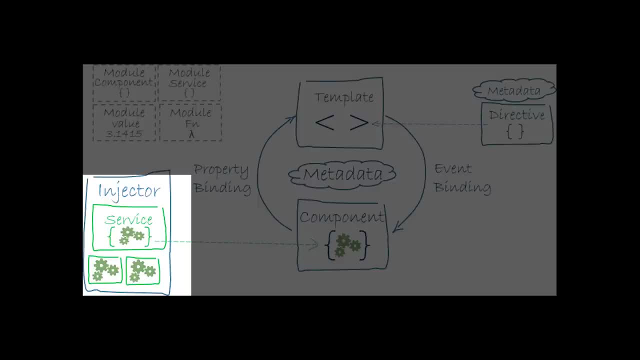 is typically a class with a narrow, well-defined purpose. It should do something specific and do it well. Examples include logging service data service message bus text calculator application configuration. There is nothing specifically about Angular services. Angular has no definition of a service. There is no service-based class and no place to register a. 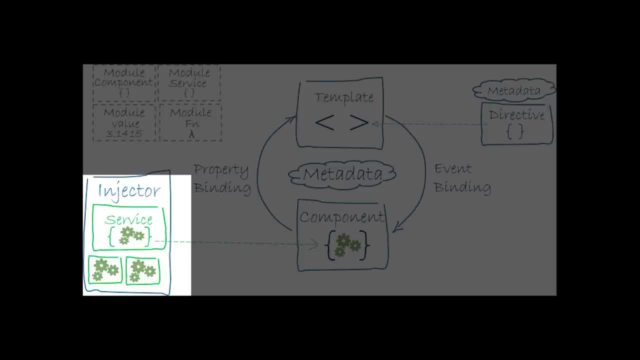 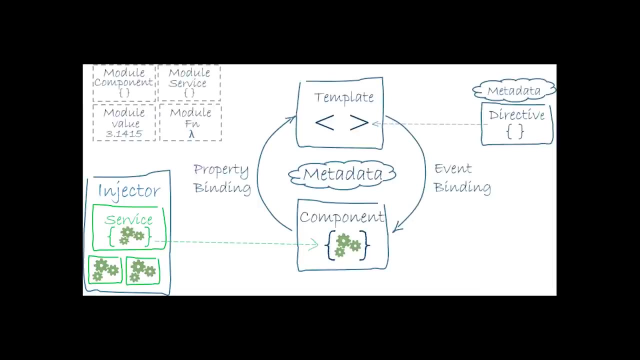 service. There is no service-based class and no place to register a service. Yet services are fundamental to any Angular application. Components are big consumers of services. Now let's talk more about components in detail. Components are the main building block of Angular. 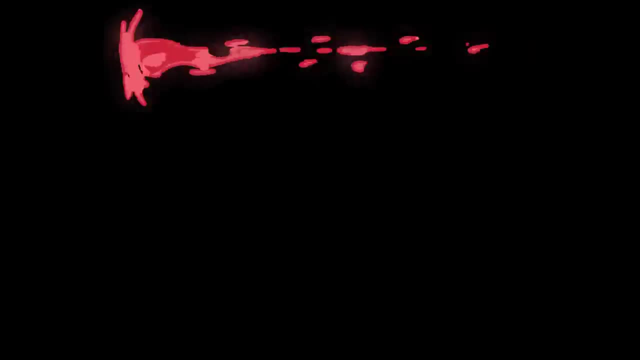 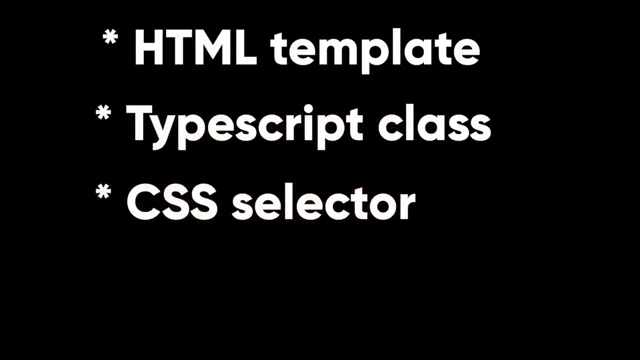 application. Each component consists of an HTML template that declares what renders on the page, a TypeScript class that defines behavior, a CSS selector that defines how the component is used in a template and, optionally, CSS styles applied to the component. A component must belong to an NG module in order for it to be available to another component. 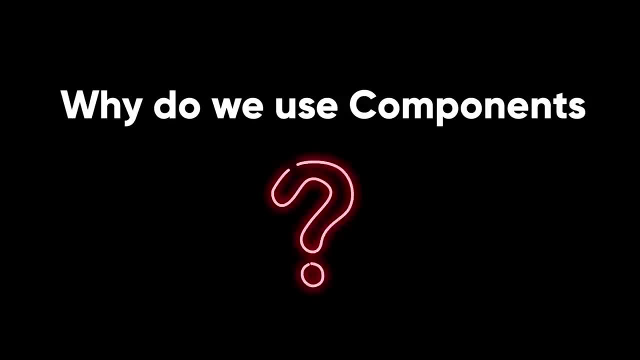 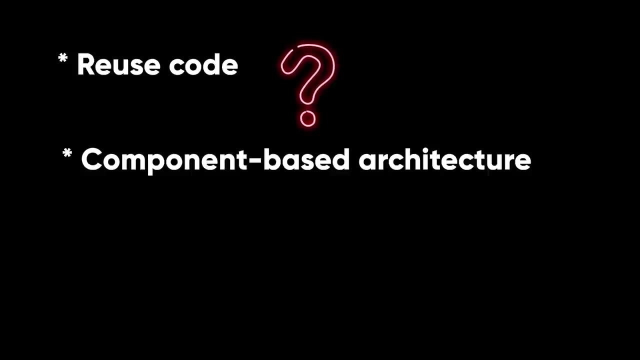 Why do we use components? There are many reasons, but the main ones are: we are able to reuse our code, so we don't duplicate it. Simplify component based architecture, easy to do, error handling and breaking down the complexity into smaller pieces. 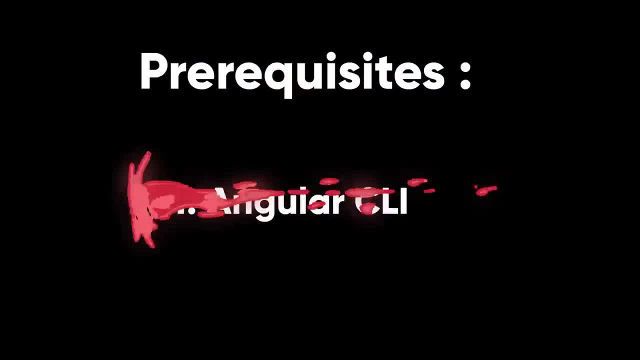 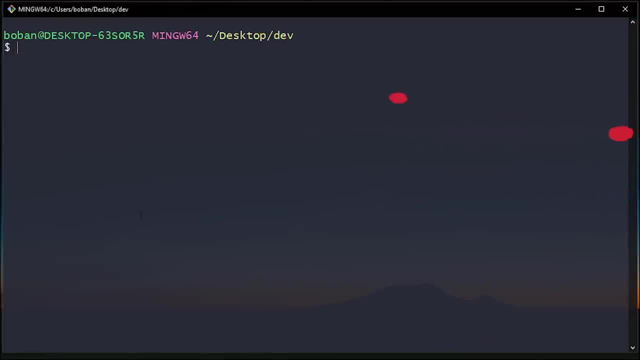 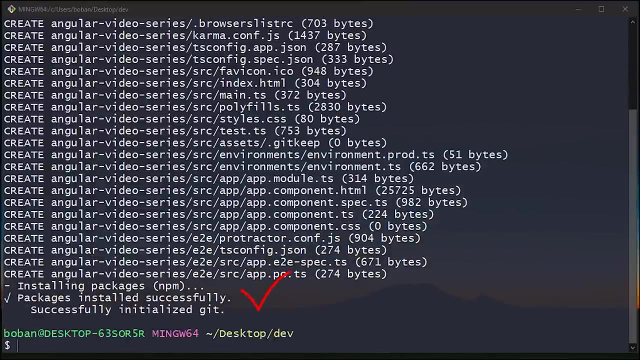 The prerequisites for these sections are: install the Angular CLI and create an Angular workspace with initial application. If you don't have a project, you can create one using NG new project name, where project name is the name of your application, Although the Angular CLI is the easiest way to create an Angular component In this tutorial. 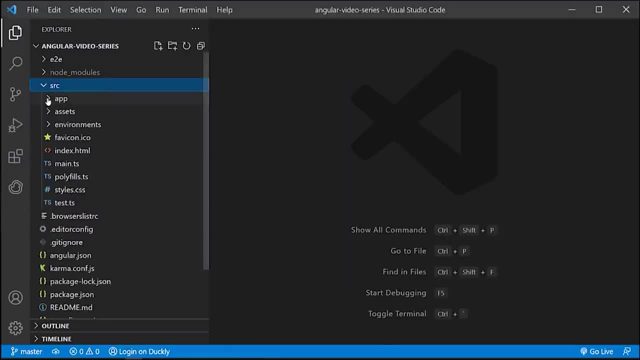 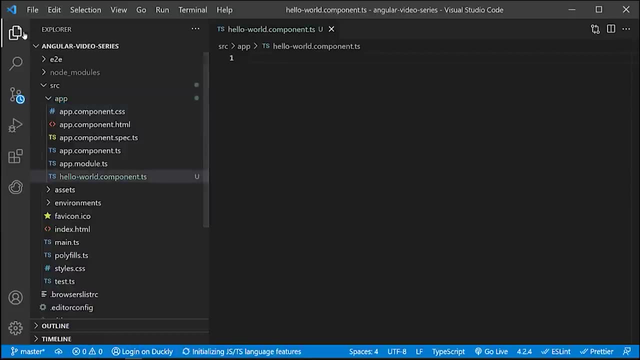 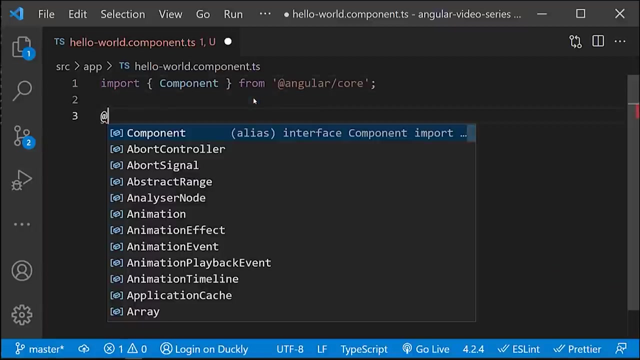 we will create our component manually. To create a new component, navigate your Angular project directory. Create a new file. hello world component TS file. At the top of the file add the following import statement: After the import statement, add a component: decorator. Decorator marks a class as an. 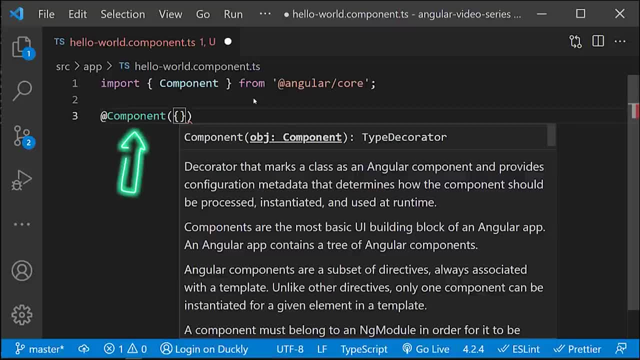 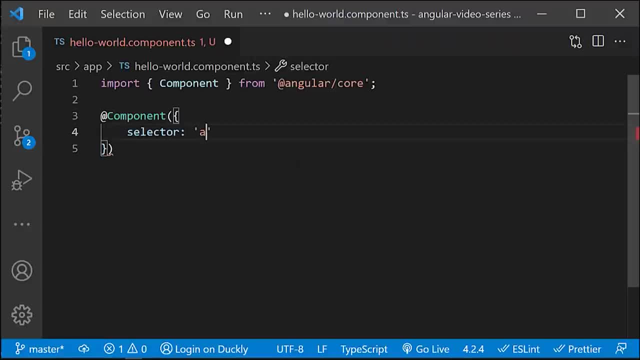 Angular component and provides metadata that decides how the component is used at runtime. Choose CSS selector for the component. This is a tag which you will be using in your template files to render your component. Define the HTML template that the component uses to display information. In most cases, this template is a separate HTML file, but I'll use it within this. 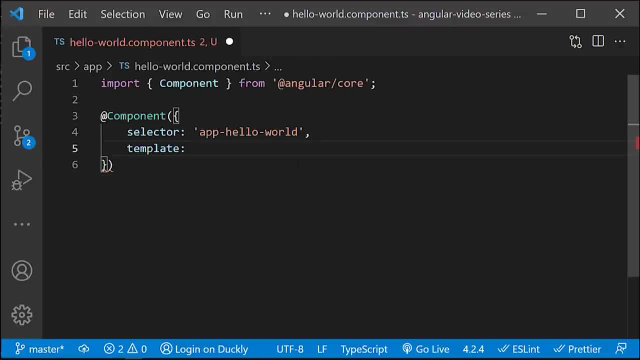 file. To define a template as an external file. add a template URL property to the component decorator for a template within the same file. Use template property. Select the styles for the components template. In most cases, you define the styles for the component decorator Under. 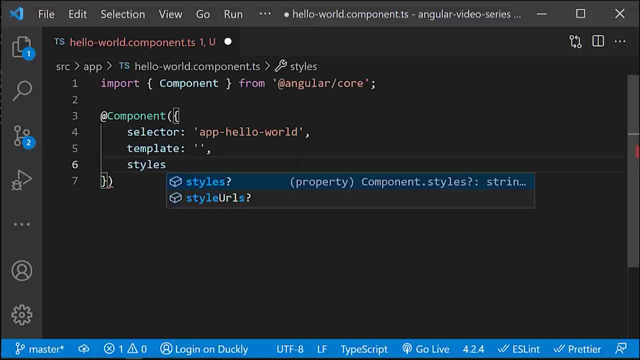 for your components template in a separate file. Again, I will use it within the file To declare the styles for a component in a separate file, add a style URLs property to the add component decorator. But for the styles within the component, add styles property. add a class statement that. 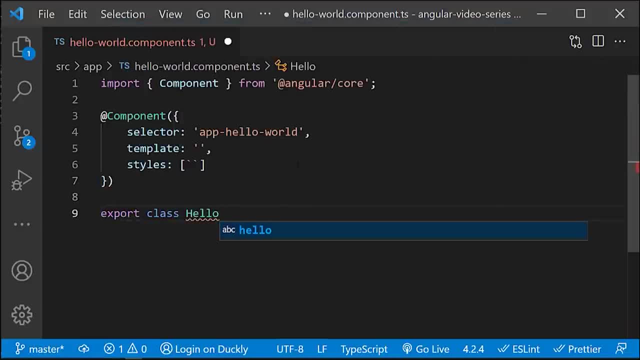 includes the code for the component. Here we can define properties, methods, catch component lifecycle events and do dependency ejection. But I'll talk more about these in the next video. Now all the public properties that you define in the class are accessible in the HTML template. 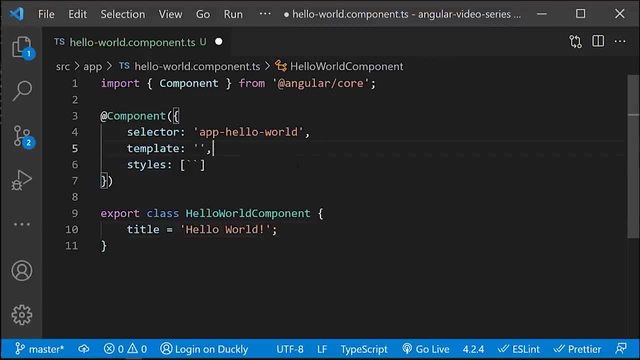 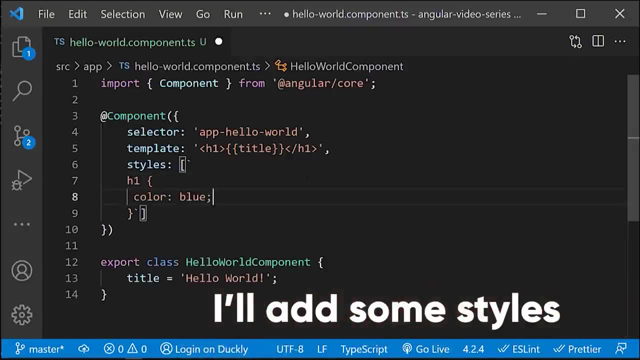 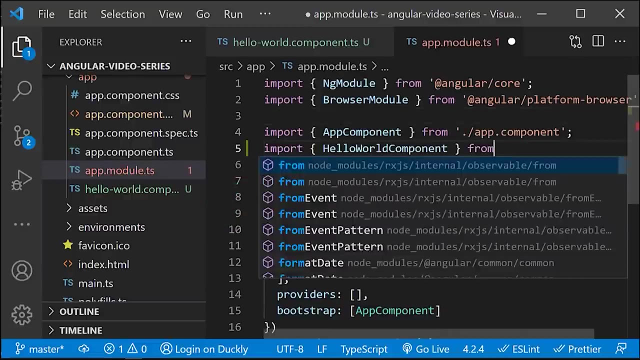 And this is one of the most powerful things here- I'll create a Tyler property and I will include it in the HTML Import, that new file, in the module where you want to use it, to make it available for the whole app in the next video. 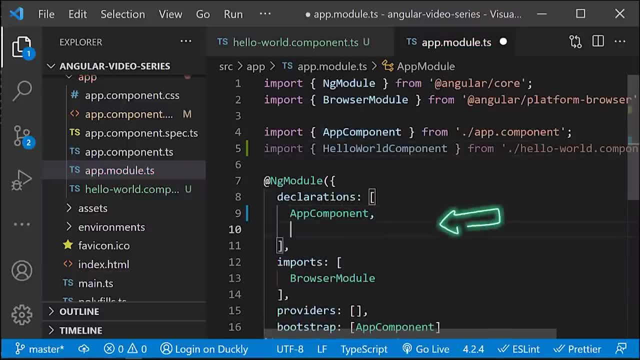 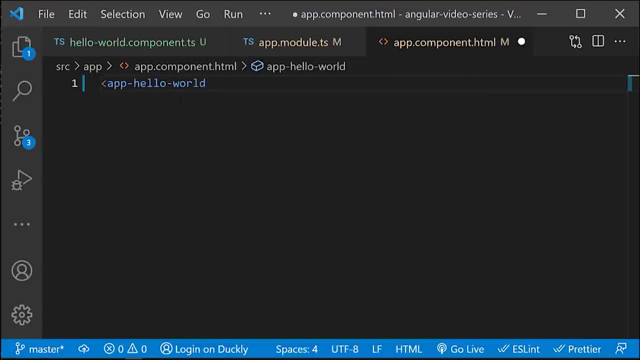 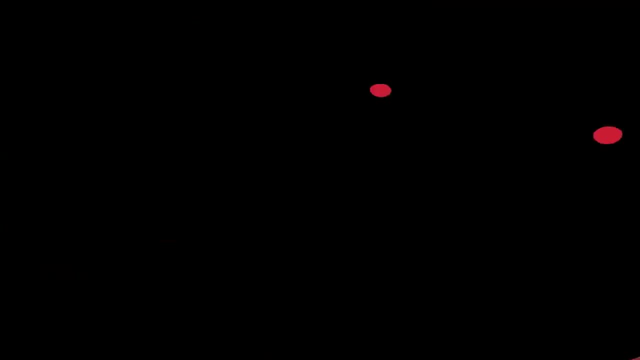 Import it in the root module In order to see our component. we can use our CSS selector inside of our app component or any other component, And this is your first component. very simple though, you can reuse across your app In this section. 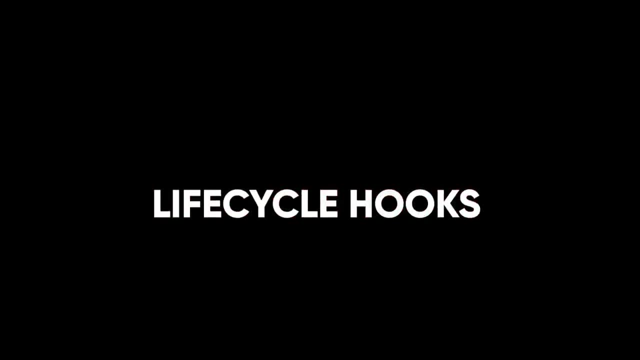 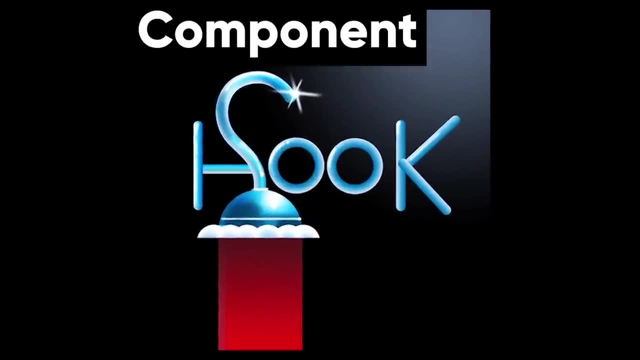 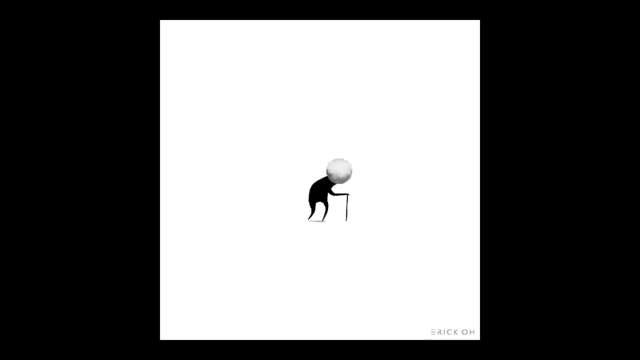 we are talking about lifecycle hooks. There are special functionality in Angular that allows us to hook into and run code at a specific lifecycle event of a component or directive. You can look at them as phases of component life, like every living being has. they get born, they change. 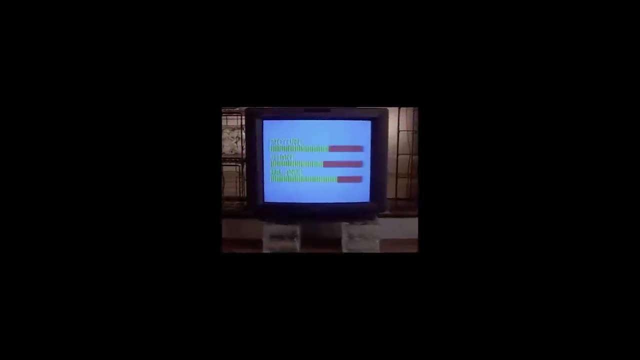 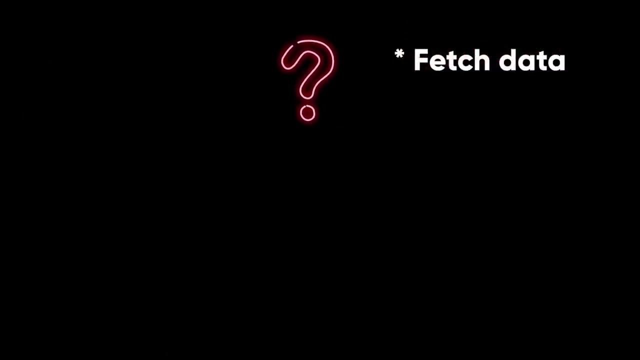 they grow and eventually they die. With lifecycle hooks you can gain better control of our application. When do we want to use them? For example, if you want to fetch some data and display it in your component, you will do that inside of ngOnInit lifecycle when it component. 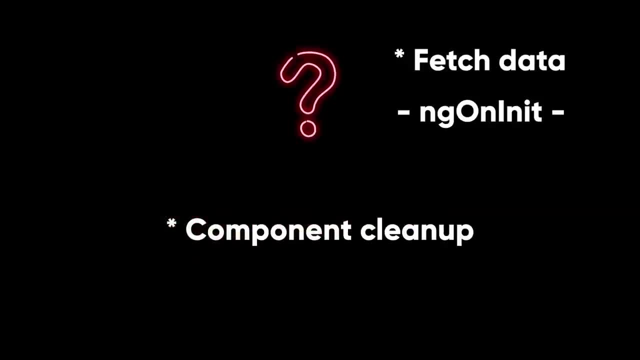 gets initialized, Or if you need to clean up your component, remove some subscriptions you might have to prevent memory leaks. You can do that inside of your component. You can do that inside of your component. You will do that inside of ngOnDestroy lifecycle hook just before component gets. 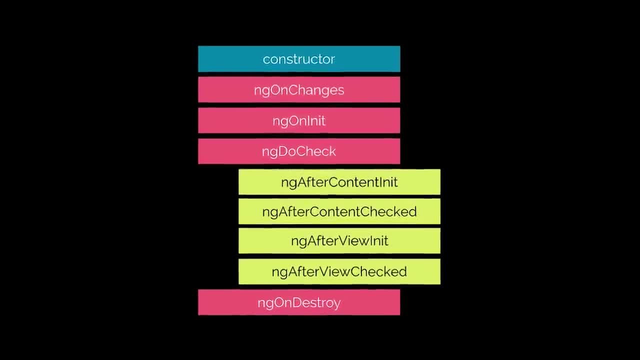 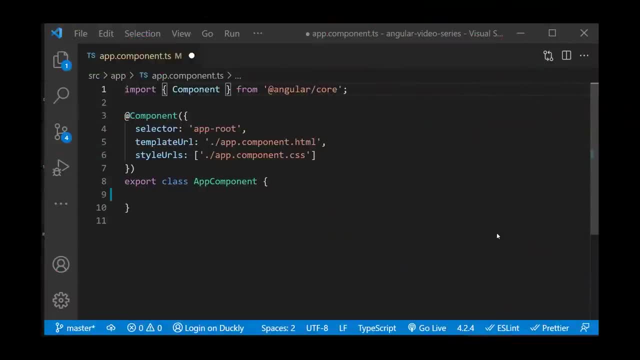 destroyed. This is the list of all hooks in exact order how they get initialized, But most used ones are onInit, onChanges and onDestroy. Let's implement the ngOnInit hook, as you will be using this hook the most First: import onInit interface from Angular core. 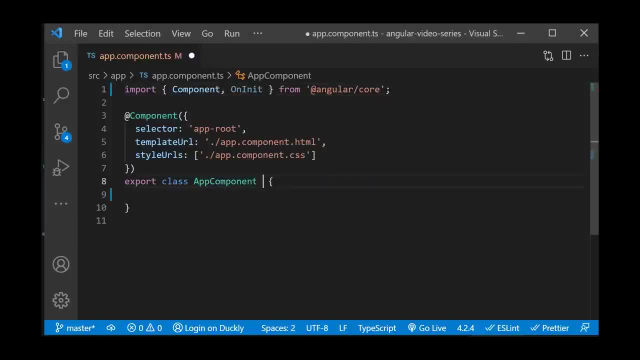 Next, we want to implement this interface inside of our class. To implement any hook, you just need to add an ng to the interface name and you will get the method needed for implementation. So in this case it's ngOnInit. We will create a simple function for logging some. 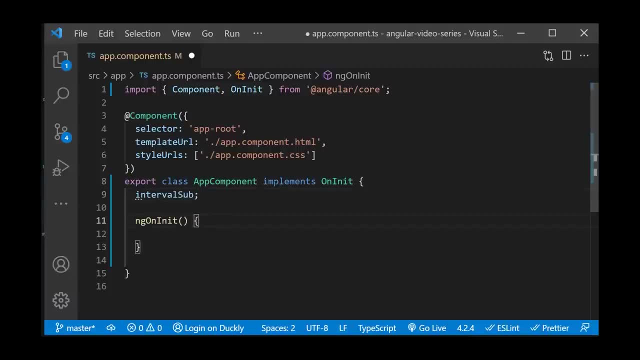 values to the console. Now I will create a property that will save that function so that we can clean it up at the end. In the ngOnInit method, let's create a simple set interval method which will make a console log on every second. 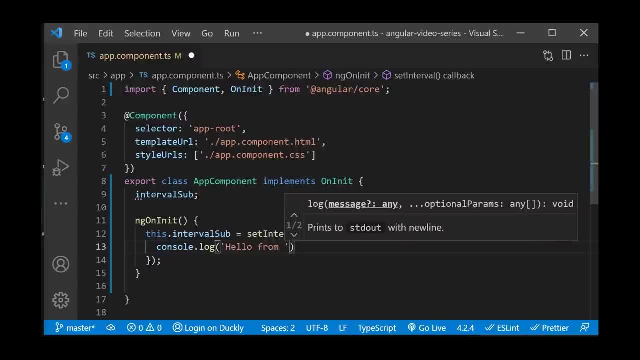 If you leave our component like this, when the component gets destroyed, our interval method will continue to log to console. To fix this side effect we need to use the ngOnDestroy hook, Import onDestroy interface and placed it next to onInit. Now create the ngOnDestroy method And in this method you need to clean up this interval. 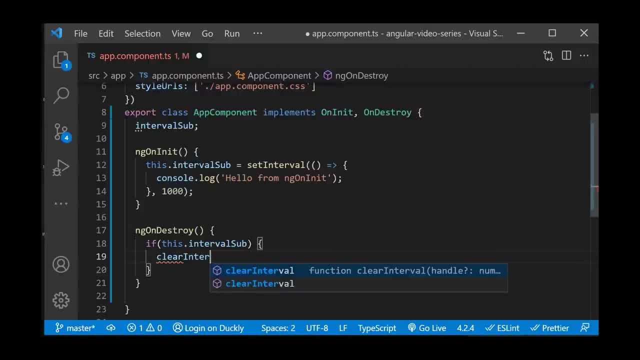 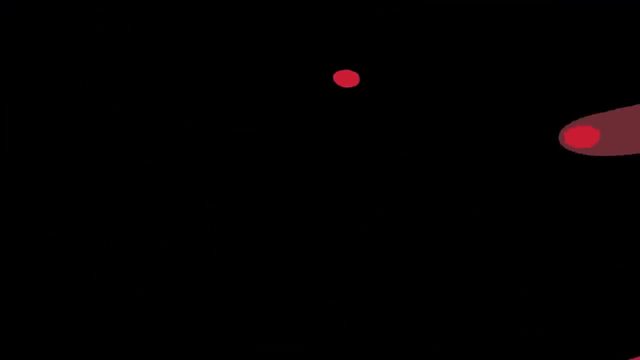 Simply use a clear interval method with our property passed as an argument, And now our component has been cleaned up. Using lifecycle hooks, we can fine tune the behavior of our components during creation, update and destruction. Next, text interpolation. Text interpolation in Angular is a one way data binding technique that is used to transfer the. 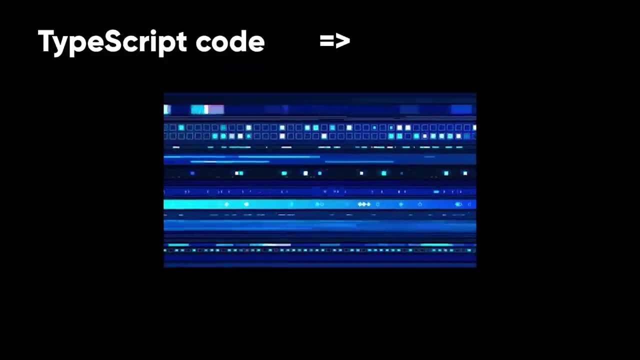 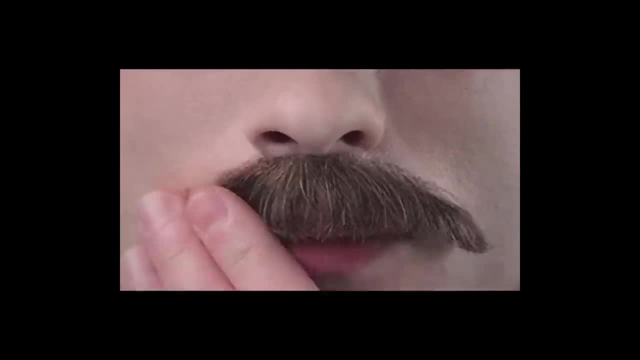 data from a test script code to an HTML template. It uses the template expression in double curly braces, also known as a mustache syntax. To do this, we need to use the ngOnInit method To display the data from the component to the view. When do we need text interpolation? Every. 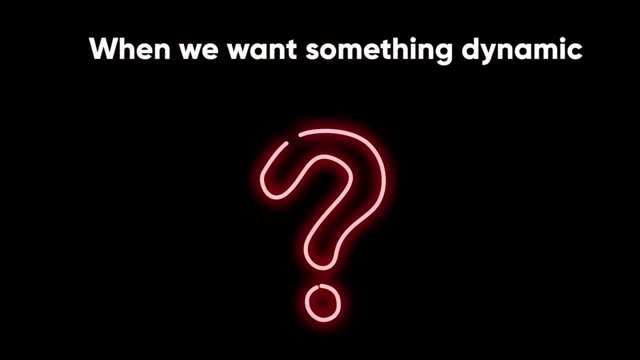 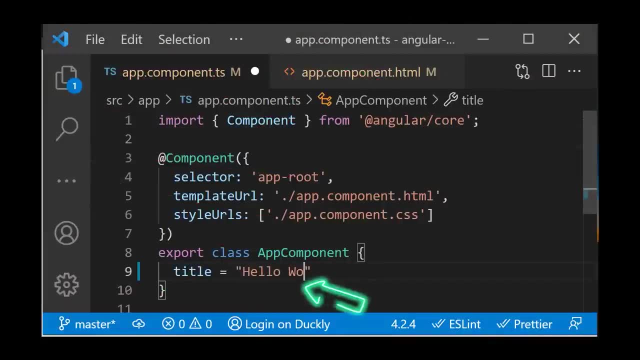 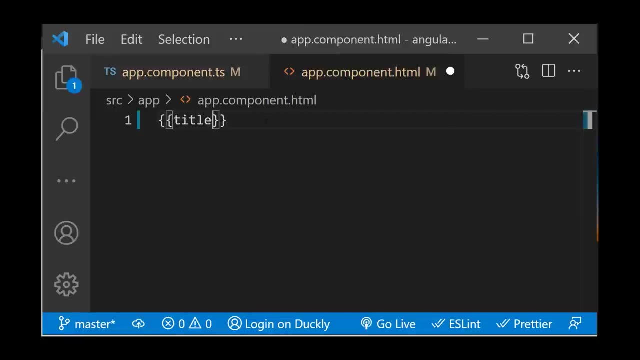 time we want to make something dynamic in our HTML template. To illustrate how interpolation works. let's create a new variable in our TS class. You can use interpolation to display the value of this variable in the corresponding component template. Angular replaces title with the string value of the corresponding component property. In this case, the value is hello world. 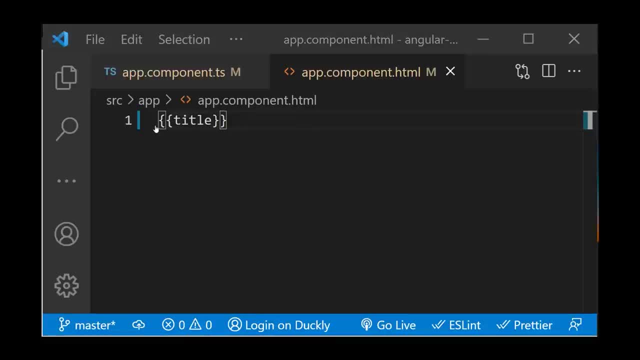 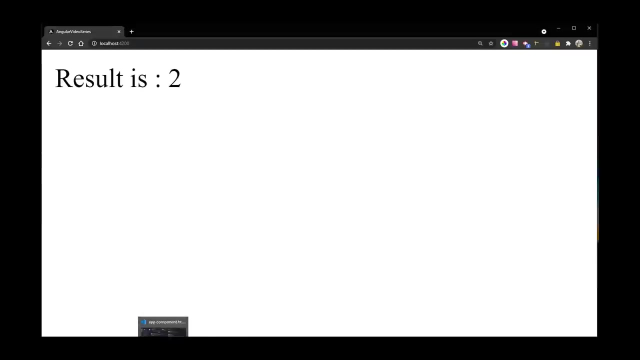 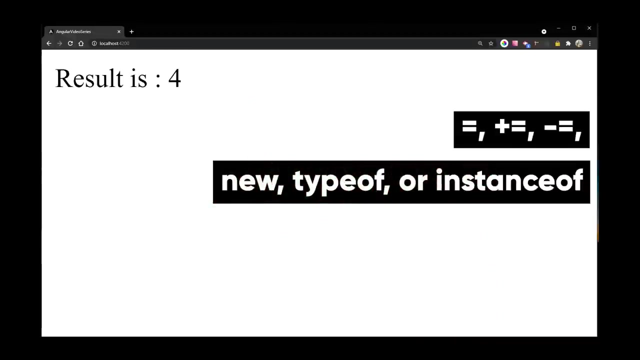 Now let's talk about template expressions. A template expression produces a value. in appears within double curly braces. Let me show you an example. Angular resolves the expression and assigns it to a property with a binding target. Template expressions are similar to JavaScript, except you can't use assignments. Also, operators such as new type of or instance. if you can't. 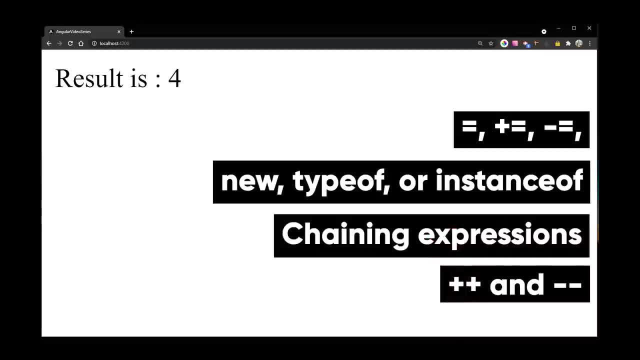 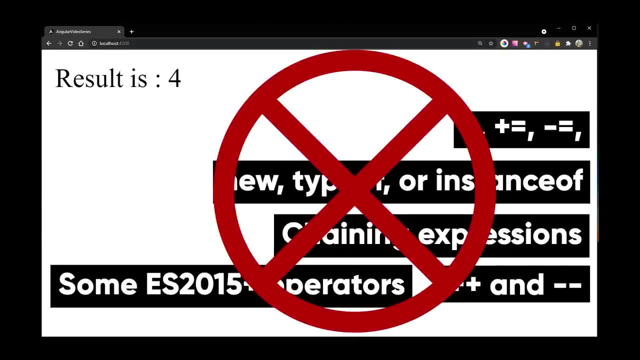 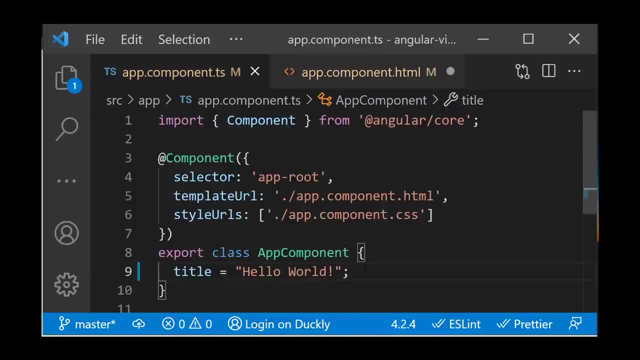 use chaining expressions, decrement or increment over the same surface value. Then you need property increment operators and some of the ES 2015 plus operators expressions can also invoke methods. So let's create one name of our method will be get mean And in this method we are returning. 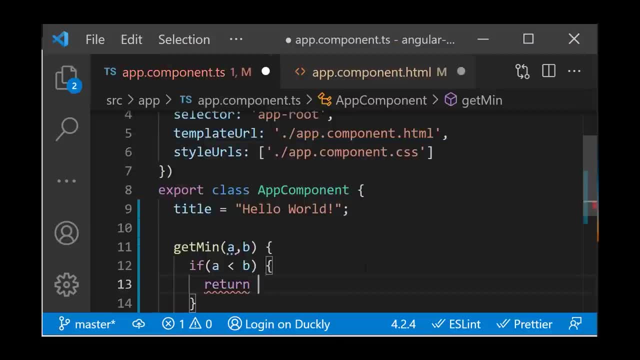 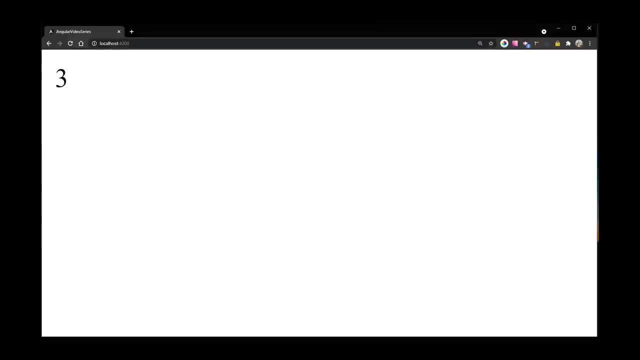 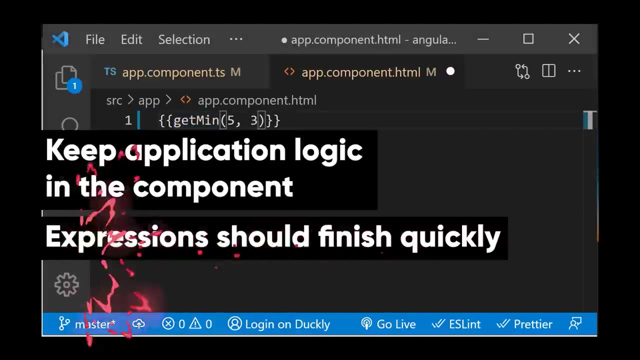 value for displaying it in our template. In this case it will be a minimum value. A couple of things I want to mention. you should keep application logic in the component as much as possible, where it is easier to develop and test. Also, expressions should finish quickly to keep. 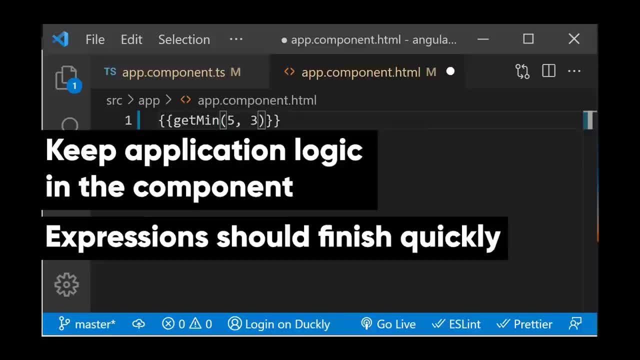 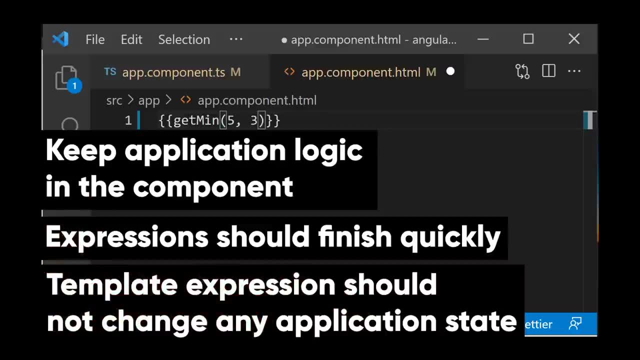 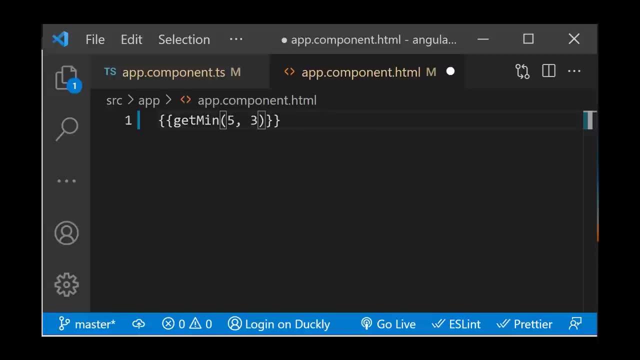 the user experience as efficient as possible, especially on slower devices, And template expression should not change any application state other than the value of the target property. Reading a component value should not change some other displayed values. Now let's learn how to communicate between the components. 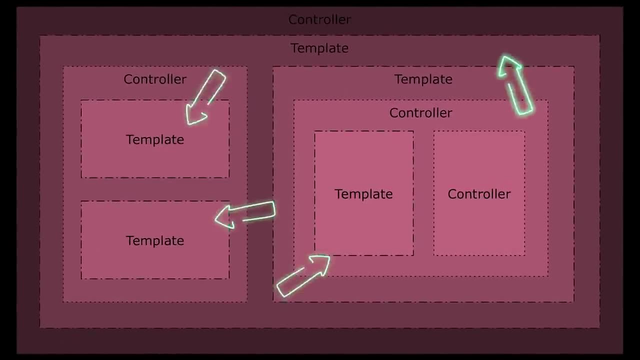 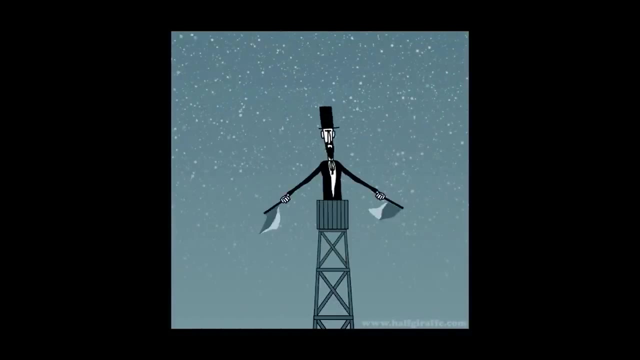 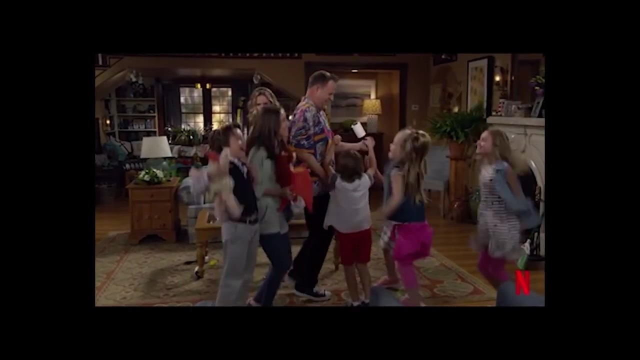 An Angular application usually consists of many separated components, And in order to make them work together, we need communication between them. You can think of components as family members, And if communication between the parents and kids is fluent and efficient, your home will be a happy. 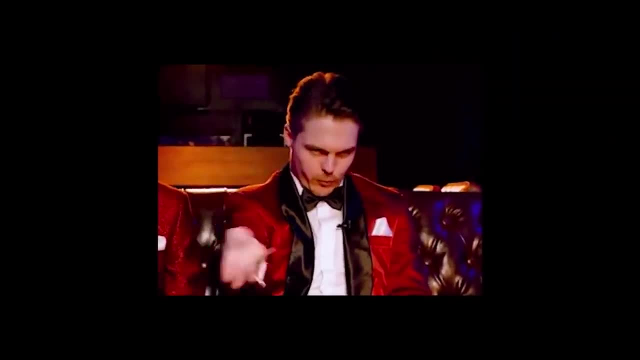 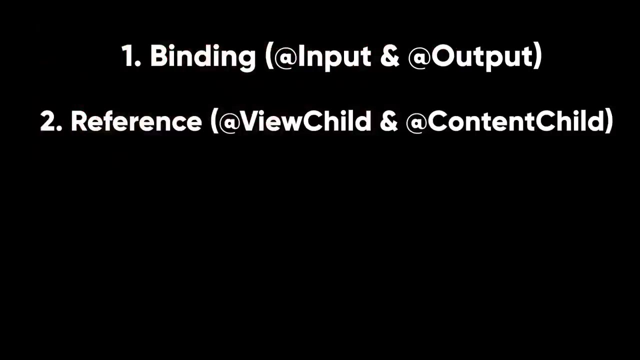 place. There are four ways to communicate between the Angular components: binding using input and output reference by using view chart. In this tutorial I'm going to cover the first two ways, as we haven't covered services yet and a template output is a little bit advanced. First use case is when we want to send data from 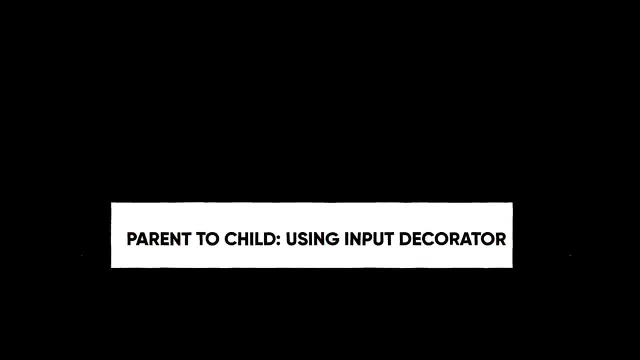 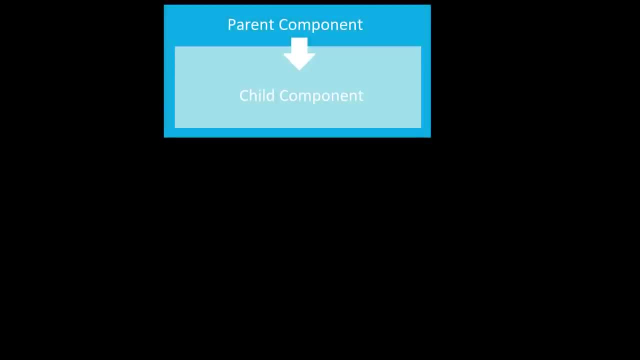 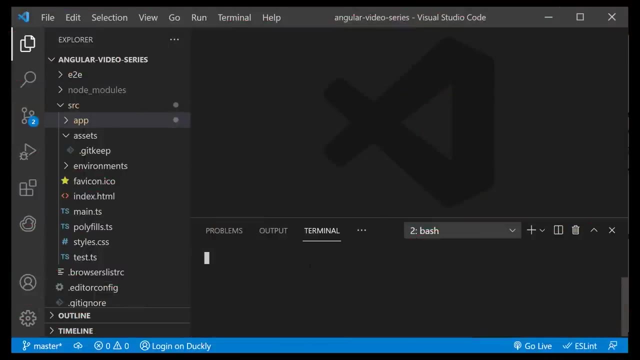 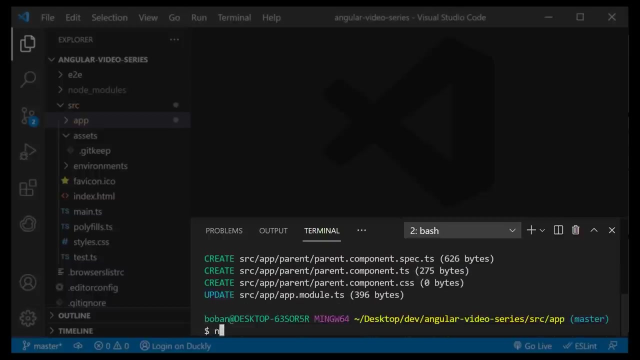 parent to child using input decorator. Input decorator takes the value passed from parent and stores that value in the child property. Let me create two components using Angular CLI. Input decorator takes the value passed from parent and stores that value in the child property. I will run the following commands: ng generate component. parent and ng generate component. 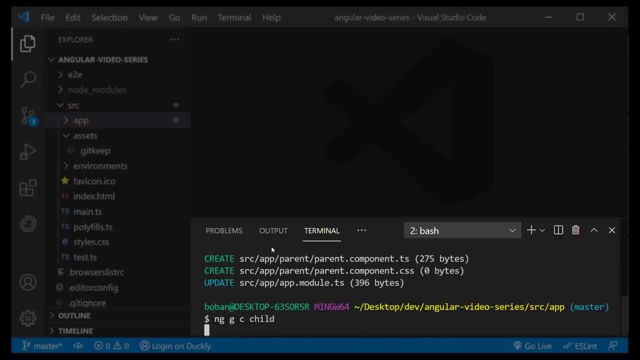 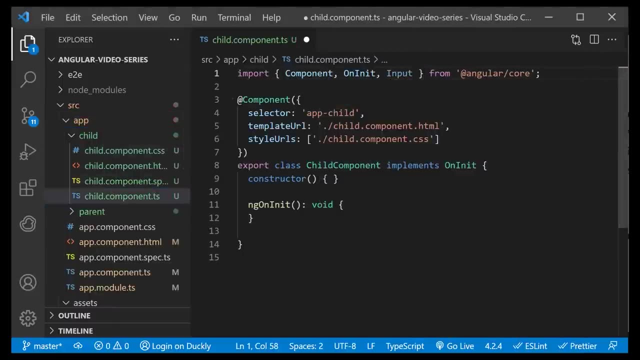 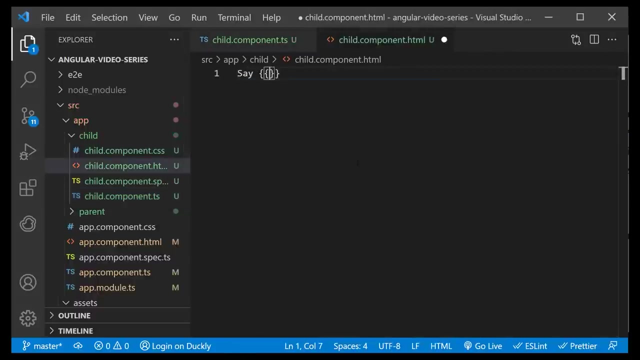 child. In our child component I will import input decorator in name our input as child message of type string. In the template of the same component I will display this property which is going to be passed from a parent Now inside of our parent component. in the template we want to place our child component. 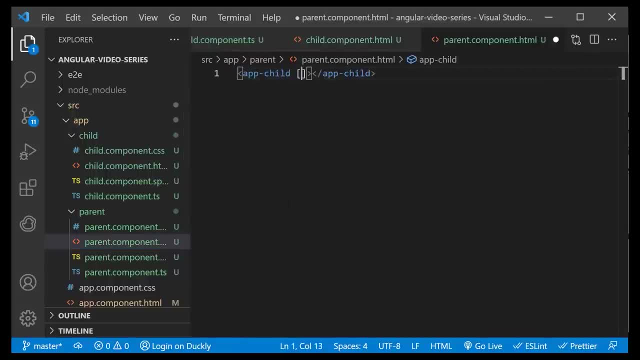 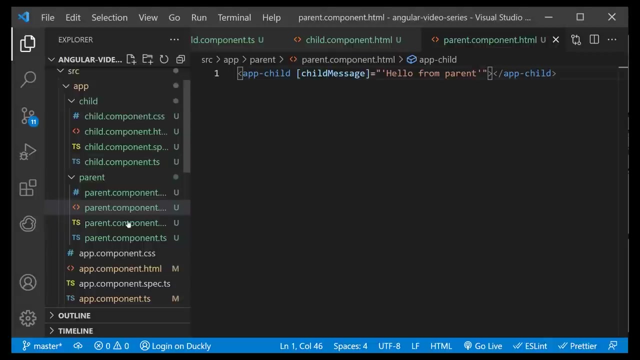 and to pass the value to the input property we just created. The name of the property is the one we defined in the child component and the value is going to be a hello message. Next, we want to place our parent component inside of our root component. 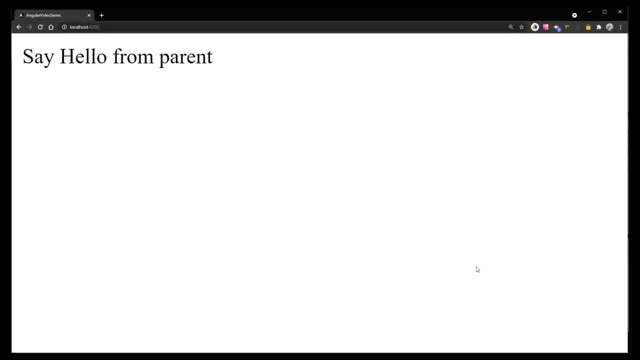 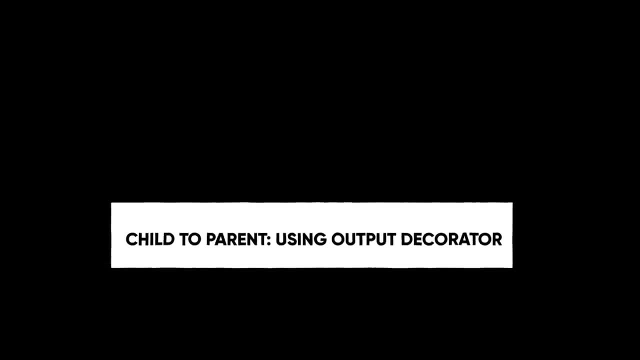 And if we preview it, we can see their message from parent has been displayed in our child component. Second use case is when we want to send data from child to parent using output decorator. Output decorator marks a property in a child component as a doorway through. 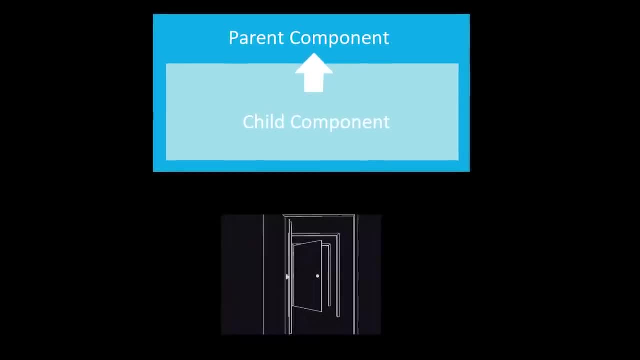 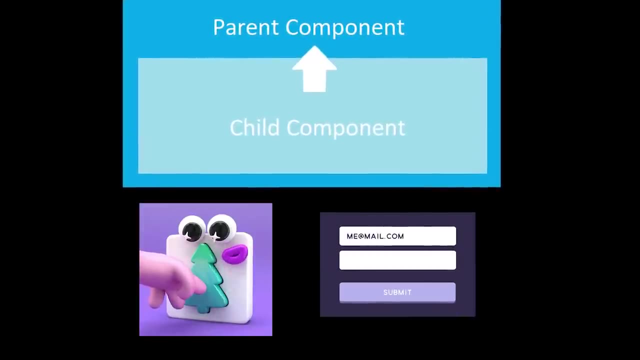 which data can travel from the child to the parent. This approach is a little bit more complicated than the previous one. The message is ideal when you want to share data that occurs on things like button click, form entries and other user events. To raise an event and output must have the type of event. 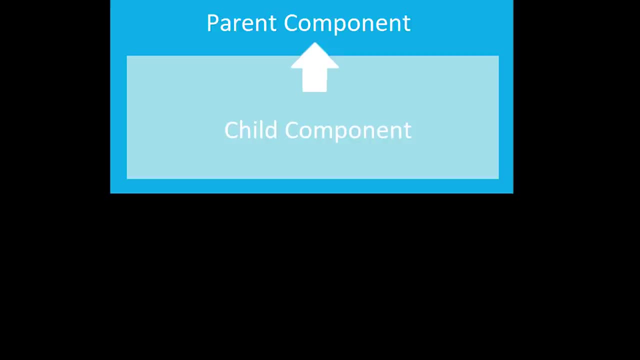 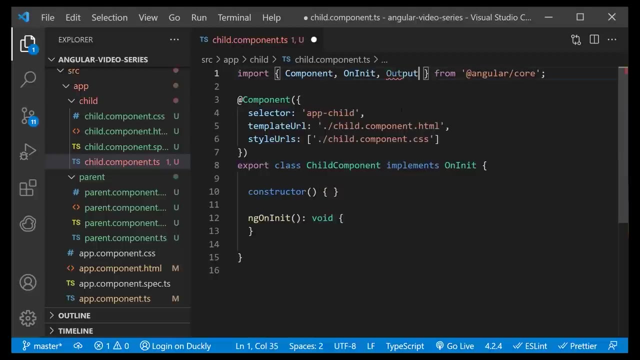 emitter, which is a class in the Angular core that used to emit custom events In the child component import, output decorator and event emitter. We declare a message event variable with output decorator and set it to equal To a new event emitter. Then we create a function named send message. 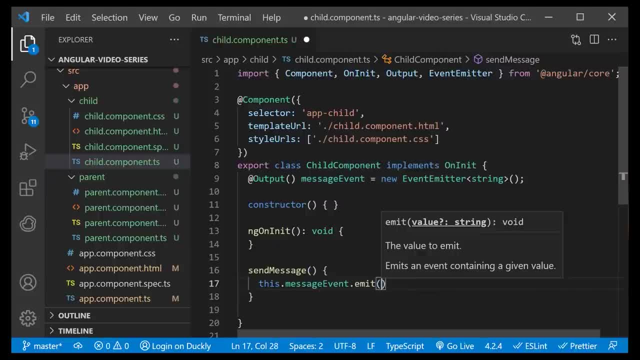 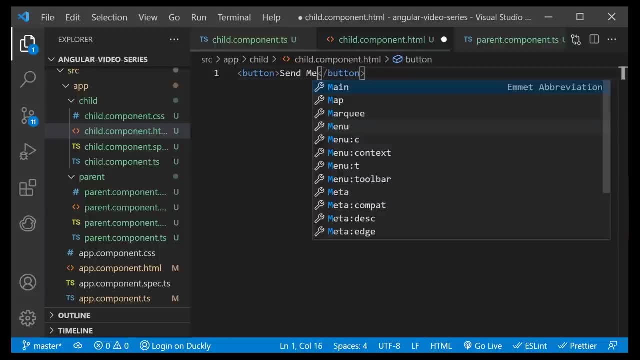 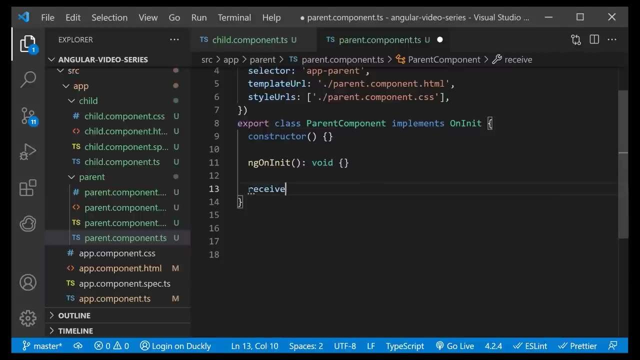 that calls emit on this event with the message we want to send. Lastly, we create a button to trigger this function In the parent. I will create a function to receive the message that will just simply alert this message for demonstration purposes Now in the parent template. call our function once the event from the child component occurs. 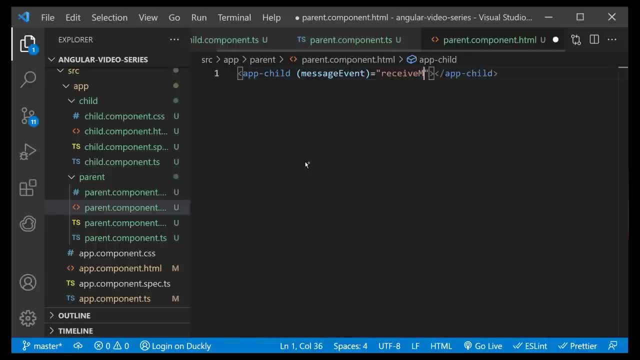 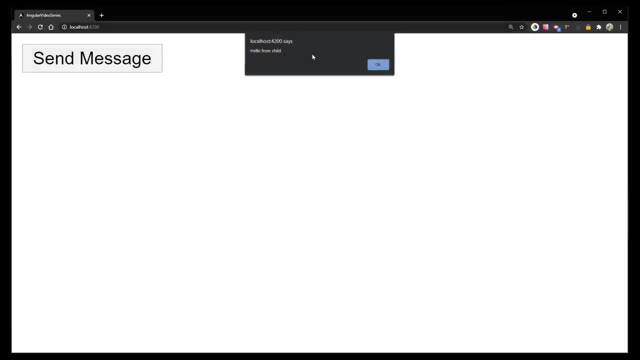 And the name of that event is the one that we defined with output decorator. Very simple and effective. Compared with all other approaches for communication, binding is the cleanest and the simplest one. It is the most maintainable way for passing data, Hence binding is always the most preferable way that Angular developers should consider first. 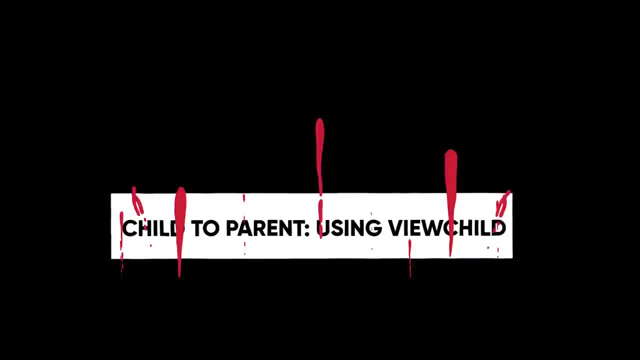 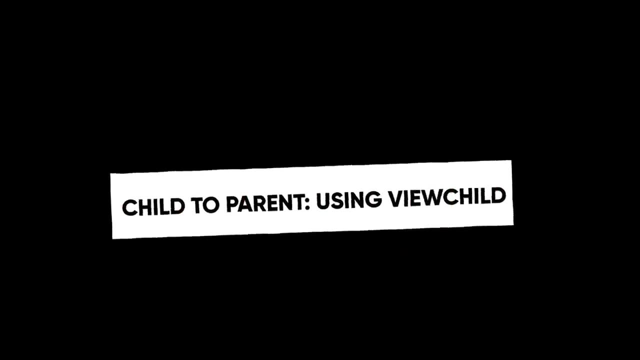 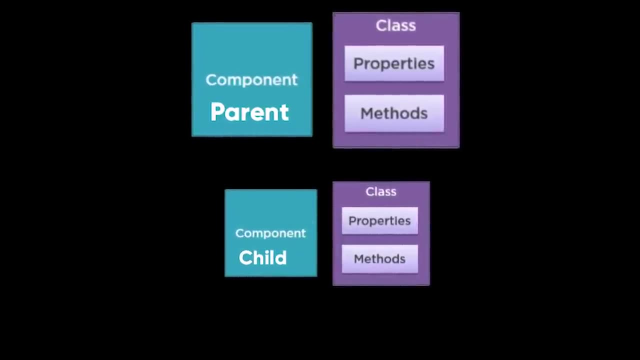 Third use case is when we want to send data from child to parent using view child. View child allows a child component to be injected into a parent component. It will give the parent access to its properties and functions. A child won't be available to give access until the view has been initialized. This means we need 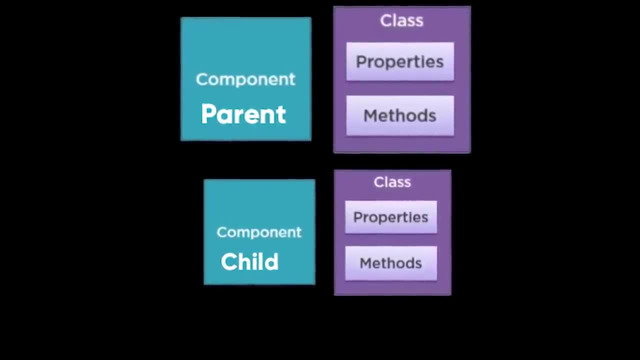 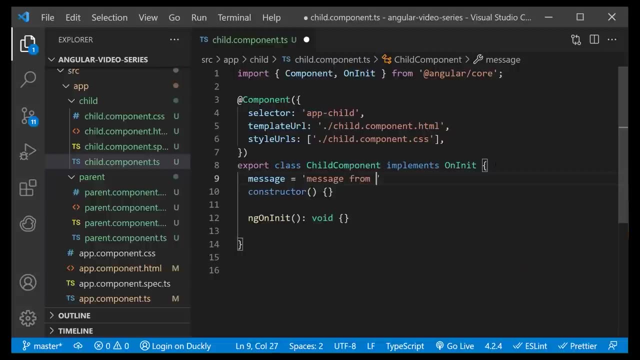 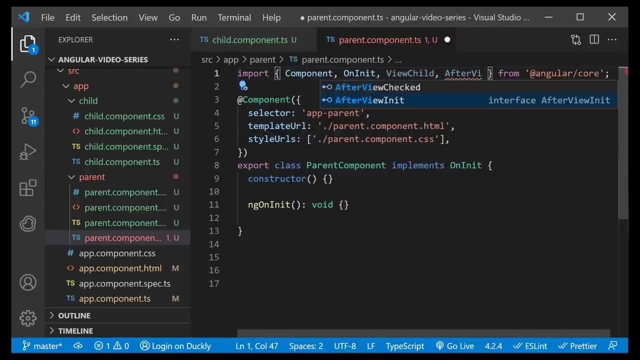 to implement the after view in the parent component And then we can send the data to the child component To implement the after view in it. lifecycle hook to receive the data from the child First, create a message property in our child component. Import your child in after view in it from Angular core and our child component. 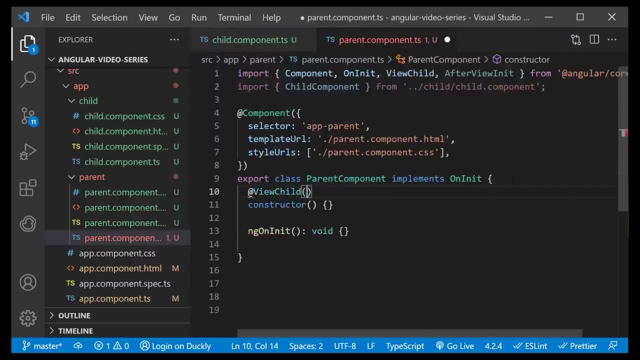 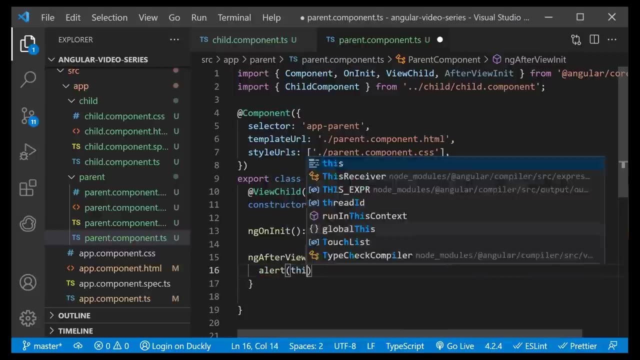 For our view, child decorator. pass our child component as an argument and name it as child And put the child component as nothing but a new name. Next, implement after view init lifecycle hook. By the way, to learn more about Angular hooks. 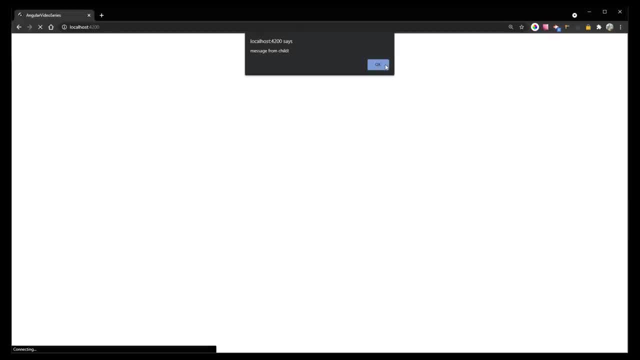 check the part two of this video series Inside the ng after view init method. just alert the message property of our child So that you can see that we have access to it And if we start our application, you can see that we are displaying a message from the child component. 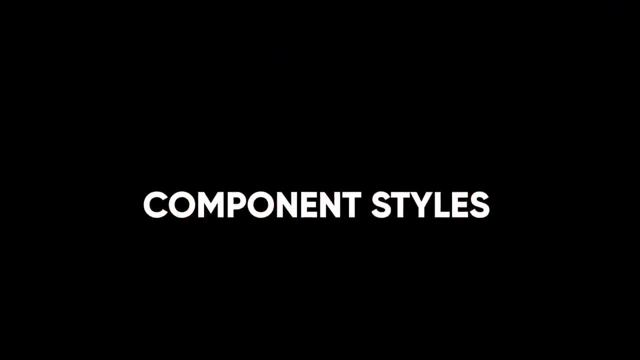 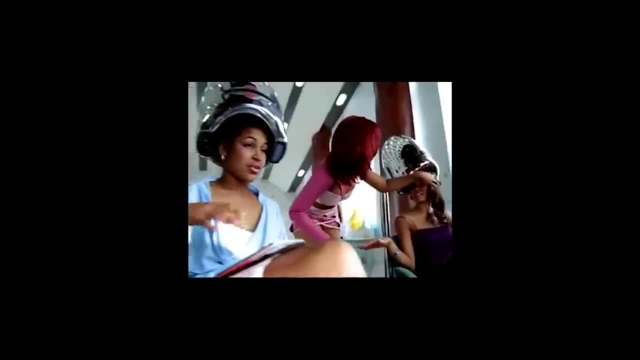 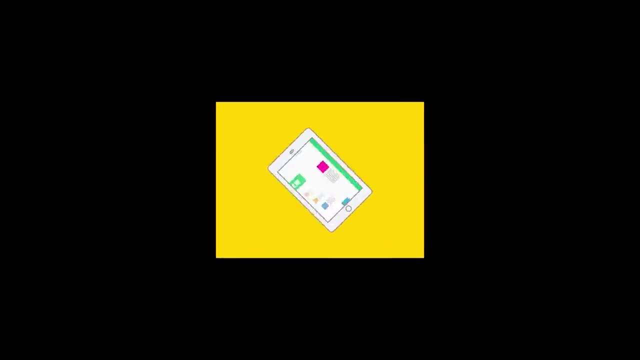 Next This: we are discussing component styles. Being able to style your app is very important because it allows you to make your app unique and attractive. in a way, it's like a beauty salon. World without CSS would be an ugly place. CSS gives us the opportunity to play with. 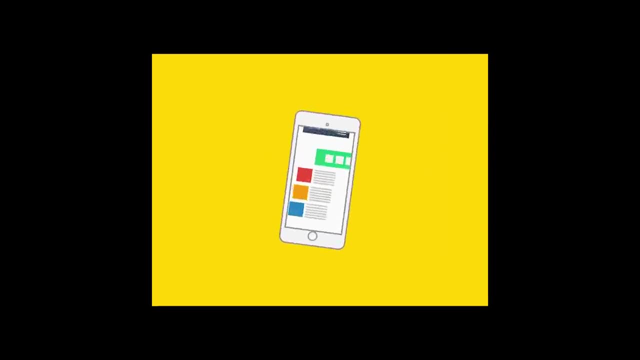 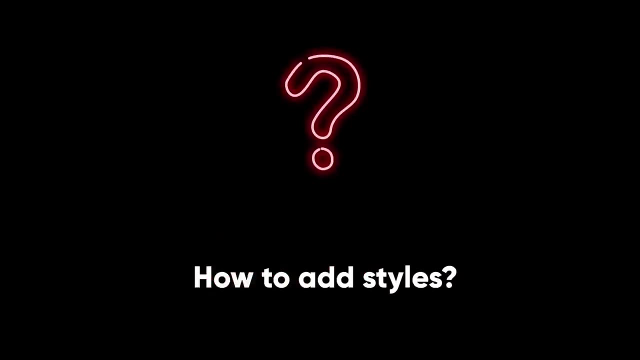 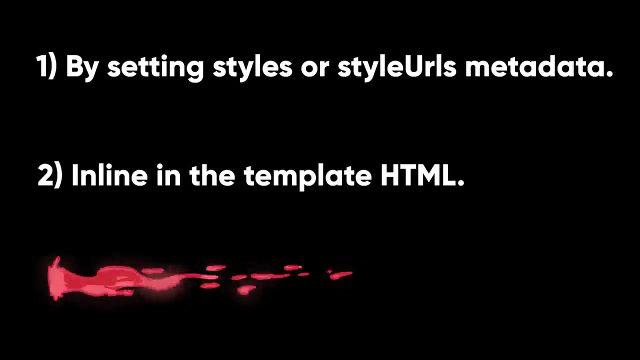 a page layout, adjust colors and fonts, add effects to images and so on. How to add styles to Angular components? There are three ways you can apply style: by setting style or style URLs, metadata in, like the template HTML, and three with CSS imports. 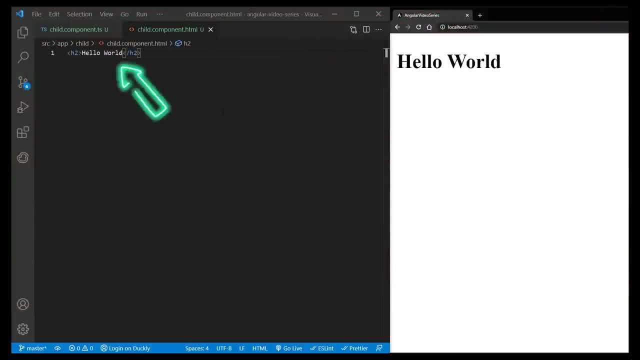 I created one blank component with only h2 tag in the view to demonstrate all different ways we can style it. You can add a styles array property to the component decorator. Each string in the array defines some C CSS for this component. You can load styles from external CSS files by adding a styles. 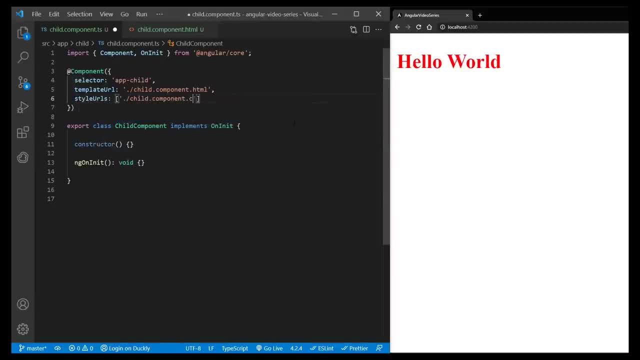 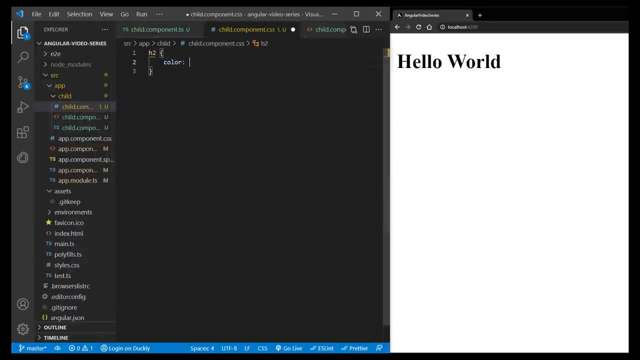 URL property to a components decorator, And now styles from external file are being applied. Next, you can embed CSS styles directly into the HTML template by putting them inside of style tags. A filehaul method is a very simple one: Just다고는, You can edit a URL you want from a package. Also, you can render a file when you create. 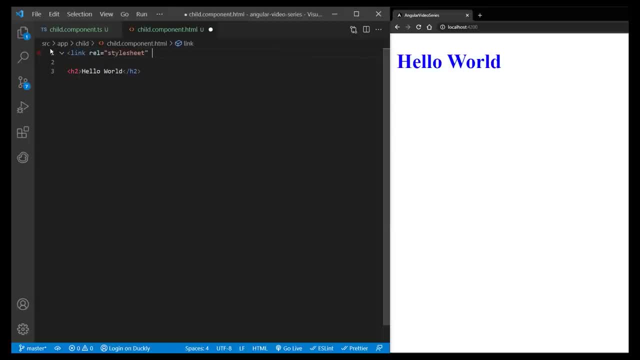 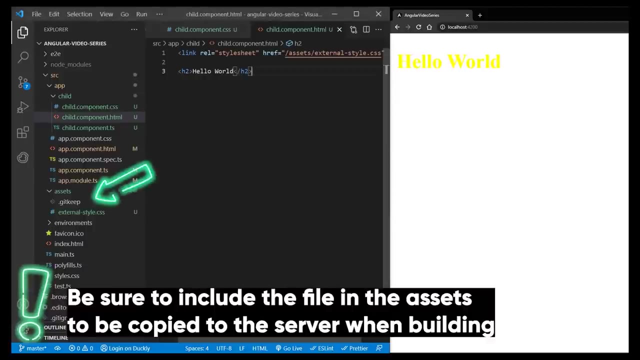 them. You can add any root steps and Wieder به Notes't. So what I said, wrote here, is to just be sure to include a link stiles file among the assets to be copied to the server when building. So when we post HTML elements to Engine dobr住. You can also import CSS files. Remember to leave us a comment. if you liked or if you really need more information about a face, please feel free to write me a comment and we will see you again in the next video. I see some in time щ. 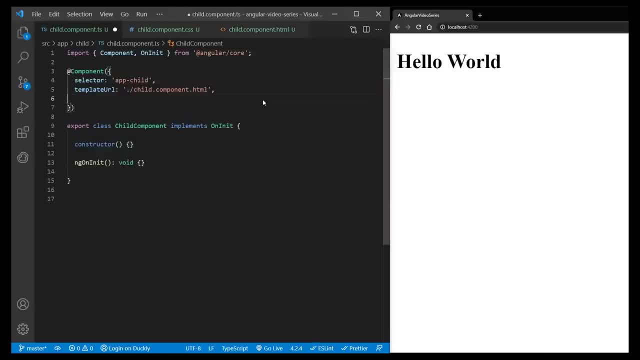 elle. One note here is to be sure to print and until you finish the lyrics or loss até the list�. Cocoon, I'm sleeping now. please do that with Java, So that we will end up with search cortex and into the CSS files using the standard CSS import rule. I usually use this approach to import. 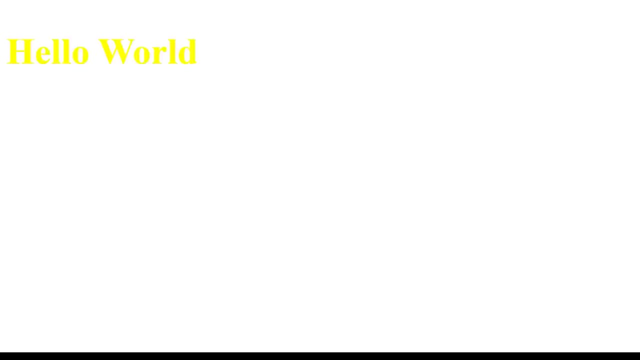 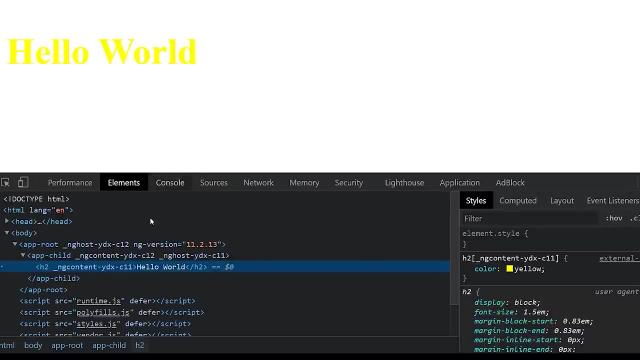 variables Reminder. these styles apply only to this component, So if you have h1 tag in a child or parent component, it won't be applied there By default. view encapsulation is set to emulated and emulates the behavior of the shadow DOM by pre processing and renaming CSS code to effectively. 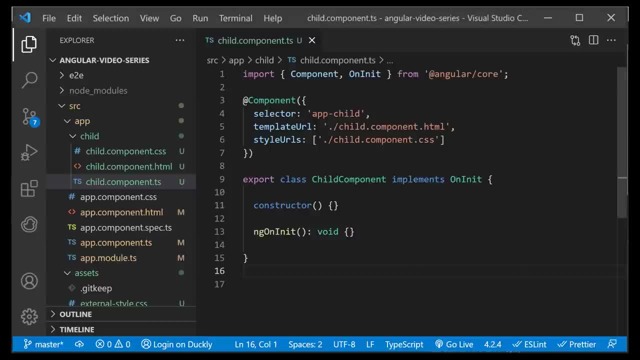 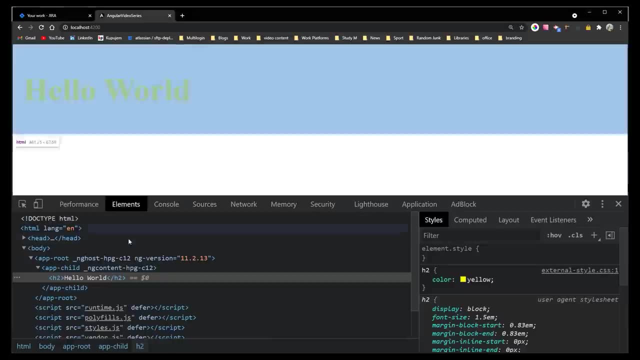 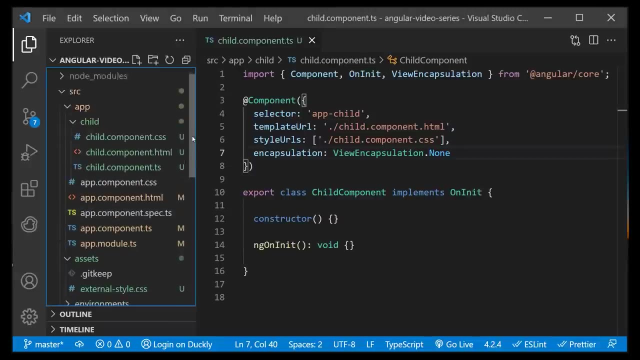 scope the CSS to the components view. We can remove these additional CSS selectors by setting encapsulation to none, And now our styles are being applied globally. Global styles are by default defined in the style CSS file And you can define more global styles in the Angular JSON file. 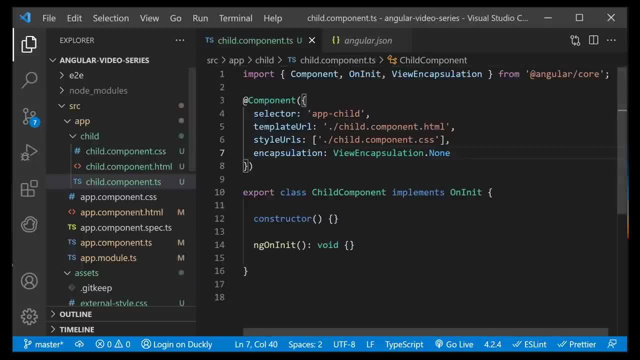 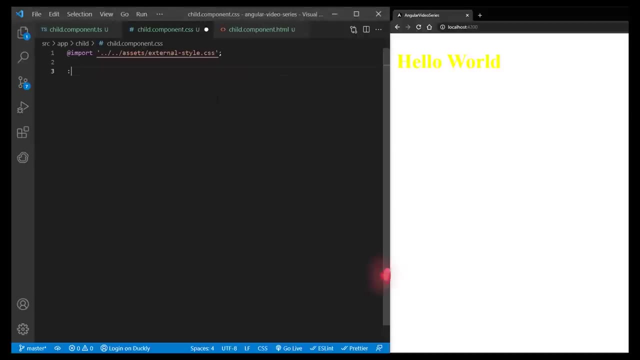 Another thing is that if you're building with the CLI, you can write style files in SAS less or stylus and specify those files in the component style URLs. metadata be the appropriate extension, as in the following example. Now let's talk about special selectors. Use the host pseudo class selector to target styles in the element that. 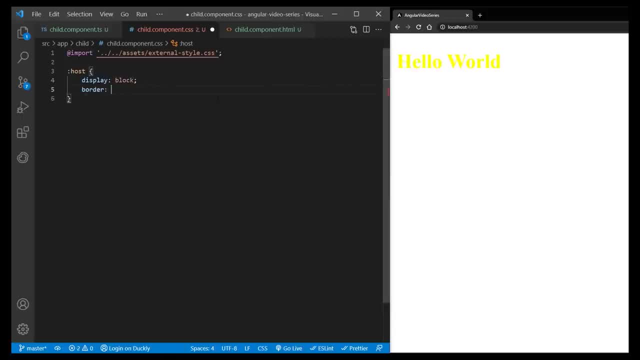 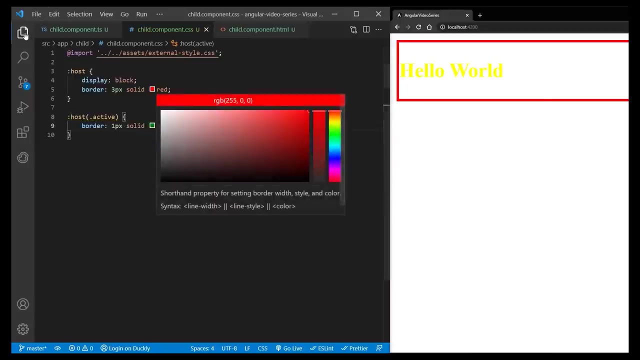 hosts the component as opposite to target elements inside the components template. For example, you can write the following code: We can style host styles with the given selector by using the function form as the following: And if you add active class to host component: 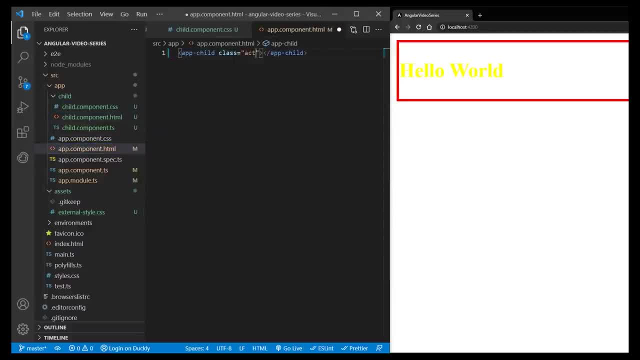 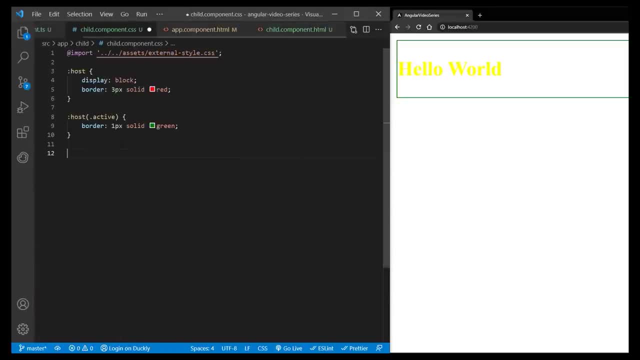 you can see that styles are being applied. Now let's talk about host context. Sometimes it's useful to apply styles based on some condition outside of the components view. For example, a CSS theme class could be applied to the document body element. 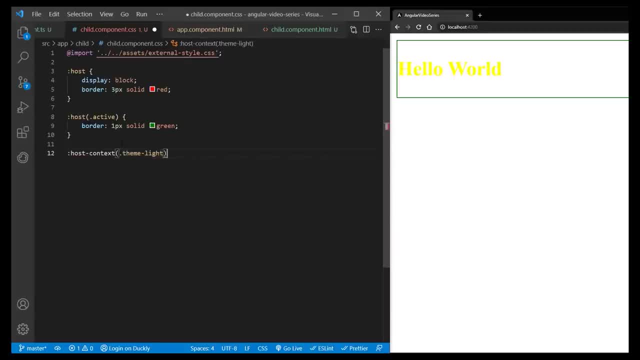 And you want to change how your component looks based on that. The following example: applies a background color style to all h2 elements inside of the component Only if ancestor elements has the CSS class theme light. Now, if you go to root element and add, 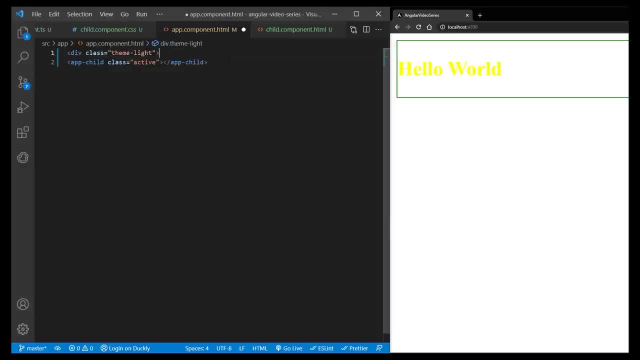 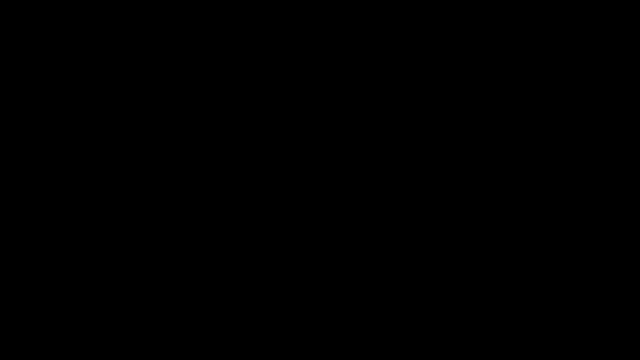 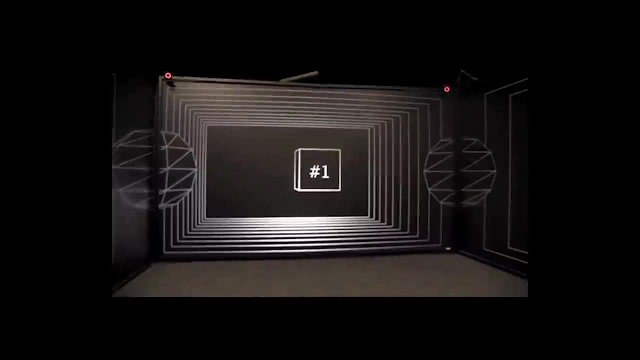 h2 element to these classes. you can see those styles and that's it. Now let's see what is ng content and you got and uses the content projection to take HTML telling the content to be not upturned to display inside itself. To me it's similar to film projector, where you have a slot to insert content which is going to be displayed as a respects' class element. 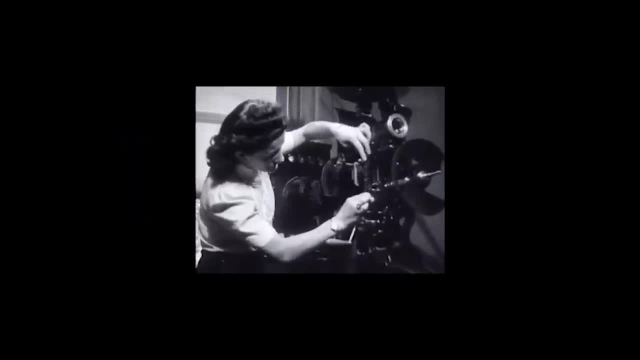 Now let's take a look at the Your поступivesangles. one basic 2005 mechanic from the database to this page says that it's more reasonable to have two a in the class, as you see them display an victory over one. It's quite easy to get better than them. 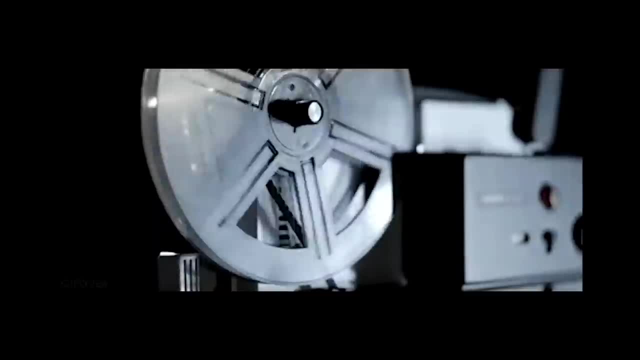 datapczenia. make it as a reference. The context bubble just e the semifinal picture related to. In the 다음 slide, let's scroll to the link from Microsoft ça be displayed on the screen. It's a very powerful tool when you're building components intended. 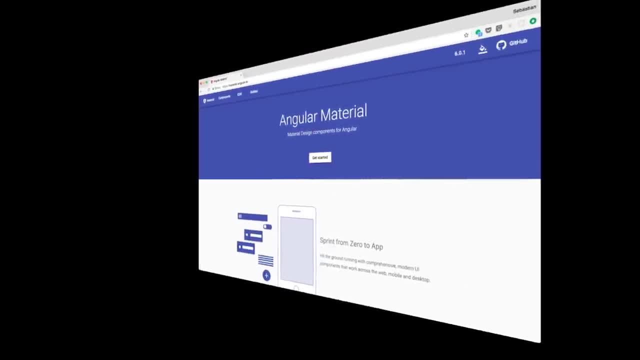 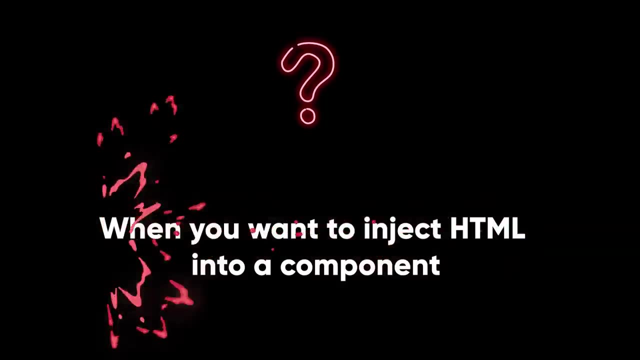 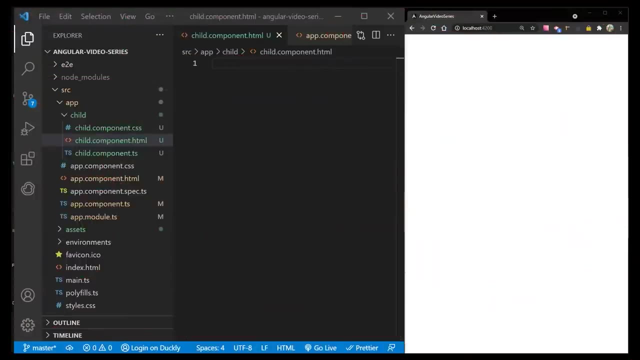 for reuse. I see it used extensively in frameworks such as ng material. When do you want to use ng content? Anytime you want to inject any kind of HTML into a component, you can do so with ng content. I have two components- child and root component- to demonstrate this feature Inside. 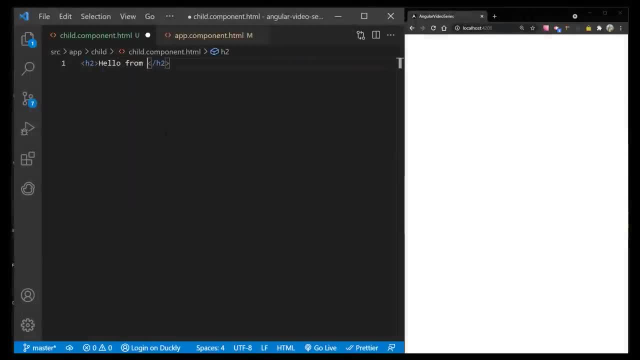 the child component. I will create some static content, So I'll add h2 title And below that title I want to show the dynamic content, So I will create an ng content tag. With the ng content element in place, users of this component can now project their own message into the component. 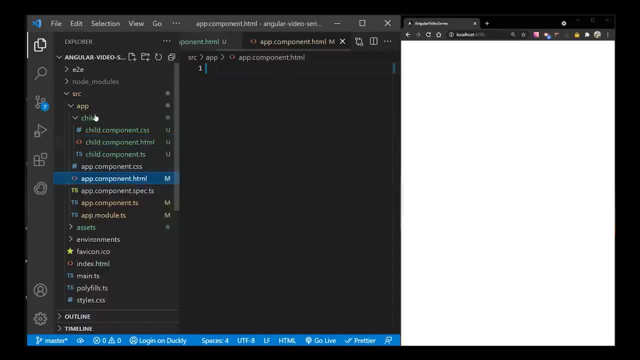 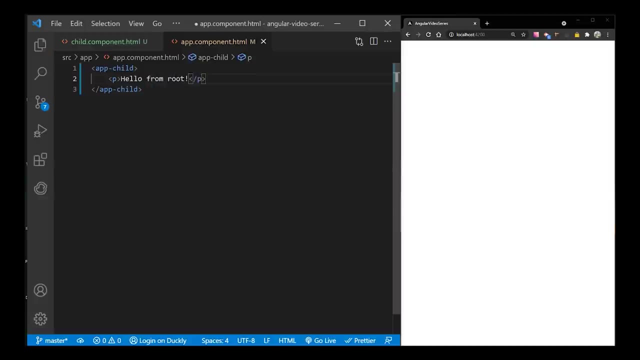 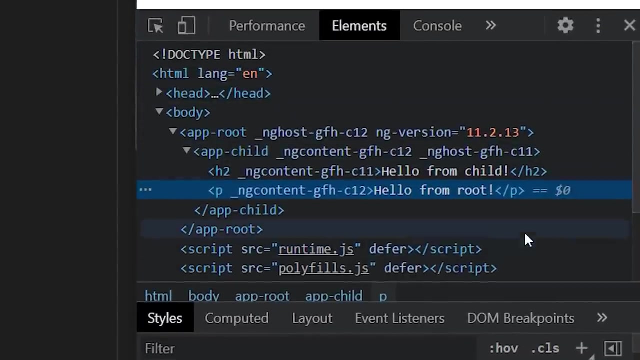 To do that, let me insert a child inside of our root component And I will pass a paragraph with a message. As you can see, the ng content element is a placeholder. that does not create a real DOM element. Now, except single, a component can have a multiple. 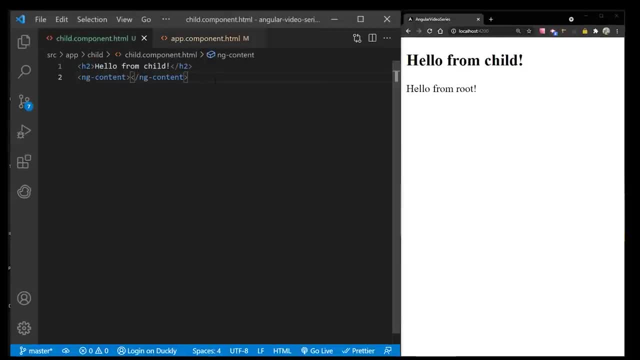 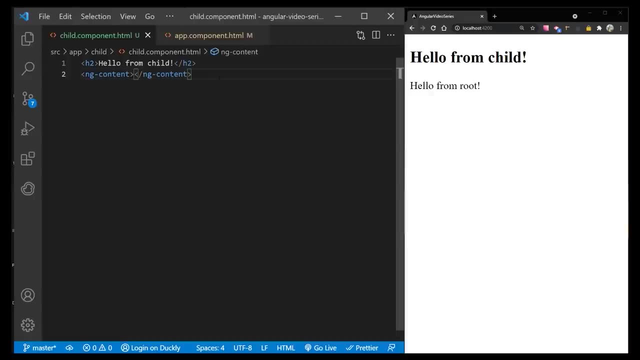 slots. Each slot can specify a CSS selector that determines which content goes into that slot. This pattern is referred to as multi slot content projection. You can accomplish this task by using the select attribute of ng content Inside of our child component. add one more ng content tag. 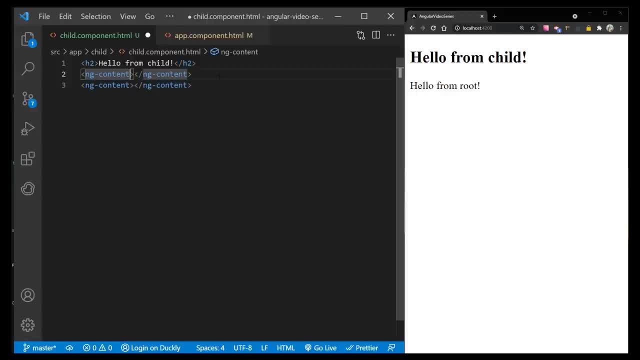 we can make our component to be like a question and answer card. So in the first ng content, add question selector And for the second ng content, add answer selector. Now we can use the select attribute to send different content. In our root component I will create h3 title. 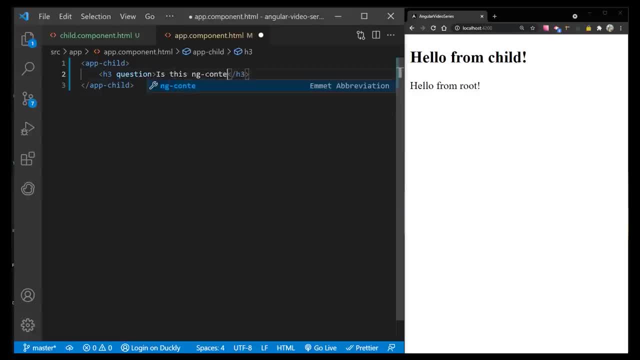 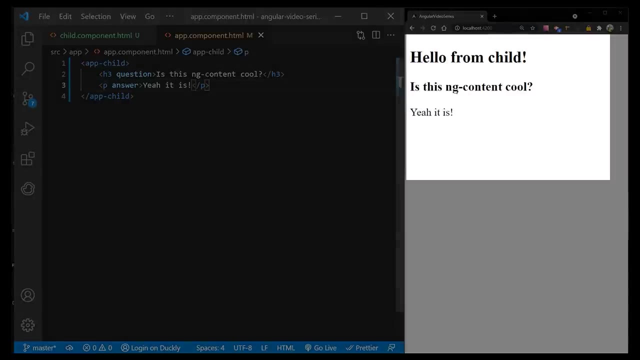 either question selector and I will type this question text Below. I will create a paragraph with an answer selector And I will type an answer text Also. there are a couple other ways to create multi slot content projection, but we haven't covered conditionals yet. As you can see, it's really easy to create reusable. 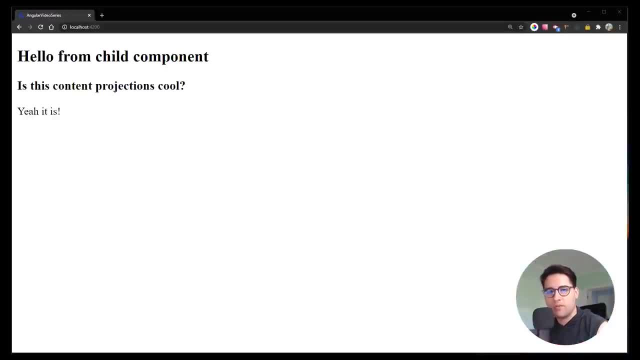 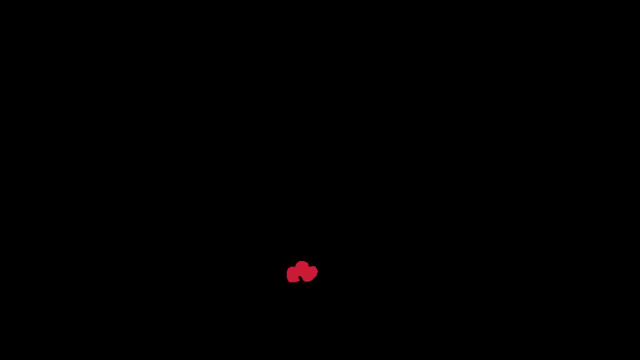 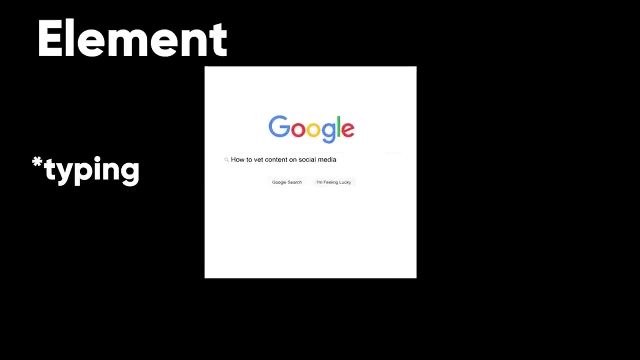 dynamics components. This approach can be used for much more complex user interfaces, But I showed you this simple example to understand the concept. Next, let's discuss template statements. A template statement is something that responds to an event raised by a target like an element. 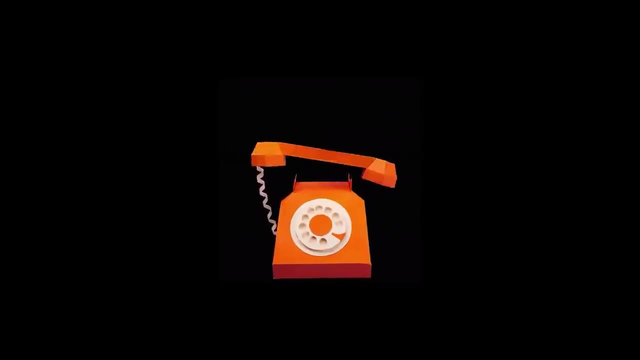 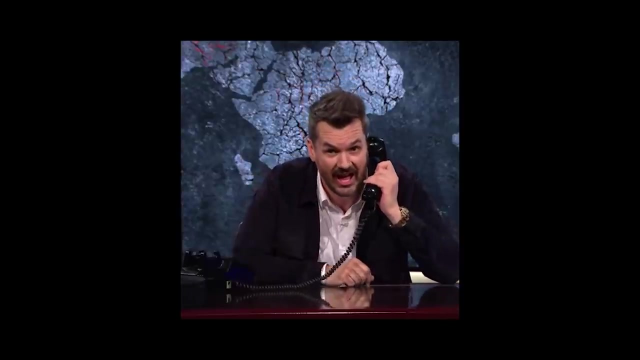 component or directive. So it's the same thing as if someone is calling you, which is an event, and you're answering that phone call, which is the response, and in our example template statement, It commits side effects as it changes the fields in the component. 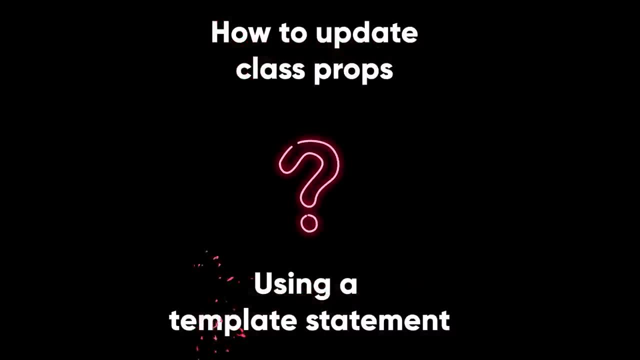 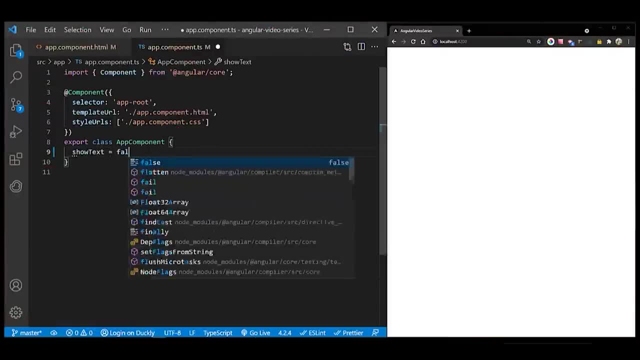 Now I will show you how to update class properties using a template statement. I have a blank component And in our template I will create a boolean property named show text, with a value of false. Below that, I will create a method named toggle text. it's not going to return. 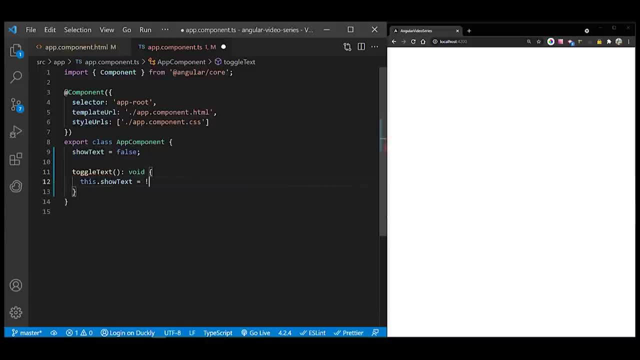 anything at this point. all we are going to do here is to toggle our show text value on every method. Usually we would use this kind of property to toggle the state in the view, But we haven't covered conditionals yet, So in the template I'm going to create a button. it will respond. 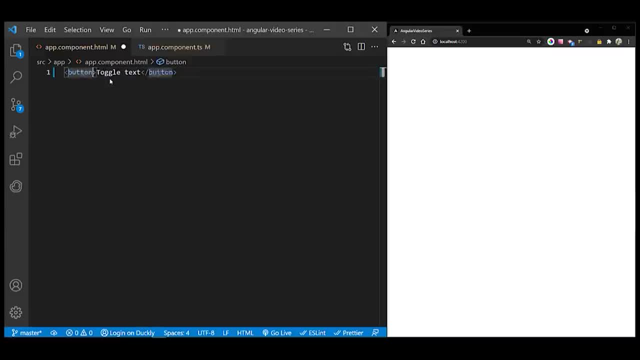 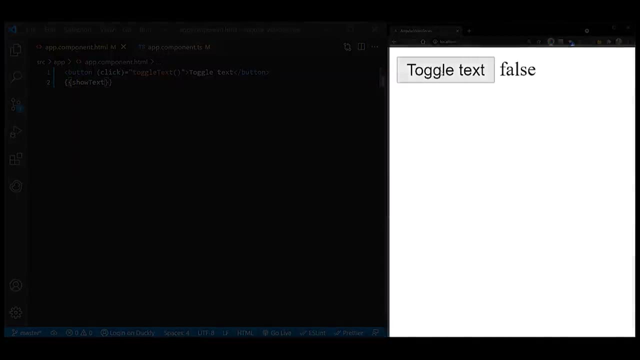 on a click event and it will call this toggle method. Below that I will just display our show text property. And now, when I click the button, you can see that it toggles the its value using template statement And in this example, toggle text is template statement. 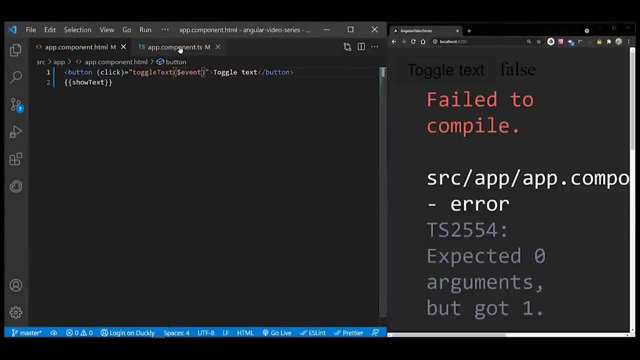 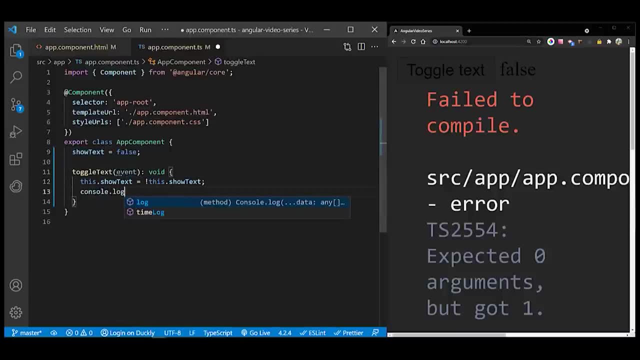 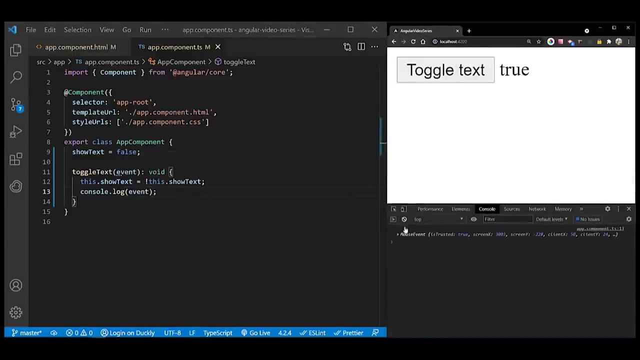 The statement context may also refer to properties of the templates on context. In the following example, toggle text takes a template own event object as an argument. If you log that object you can see that it contains various information about the target and the event that occurred. Passing arguments can be very useful when you're submitting the form. 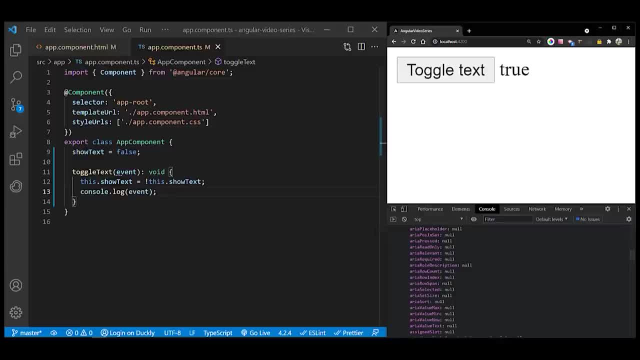 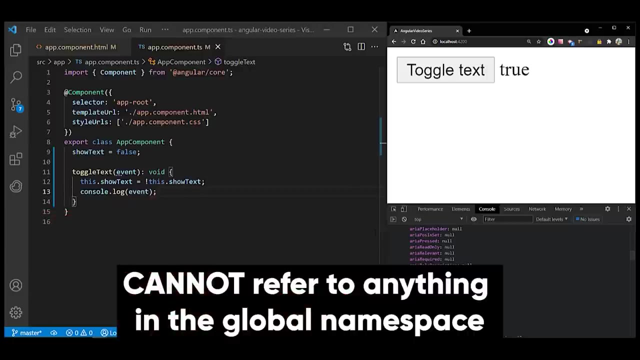 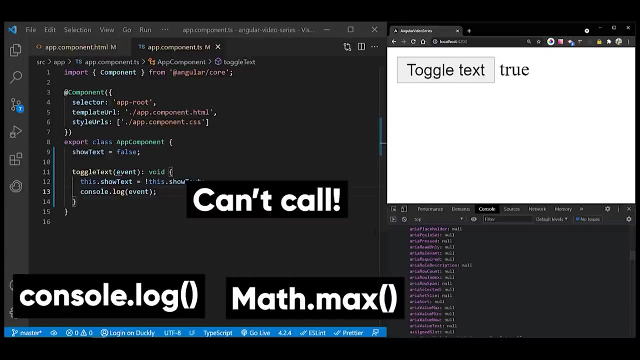 or looping through arrays and you need to access a specific element. One note here is that the context of a template statement can be the component, class instance or the template. Because of this, template statements cannot refer to anything. the global namespace, such as window or document, For example, template statement can call console log or mathmax. 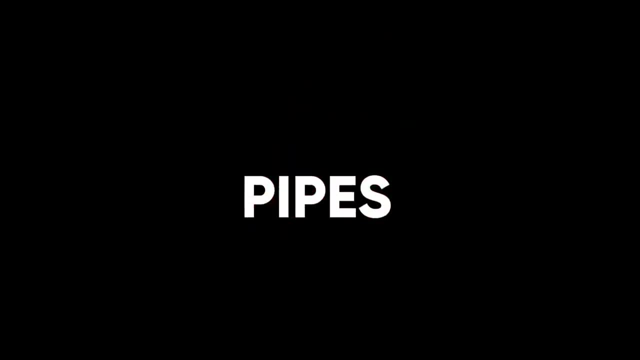 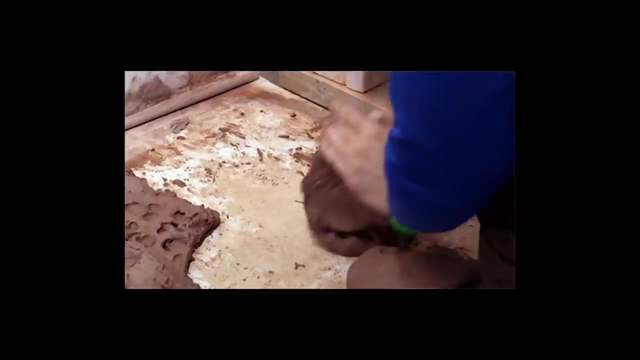 Pipes. Pipes are simply functions you can use in your templates to accept an input value and return a formatted value. In this case you can see your data is untouched clay which is ready to be molded. At the beginning it's not very nice or clear what it's for. 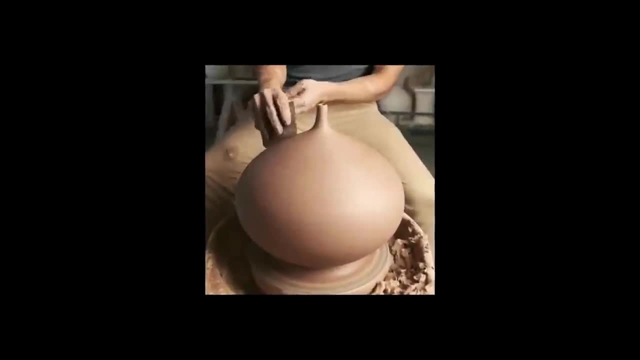 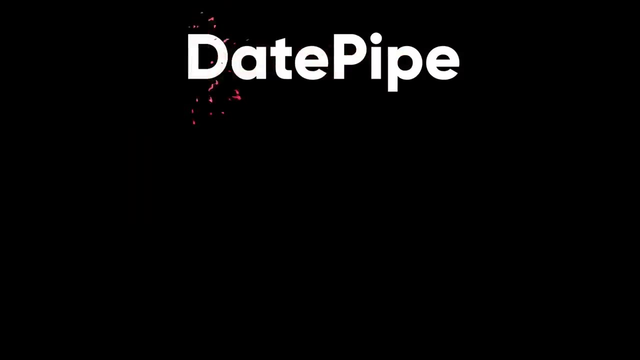 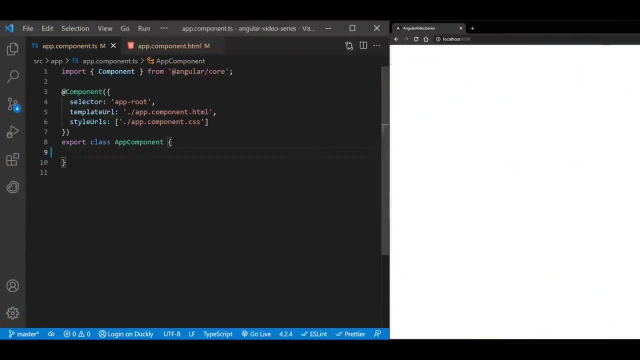 But with a little bit of crafting and modeling you can get the end results that you want. Angular provides built in pipes for typical data transformation, like date pipe, uppercase pipe, currency pipe, percent pipe and similar. In my app component I will define a date property with a value of new date. 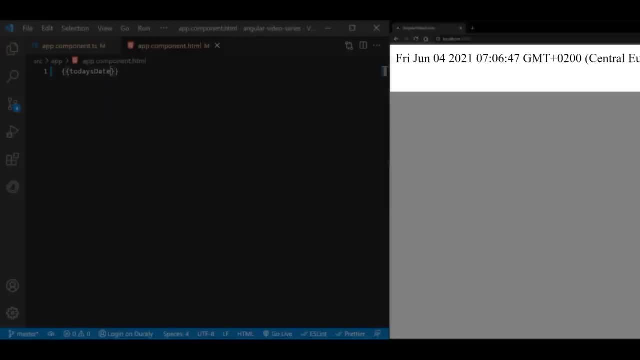 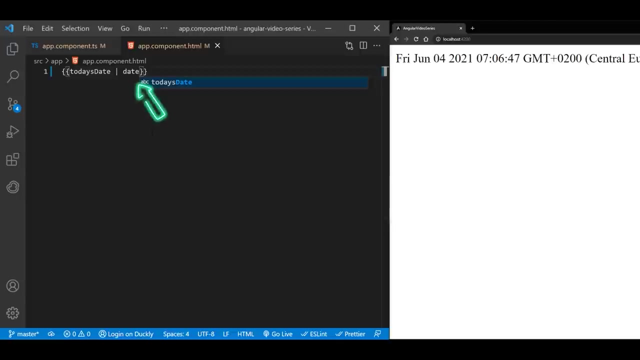 If we just display our date object in our template, you can see what kind of format we get. It's not very user friendly. Now let's make it nicer To apply a pipe. use the pipe operator within a template expression along with the name of the pipe. 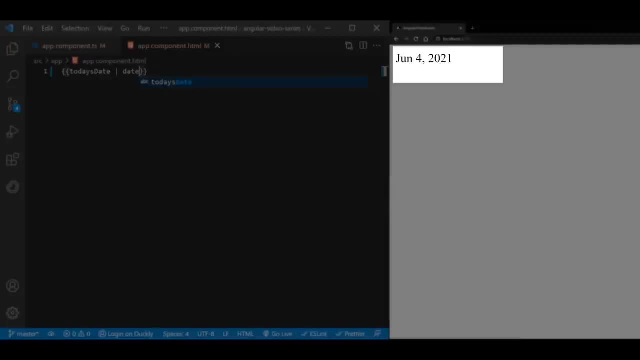 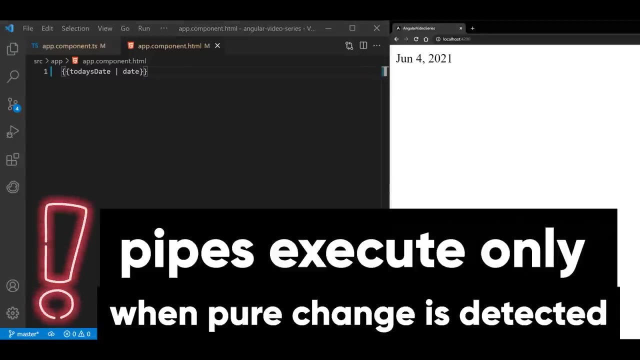 which is the date for the built in date pipe. Now this is much more readable. One note here: date pipe is executed only when it detects a pure change to the input value. A pure change is either a change to a primitive input value such as string. 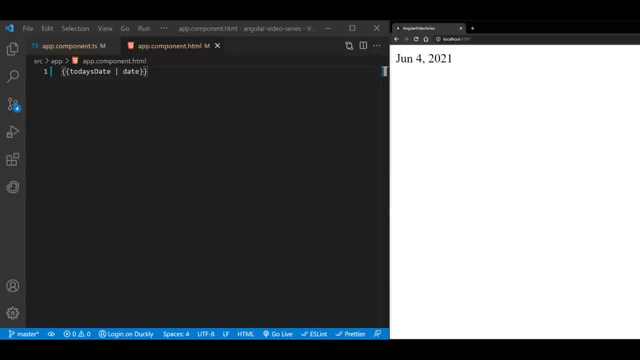 number, boolean or symbol or a change object reference, such as date, array, function or object. If you still don't like the output format for date, you can fine tune it by using optional parameters. There are predefined options like short or long and others. 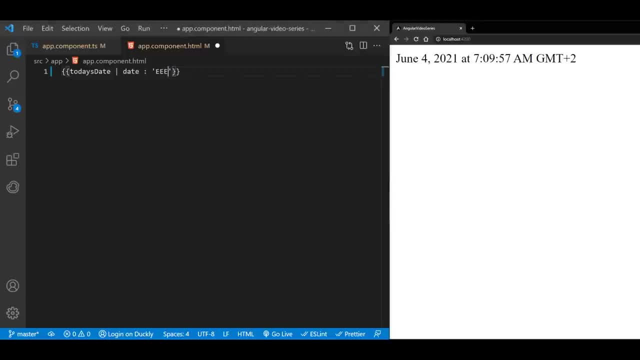 Or you can customize it completely. For example, I'll write four E's for a day in a week, four Ms for a month, one lowercase D for a day in a month and one lowercase Y year. You can also change multiple pipes as well. You just add another pipe operator and a pipe name. 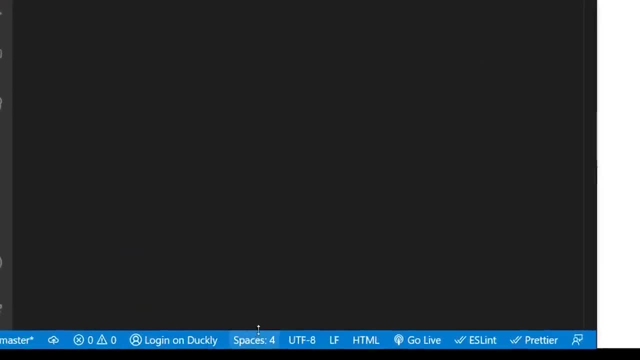 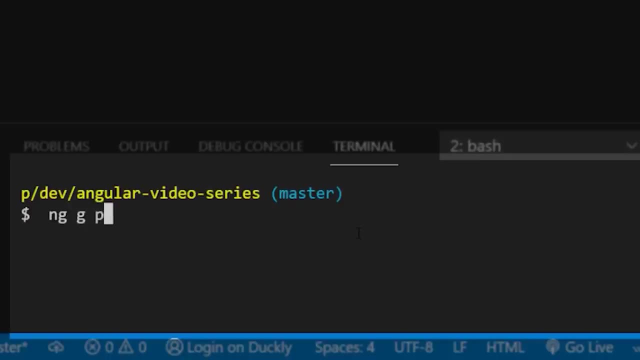 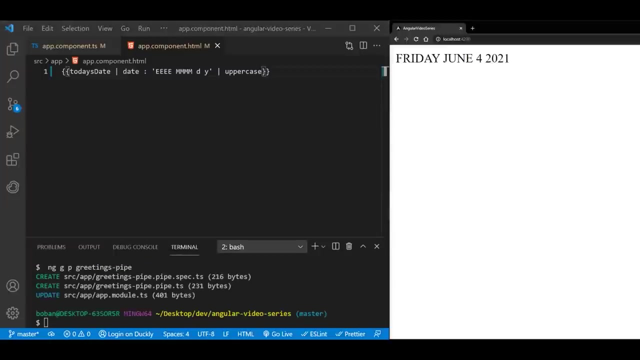 Now we can create custom pipes as well. Let's create a simple greetings pipe that will concatenate hello to past name. I'll use Angular CLI to generate this file for me. So type ng: generate pipe and the name is greetings pipe. In our pipe we have boilerplate code generated. 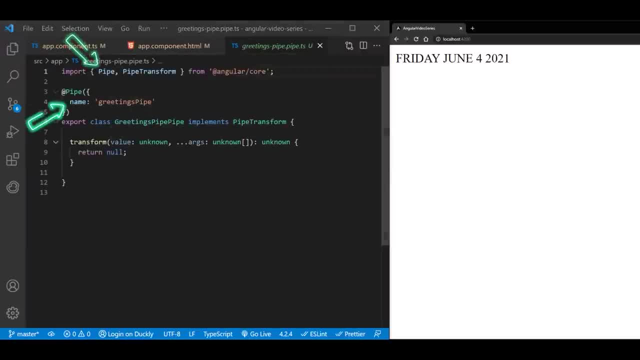 you can see that pipe decorator has been imported with a name property which we can use to call our pipe in our templates. Also, there's a pipe transform interface which needs to be implemented. This interface requires the transform method to be implemented And this method receives a value. 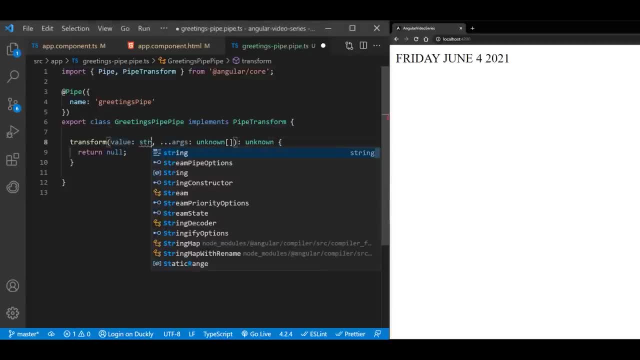 pass from a template. In our case it will be a string, And the second parameter is for optional parameters from pipe itself. return type, in our case, is going to be a string. Now, all we are going to do here is to concatenate hello on the past string and return that. 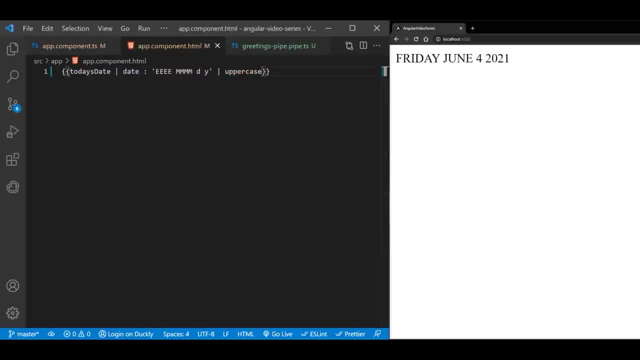 Now in our template, we can call our custom pipe with the greetings pipe name that we defined, and I will pass world as our string. Now that's how you create a custom pipes. Angular pipes are very simple but useful functionality provided by Angular. 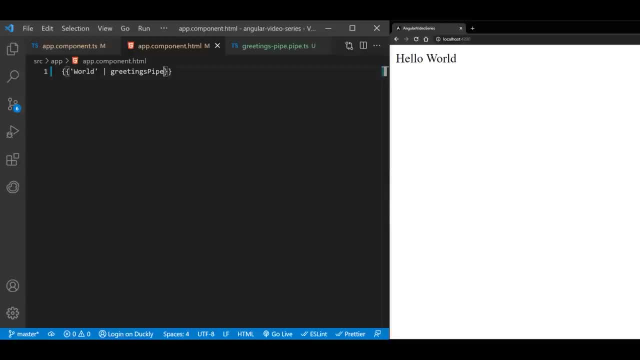 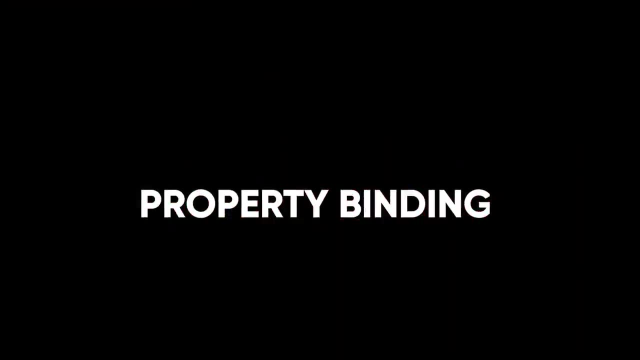 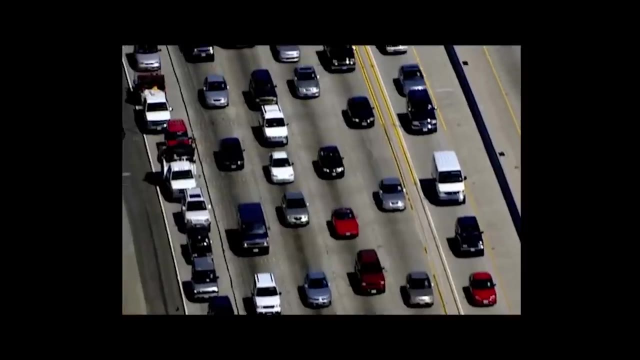 and you will use them a lot. Once again, for a detailed list of all pipes, check the documentation link from the description. Now let's discuss property binding. Property binding moves a value in one direction, So you can see it as one way street. you can go the other way. 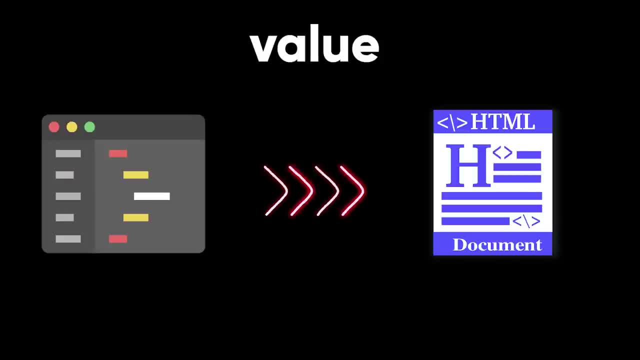 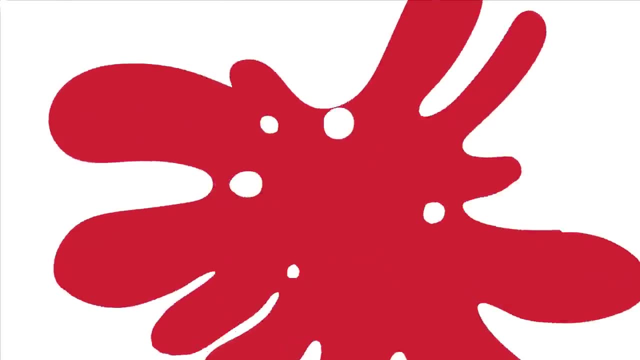 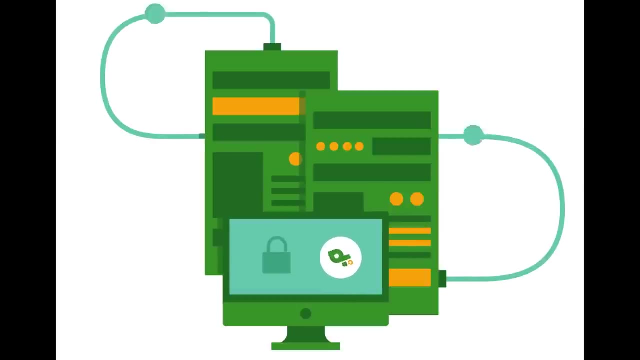 Value goes from class property to target element property. Property binding in Angular helps you set values for properties of HTML elements or directives. With property binding you can do things as Google button functionality, set paths programmatically and share values between components To bind the source property of an image element to a component's property. 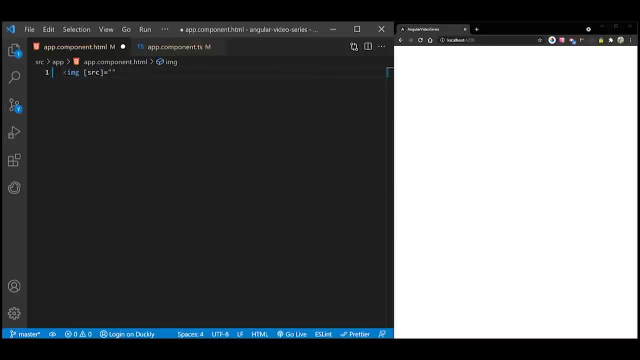 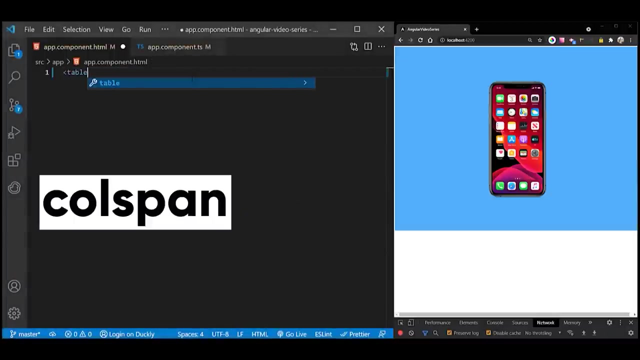 place the target source in the square brackets, followed by an equal sign, and then the property. The property here is item image URL. Declare the item image URL property in the class, in this case app component. A common point of confusion is between the attribute call span and the property call span. 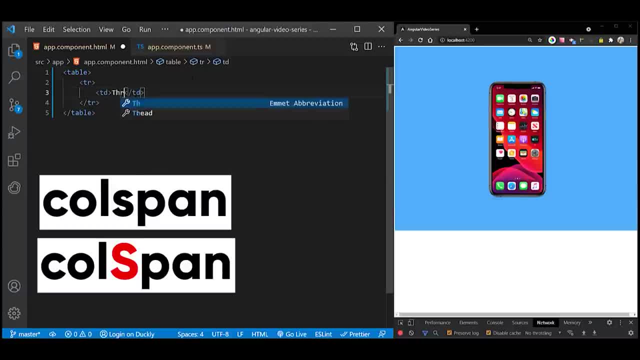 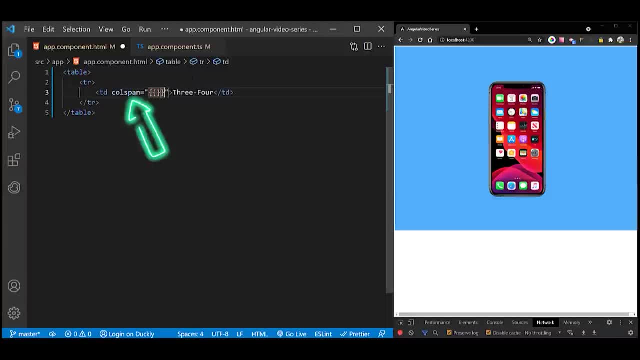 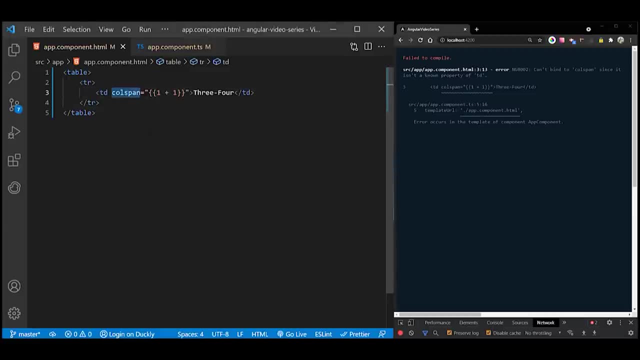 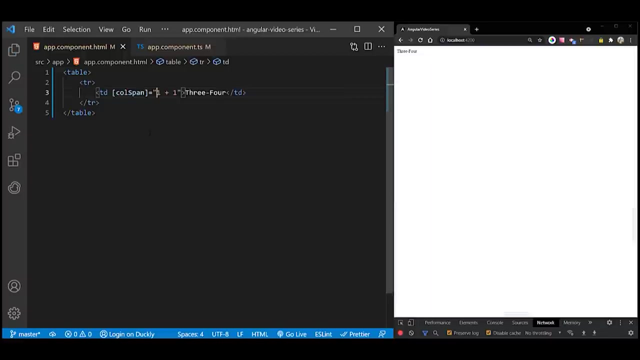 Notice that these two names differ by only a single letter. If you wrote something like this, you'd get template parse error, Interpolation and property binding can set only properties, not attributes. Instead, you'd use property binding and write it like this: Another example is disabling a button when the component says that it's unchanged. 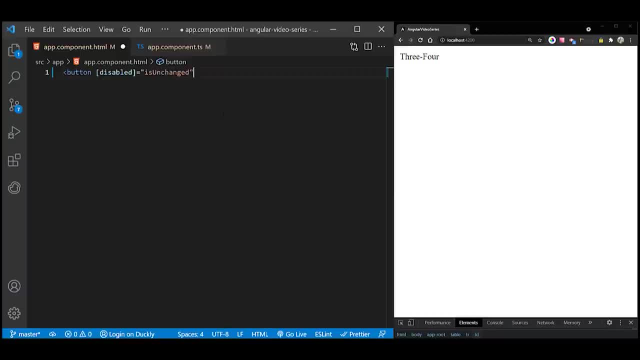 To disable a button's functionality depending on a boolean value. bind a DOM disable property to a property in the class that's true or false, Because the value of the property is unchanged. is true in the app component. Angular disables the button. Often interpolation and. 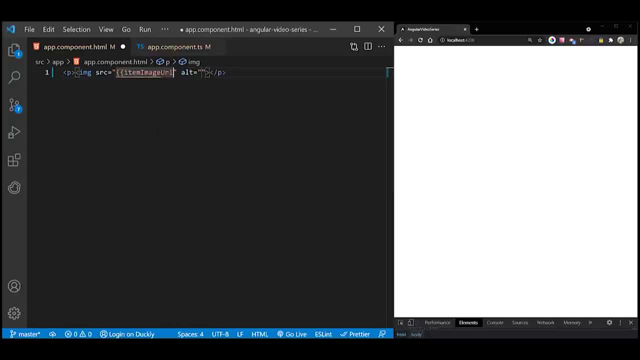 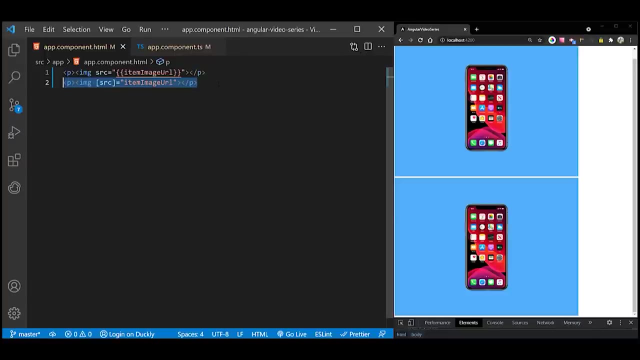 property binding can achieve the same result. The following binding pairs do the same thing. One note: Evaluation of a template expression should have no visible side effects. You shouldn't be assigning anything in the template expression or using increment or decrement operators. If you had an expression that changed the value of something else that you were binding. 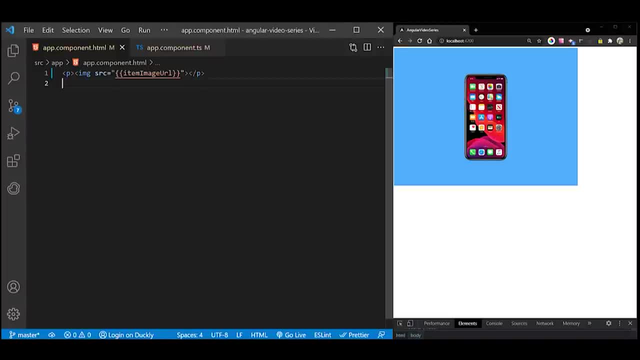 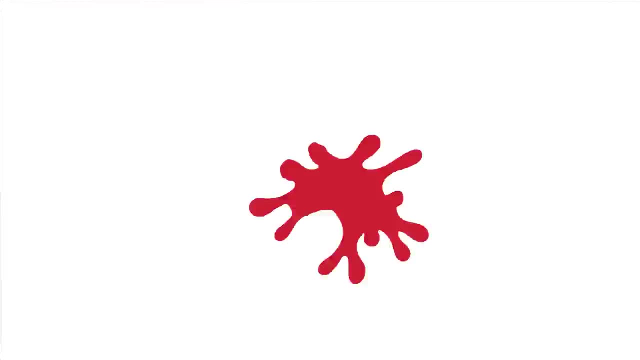 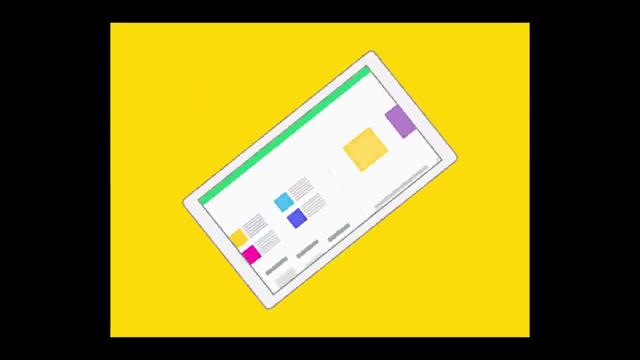 to the change of value would be a side effect. Now let's see about our attribute, class and style bindings. Using these bindings, you can improve accessibility, dynamically style your application and update classes on the fly. First, let's talk about attribute binding. Attribute binding in Angular. 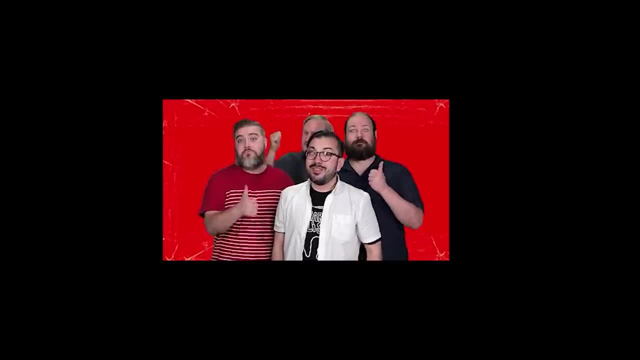 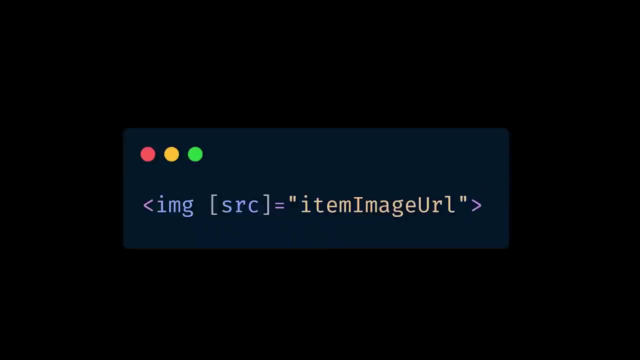 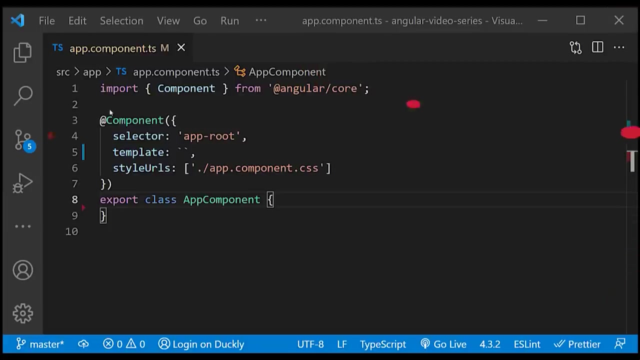 helps you set values for attributes directly. It is recommended that you set an element property with a property binding whenever possible. However, sometimes you don't have an element property to bind. In those situations, you can use attribute binding. Attribute binding- syntax resembles. 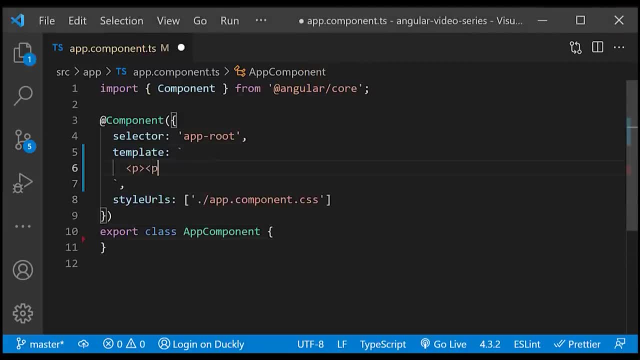 property binding, but instead of an element property. between brackets you precede the name of the attribute with prefix ATTR followed by a dot. Then you set the attribute value with an expression that resolves to a string. Another common use case for attribute binding is with the colspan attribute intables: My 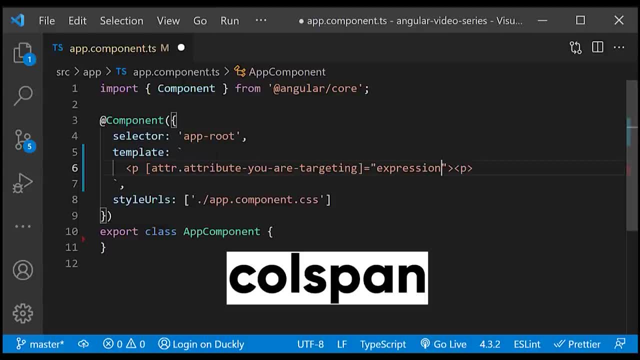 name is colspan and I'm the one who will be binding the attribute. Binding the colspan attribute helps you keep your tables programmatically dynamic, Depending on the amount of data that your application populates. a table with the number of columns that are row span could change. 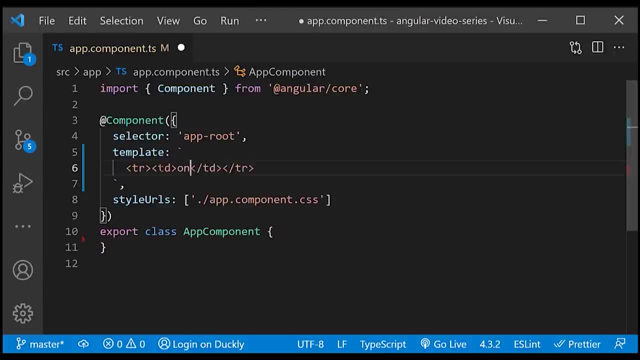 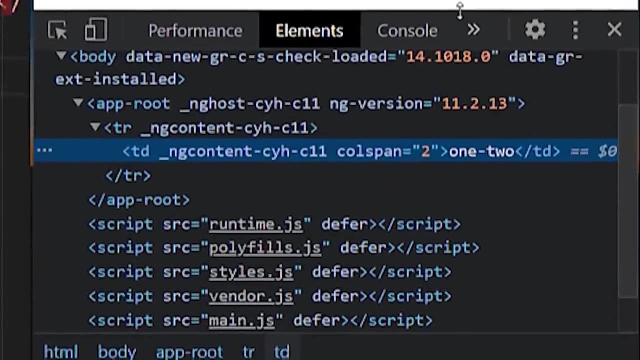 To use attribute binding with the td attribute colspan. specify the colspan attribute. by using this syntax, Set attribute colspan equal to an expression. In this example, we bind the colspan attribute to the expression 1 plus 1.. This binding causes the table row to span two columns. Sometimes there are differences. 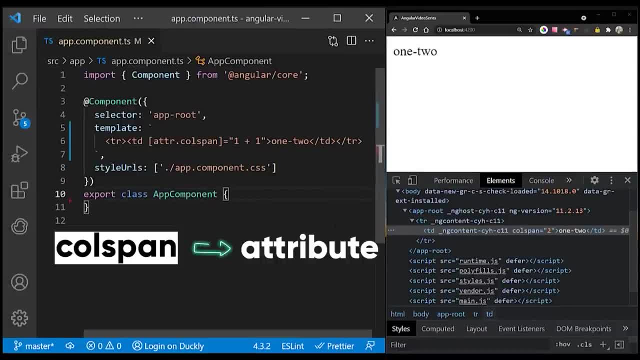 between the name of property and an attribute. Colspan is an attribute of table row, while colspan with a capital S is a property. When using attribute binding, use colspan with a lowercase s. For more information on how to bind to the colspan property, check out the. 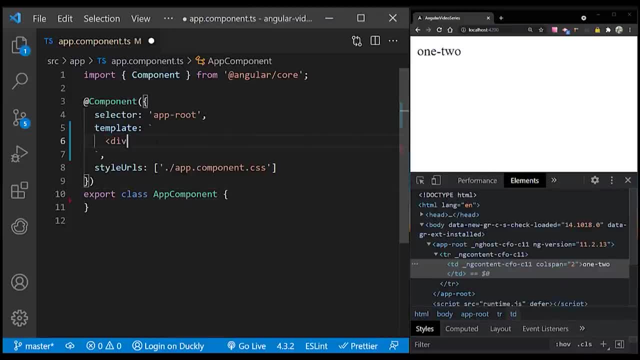 video about the property binding. Now let's move to class binding. You can use class binding to bind to the class binding. You can use class binding to bind to add and remove CSS class names from an elements class attribute To create a single. 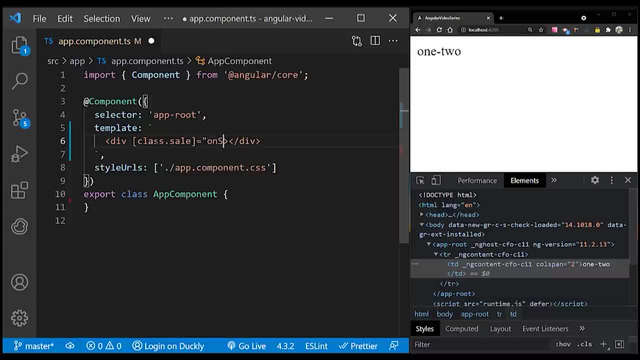 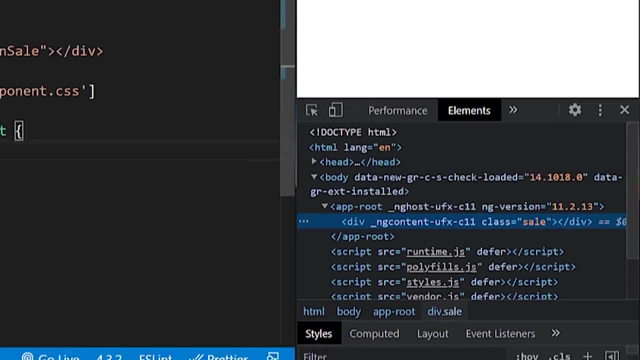 class binding, use the prefix class followed by a dot and the name of the CSS class. Angular adds the class when the bound expression on cell is truthy and it removes the class when the expression is falsy, with the exception of undefined. To bind the multiple class binding: 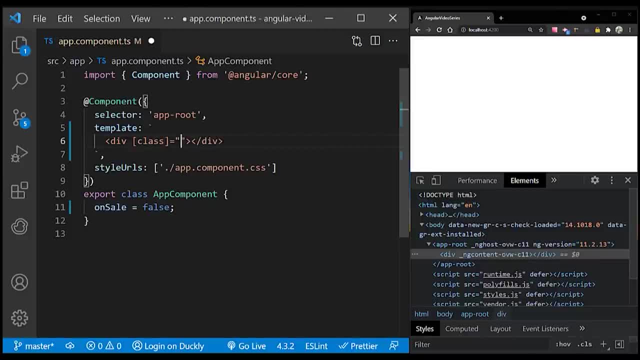 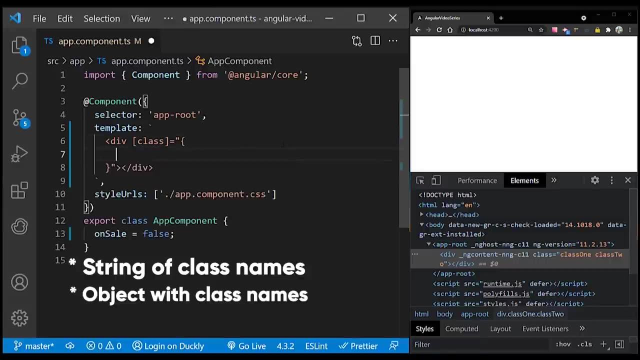 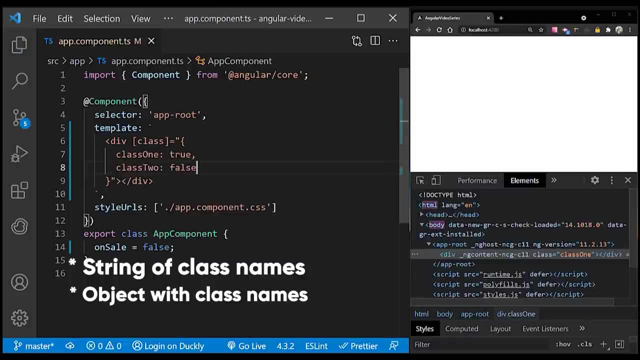 use class set to an expression. The expression can be one of space delimited string of class names. An object with class names as the keys and 30 all fall C expressions as the values. an array of class names With the object formats. class names can be used to add styles and references. We can 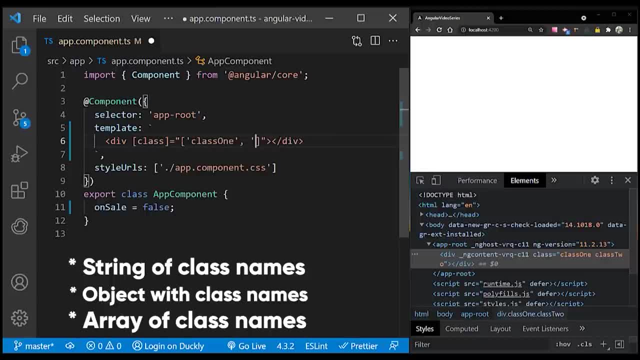 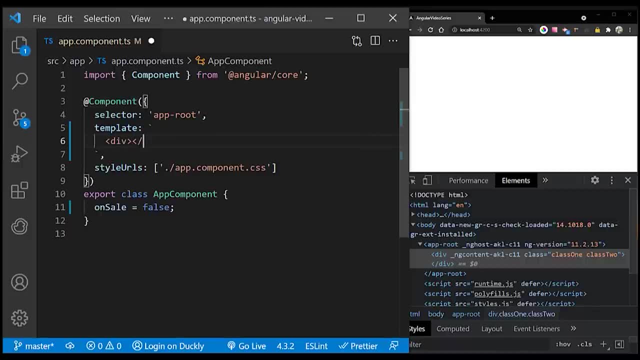 also speed up the operation of class names. Now let's create a string of class names. it Angular adds a class only if its associated value is truthy. And finally, let's talk about style binding. You can use style binding to set styles dynamically To create a single. 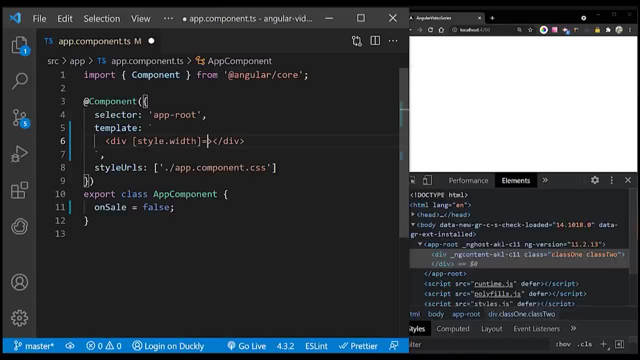 style binding. use the prefix style followed by a dot and the name of the CSS style property. Angular sets the property to the value of the bound expression, which is usually a string. Optionally, you can add a unit extension like M or percentage, which requires a number. 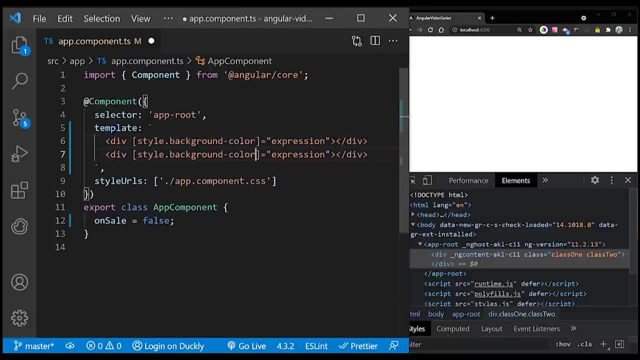 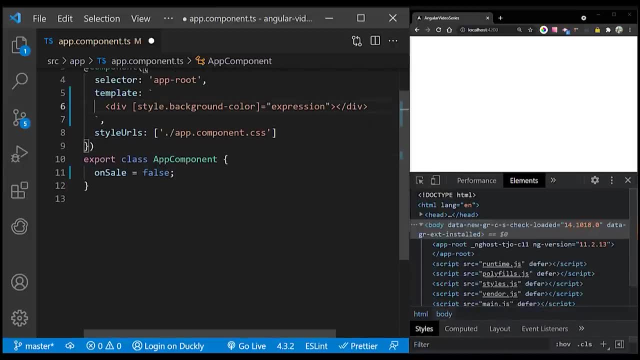 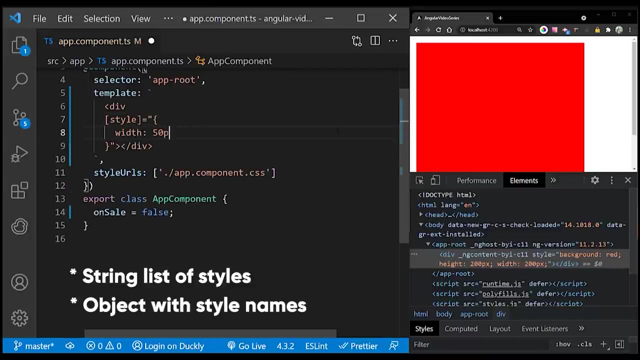 type. You can write a style property name in either dash case or camel case To toggle multiple styles. bind to the style attribute the style expression. The style expression can be one of a string list of styles Or an object with style names as the keys and style values as the values. And note that 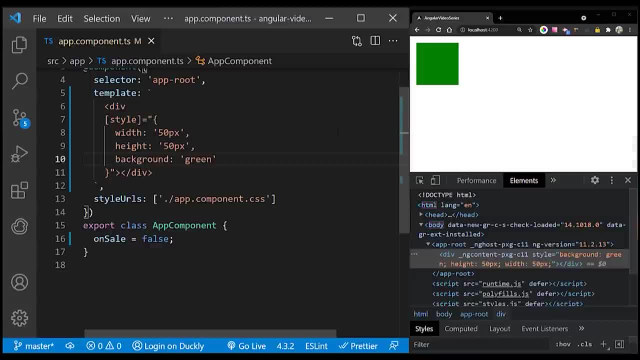 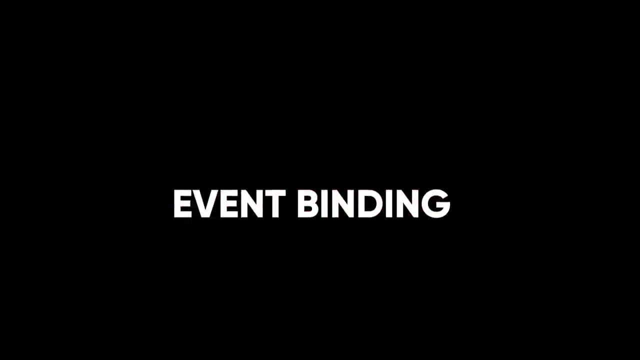 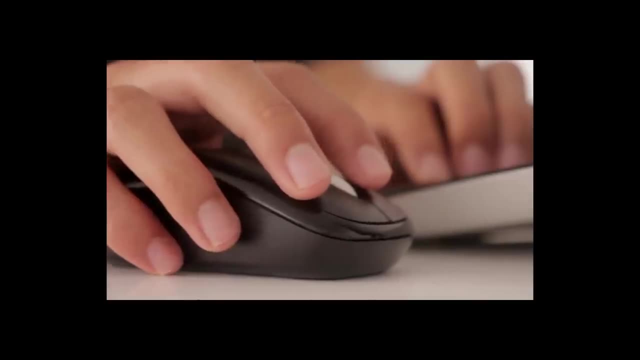 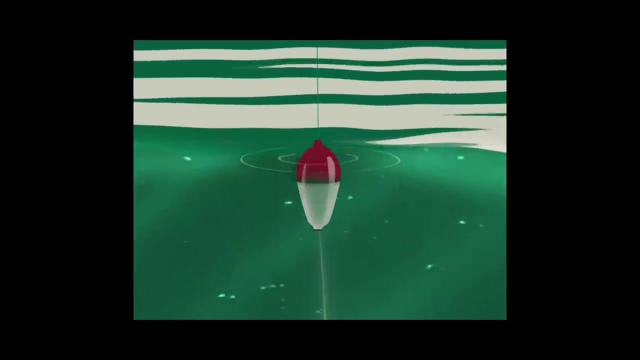 binding, an array to style is not supported. This time I'm talking about event binding. Event binding allows you to listen for and respond to user actions Like keystroke mouse movements, clicks and touches. It's similar to float fishing, as you're waiting for a fish to take your bite and, once it drips off, you respond quickly. 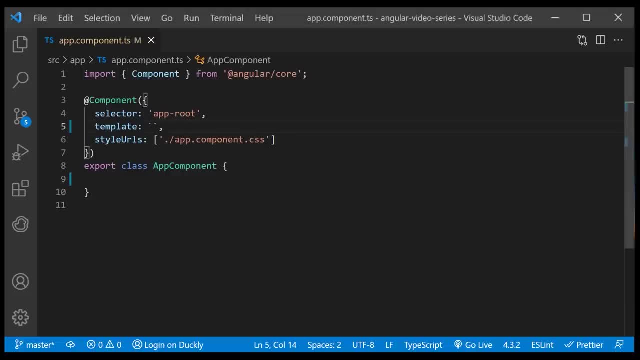 and strike. To bind an event, you'll use the Angular event binding syntax. This syntax consists of an event name, within parenthesis, to the left of an equal sign and a template statement to the right. In this example, the event name is click and the template statement. 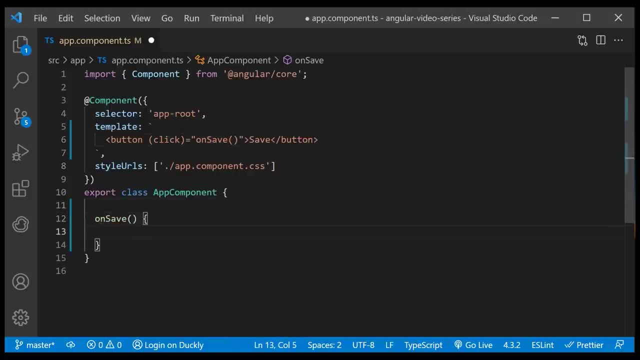 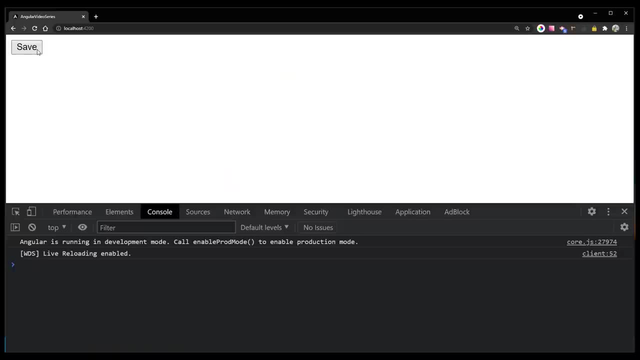 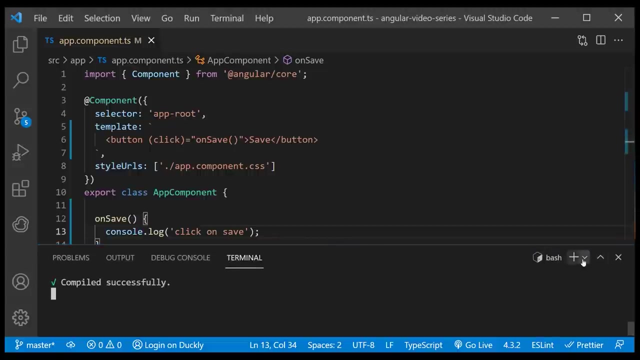 on save. we can now define the on save method in RTS class And once we click our button, that event has been bound and our method is executed. We can also bind to custom events. to demonstrate that, I'll create an item details component. 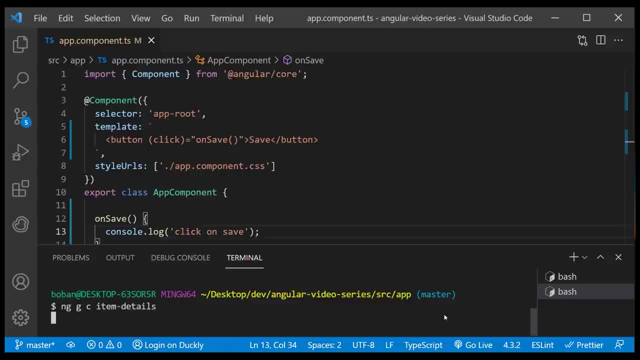 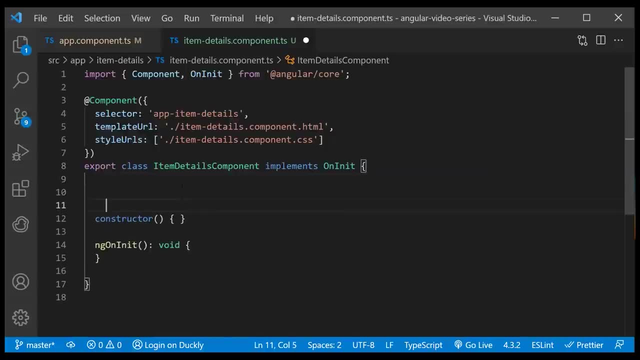 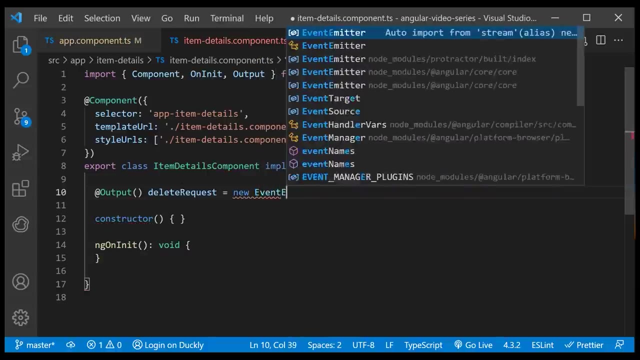 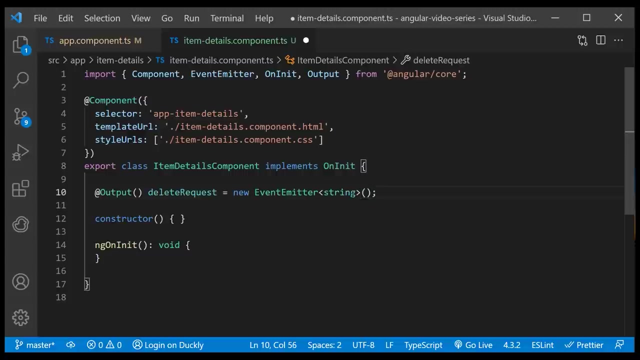 In this component I'll create an event emitter with output decorator which exposes our property to parent components. Then I'll create a delete dummy method which will just emit our property once we call it. Now I'll define a button and bind this method to a click event. 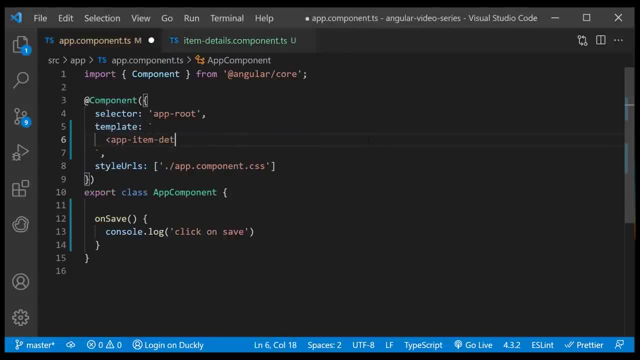 Next I'll place our item details component in our app component and I will bind to the delete request custom event that we just created. I'm calling the lead item method and I'll use the event parameter to cache the string sent with this event. And now I'll define the delete item method in our class and just log. 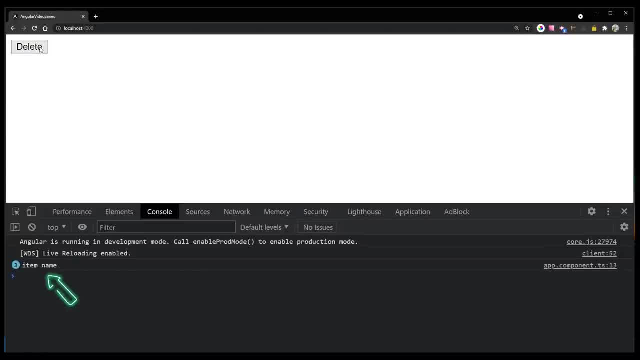 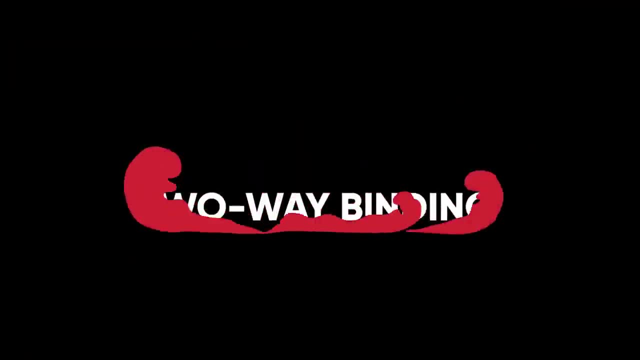 what we got. And that's how you bind to custom event. Now let's see two way binding in action. Two way binding is the concept of sharing and giving. What you give is what you can expect. And that's the concept of sharing and giving, The two way binding. 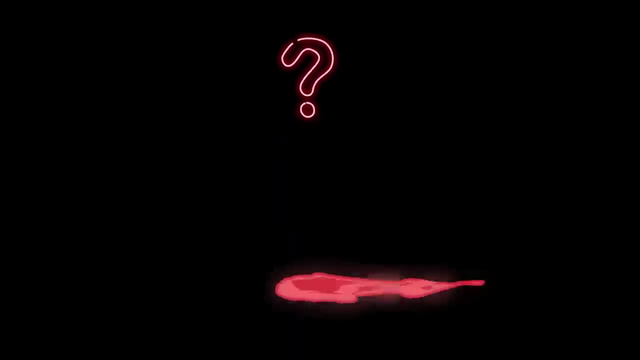 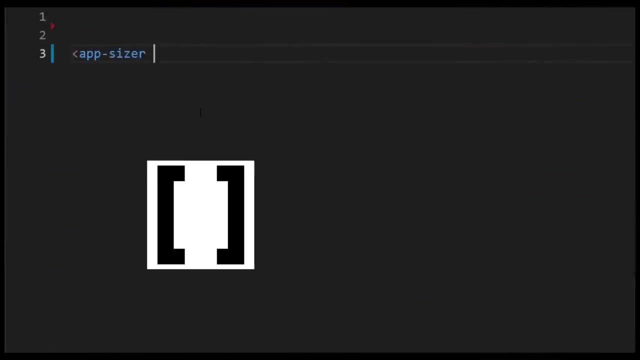 expect from others. Why two-way binding? Two-way binding gives components in your application a way to share data. Use two-way binding to listen for events and update values simultaneously between parent and child components. Angular's two-way binding syntax is a combination of square brackets and parentheses. This 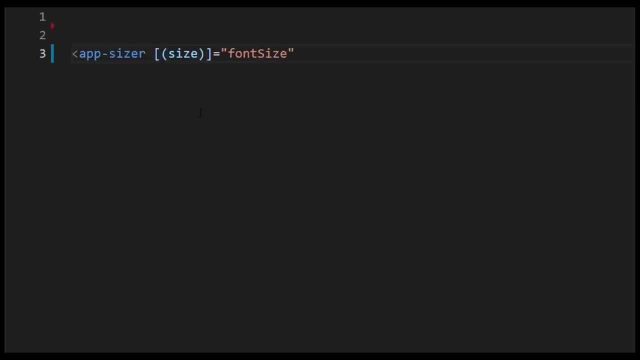 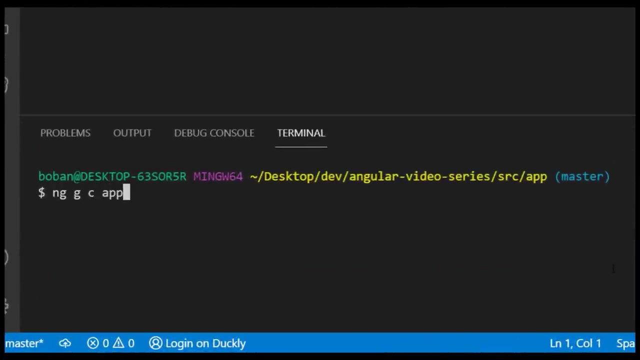 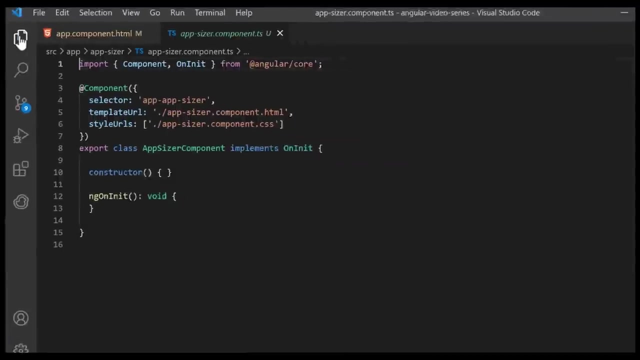 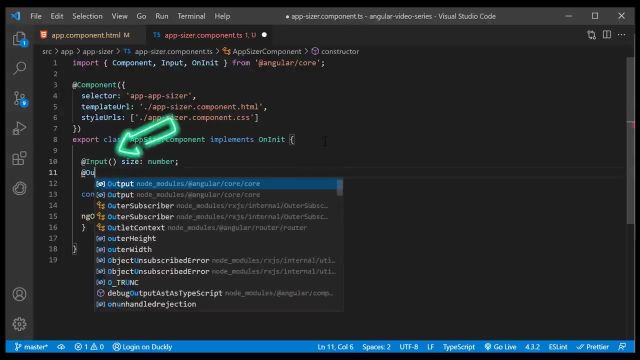 syntax combines the brackets of the property binding with the parentheses of event binding. I'll create a Sizer component In our component. I will define a size value property and a size change event. The size property is an input so data can flow into the Sizer component. 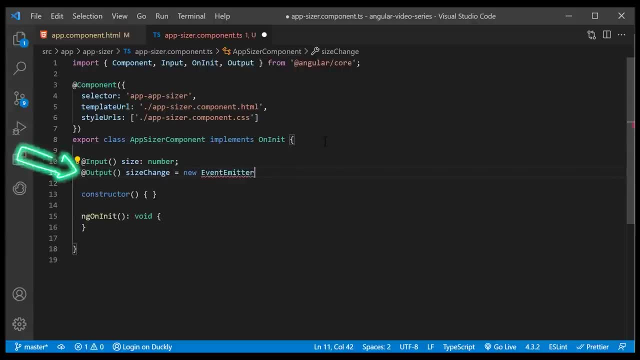 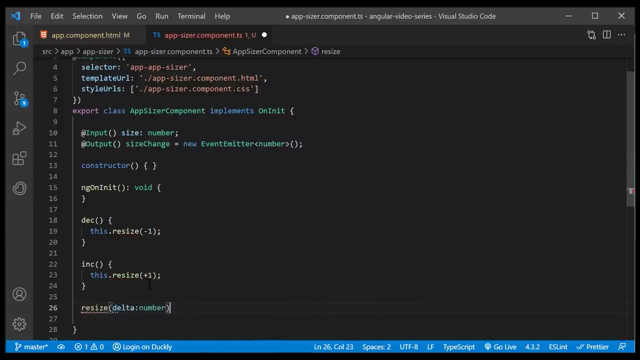 The size change event is an output which allows data to flow out of the Sizer component to the parent component. Next, there are two methods: Dec. to decrease the font size and Inc. to increase the font size. These two methods use resize to change the value of the size property within. 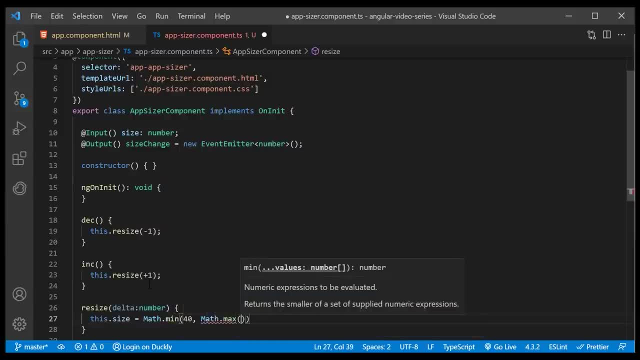 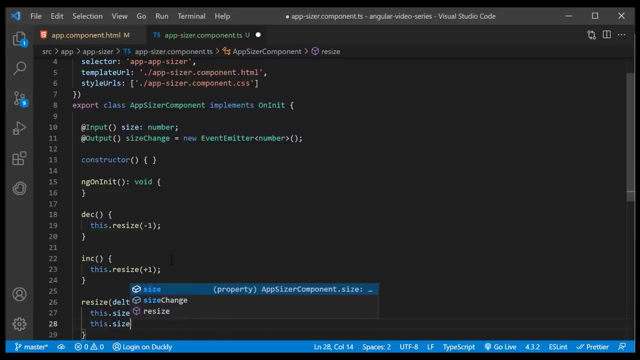 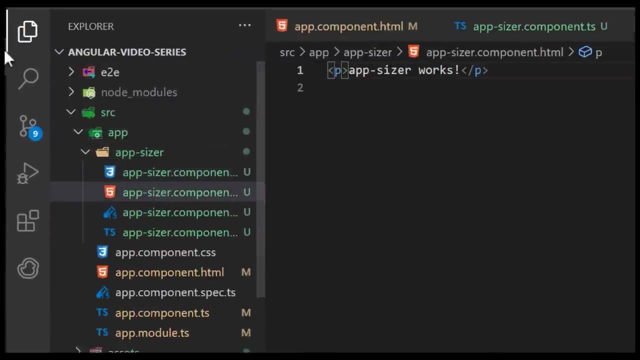 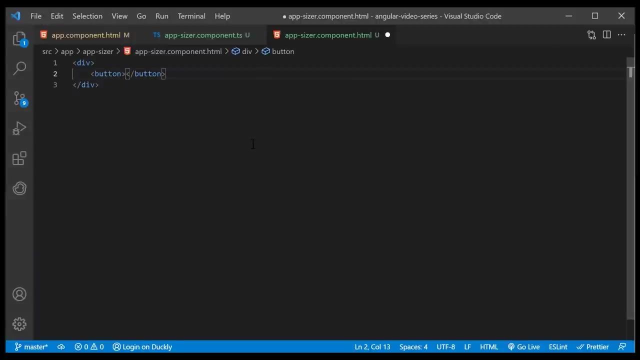 min max value constraints and emit an event that conveys the new size value In the sizer component template. I'll create two buttons that each bind the click event to the ink and deck methods. When the user clicks one of the buttons, the sizer components called the corresponding method, Both methods. 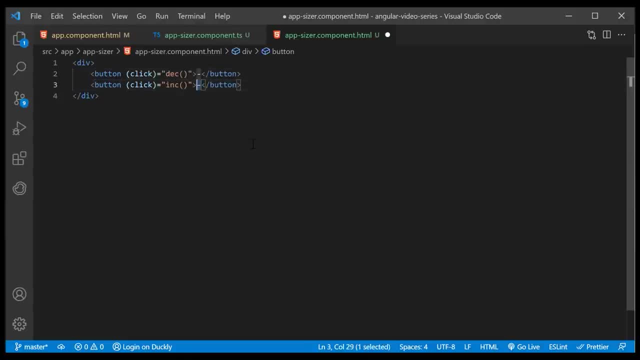 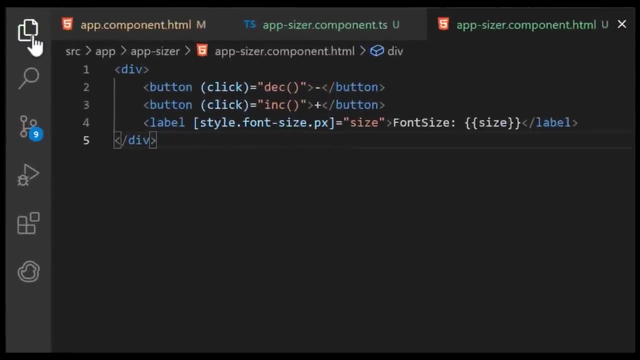 ink and deck called the resize method, with a plus one or minus one, which in turn raises the size change event with the new size value, And below them I'll add a label which displays the size property and dynamically updates its own font size In our root app component. 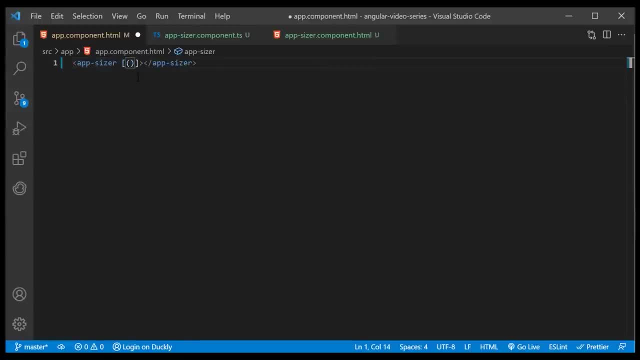 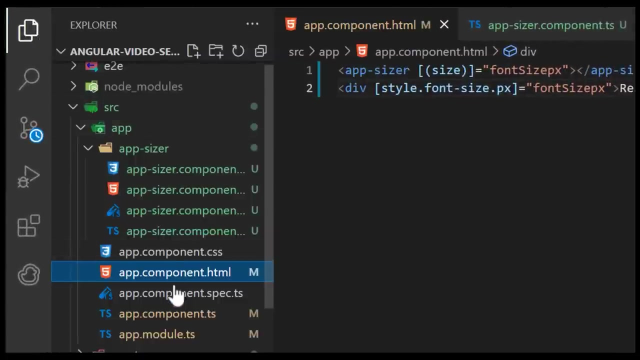 I'll include an app sizer component and I will use two way binding to bind font size px property to the sizer component, And below that I'll add a div which will utilize this property to adjust its text size In the app component. font size px establishes the initial sizer component size value by. 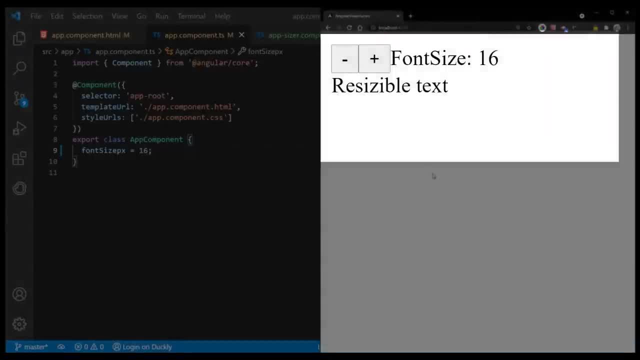 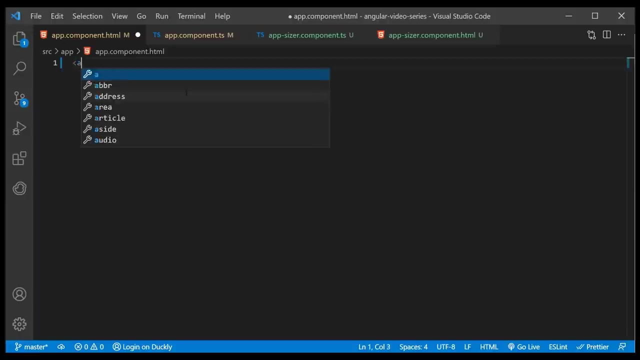 setting the value to 16.. Clicking the button updates the app component. font size px. The revised font size px value updates the style binding which makes the display text bigger or smaller. The two way binding syntax is shorthand for a combination of property binding and event. 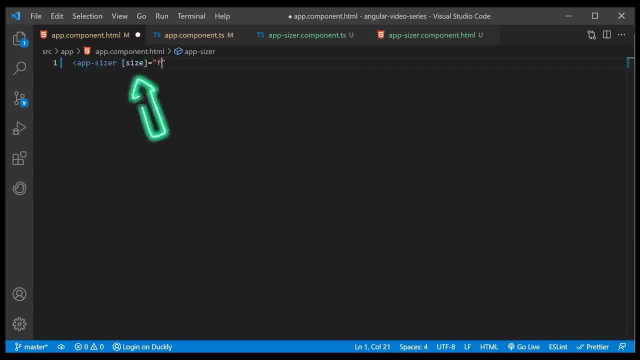 binding. The sizer component binding as separate property binding and event binding is as follows: The event variable contains the data of the sizer component size change. event Angular assigns the event value to app component font size: px and the user clicks the buttons. 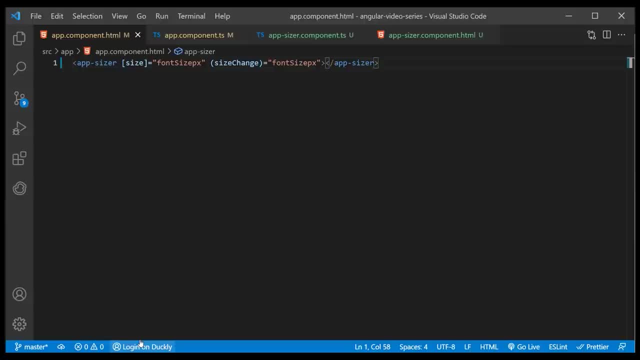 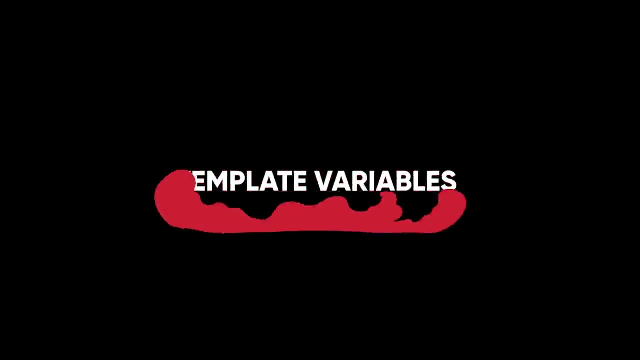 To use two way binding with form event binding, we need to set the size change event value to 0.. To use two way binding with form elements, we need ng model, which I will cover in the form section. Next ones are template variables. 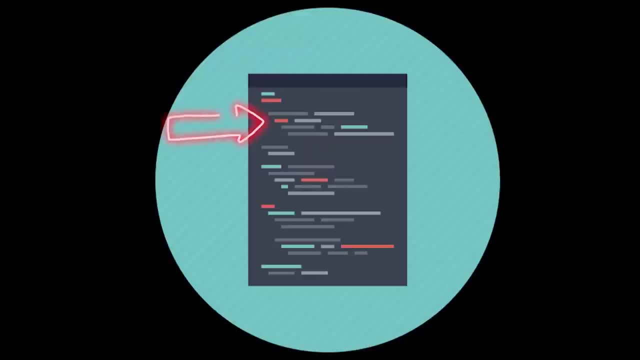 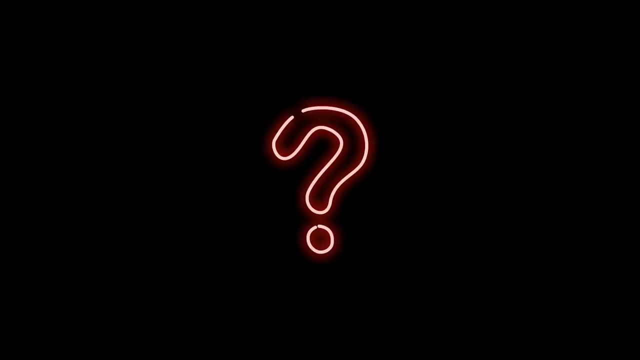 Template variables helps you to use data from one part of a template in another part of a template. It's a variable that is created in and identifies a component or element within the template itself. So it's like a phone number of a component that you can use to. 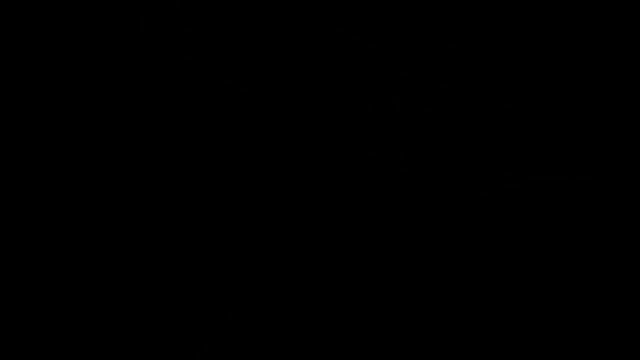 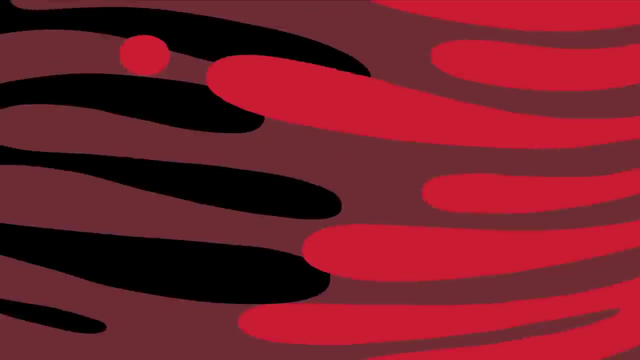 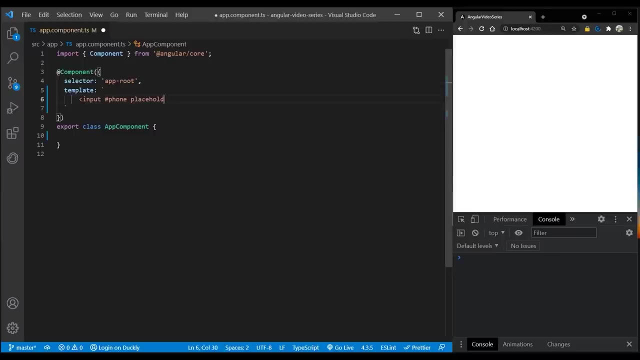 call it in case you need something from it. With template variables you can perform tasks such as respond to user input or finely tune your application's form Syntax. In the template you use the hash symbol to declare a template variable. The following template variable- phone- declares a phone variable on an input element You can refer. 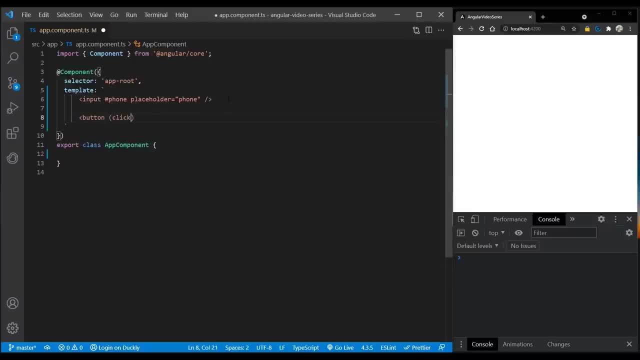 to a template variable anywhere in the component's template. Here, a button further down, the template refers to the phone variable. Now we can define the call phone method and log the passed value, which is the actual value of the input. So what is the template variable? scope? You can refer to a template variable anywhere. 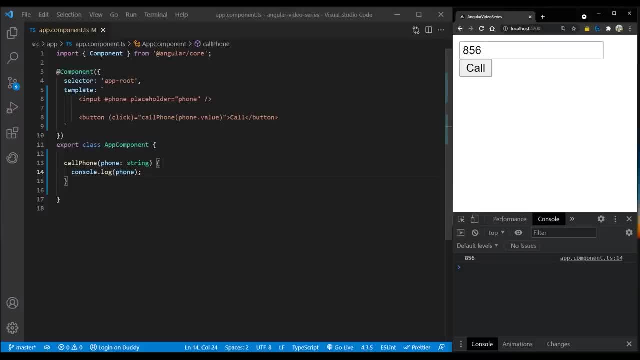 within its surrounding template. Central directives such as ng-if and ng-for, which we'll cover in the later videos- or ng-template, act as a template boundary. You cannot access template variables outside of these boundaries. So can we access variables in a nested template, An inner template can? 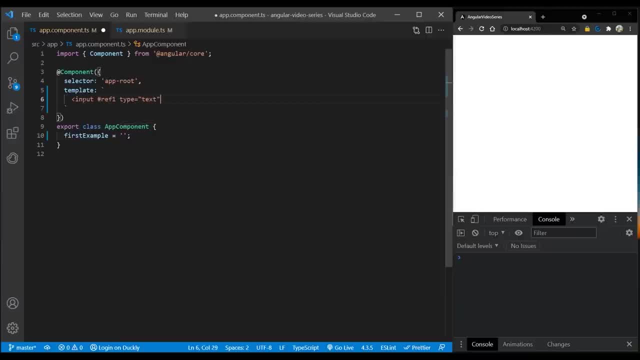 access template variables that the outer template defines In the following example: changing the text in the input changes the value in the span because Angular immediately updates changes to the template variable ref1.. In this case there is an implied ng-template around the span and the definition of the 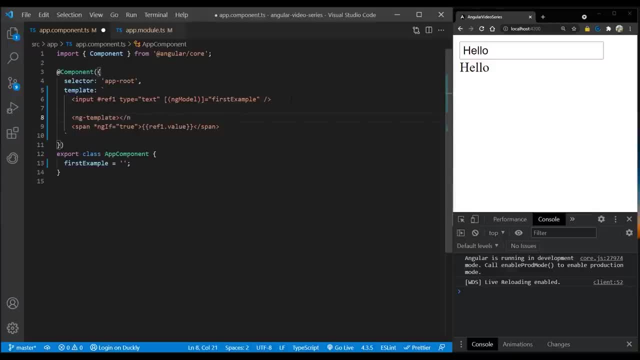 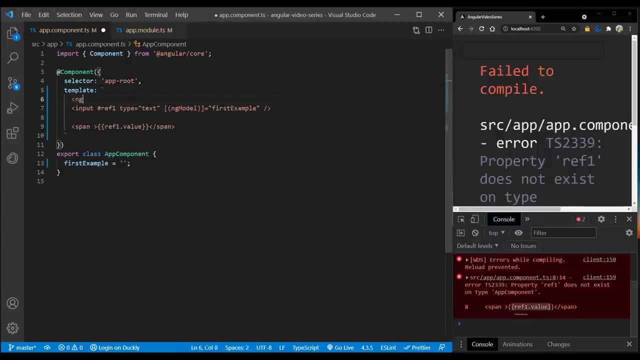 variable is outside of it. So it's the same thing as writing explicitly like this: How do you define a template variable? However, accessing a template variable from outside the Balance template doesn't work. It's the same as writing the following: Ist-DA. 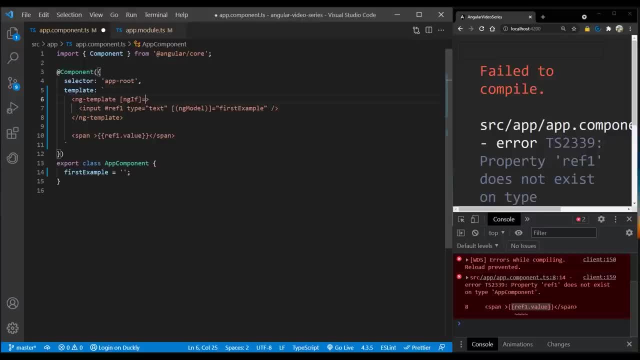 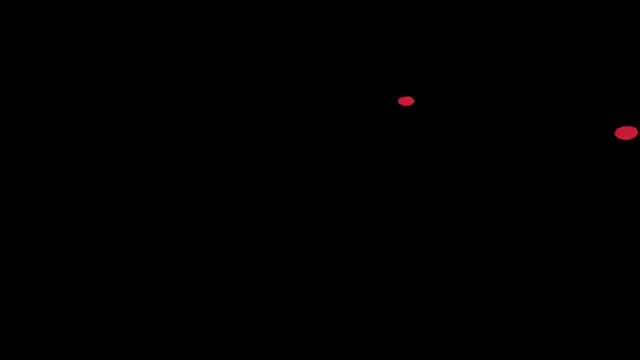 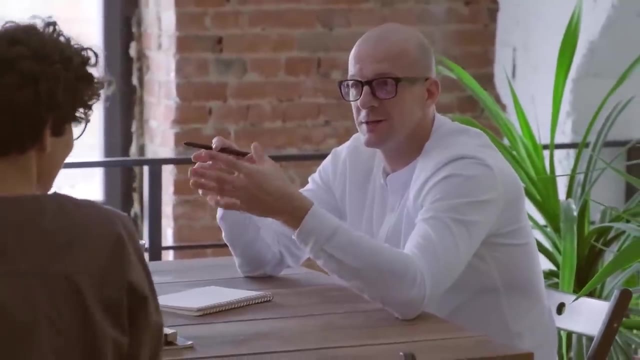 For that example, we just changed the index to: are there from interest " Filipino Mm, Let's do the 2019 Text 한번 Now from policy: hele chlusscom, Connecticutcom, Pacific Northwestcom, and you are giving directives to your employees how to behave and what to do in certain situations. 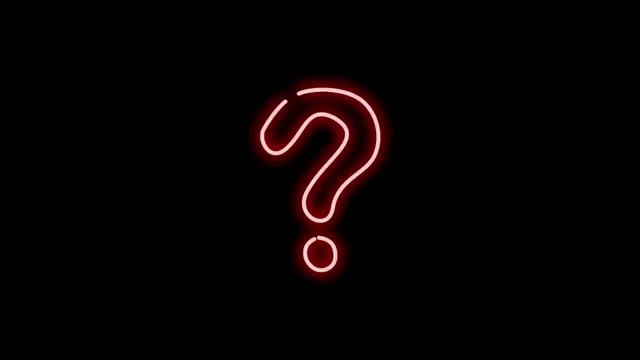 What are directives? Directives are classes that add additional behavior to elements in your Angular application. With Angular built-in directives, you can manage forms, lists, styles and what users see. The different type of Angular directives are as follows: Components directives. 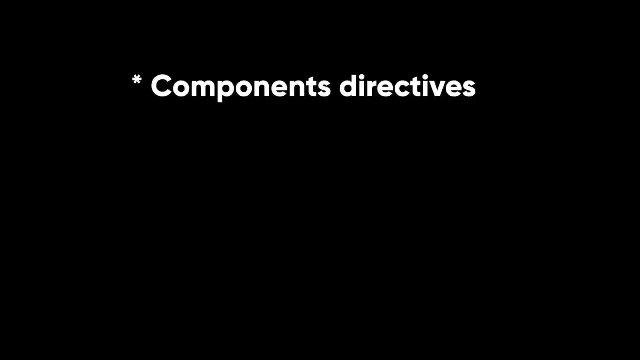 with a template. This type of directive is the most common directive type. Attribute directives: Directives that change the appearance or behavior of an element, component or another directive. Structural directives: Directives that change the DOM layout by adding and removing DOM elements. Today we are talking about built-in attribute directives. Attribute directive listens to and. 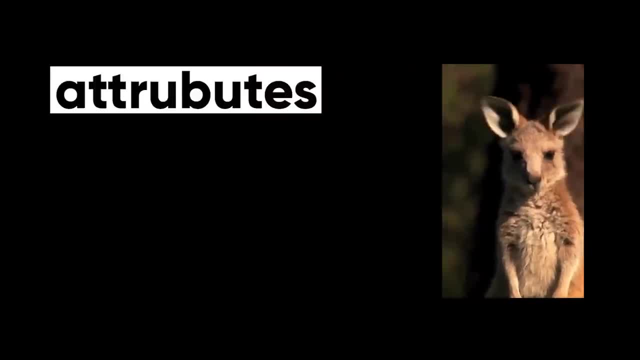 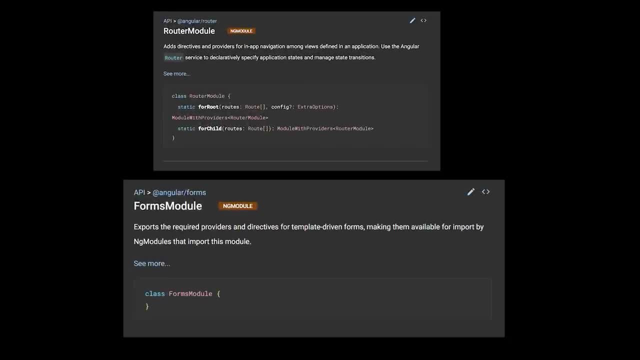 modifies your methods. Additives that change themselves in the DOM layout will be added and replaced with new ones. the behavior of other HTML elements, attributes, properties and components. Many ng modules, such as router module and forms module, define their own. 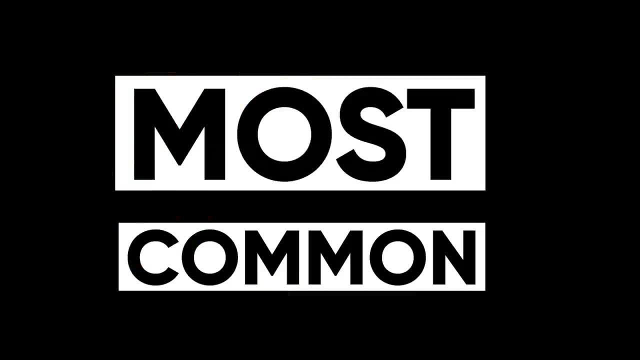 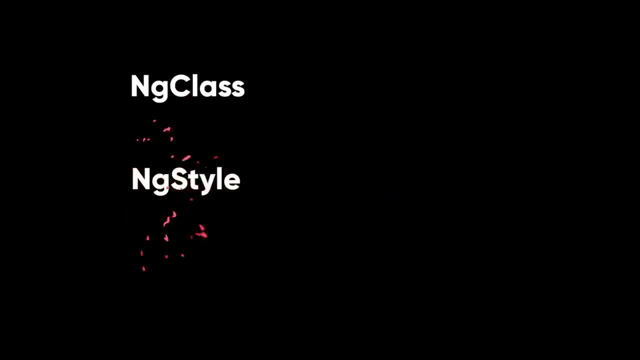 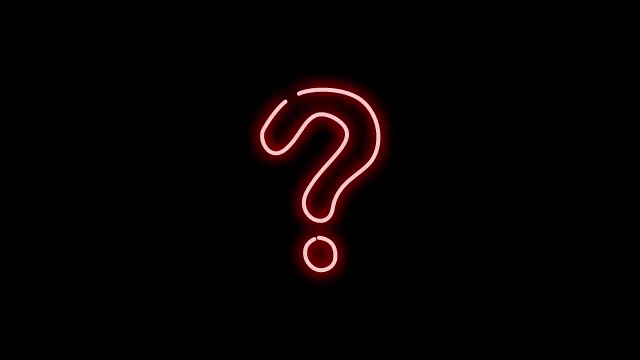 attribute directives. The most common attribute directives are as follows: ng class adds and removes a set of CSS classes. ng style adds and removes a set of HTML styles. ng model adds two-way data binding to an HTML form element. How to add and remove classes: with ng class, You can add or remove multiple CSS classes. 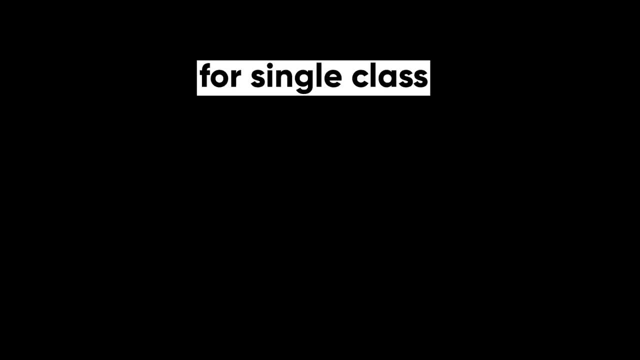 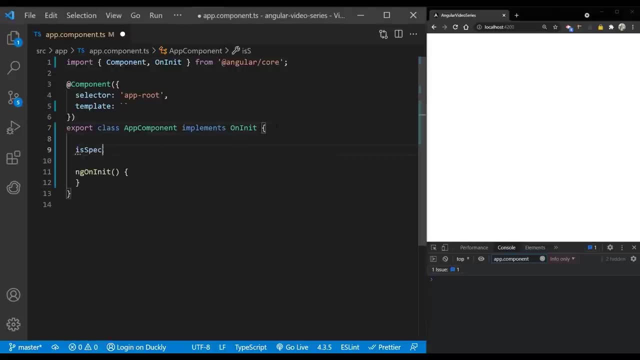 simultaneously with ng class. To add or remove a single class. use class binding rather than ng class On the element you'd like to style. add ng class and set it to equal to an expression In our class. let's define isSpecial as true, Because isSpecial is true, ng class applies. 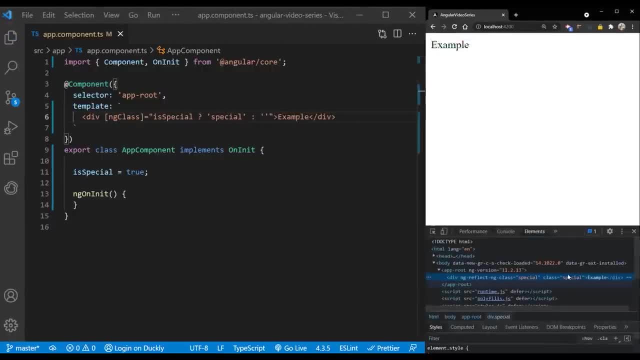 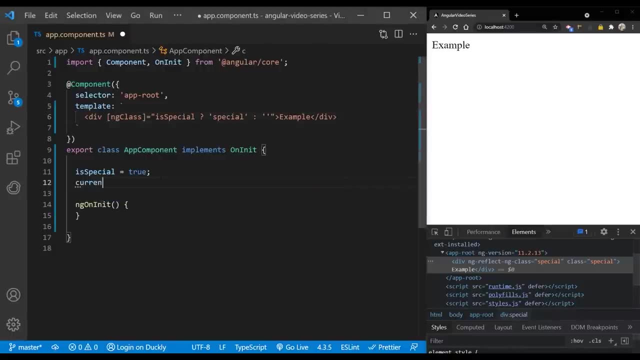 the class of special to the div. To use ng class with a method: add method to the component class In the following example: setCurrentClasses sets the property currentClasses with an object, The object that adds or removes three classes based on the true or false state of three. 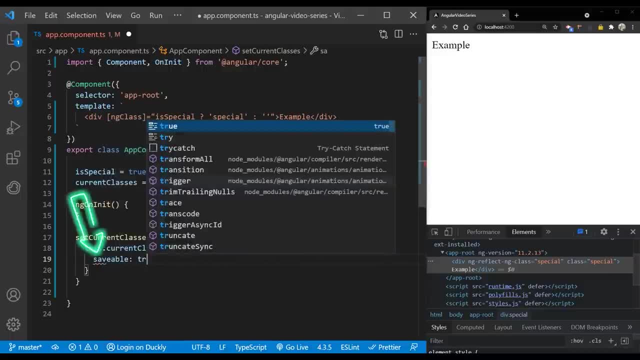 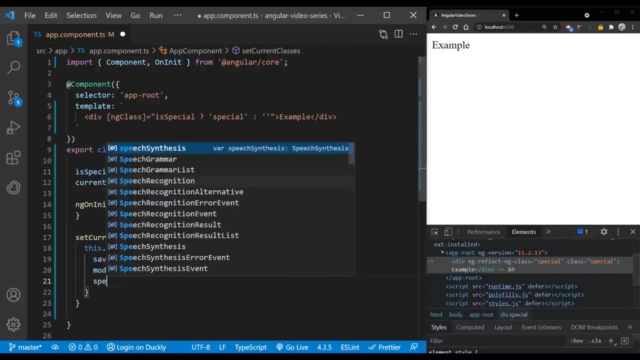 other component properties. Each key of the object is a CSS class name. If a key is a true ng class adds the class. If a key is false ng class removes the class. Boolean values are hard coded just for demonstration In the template. add the ng class property. 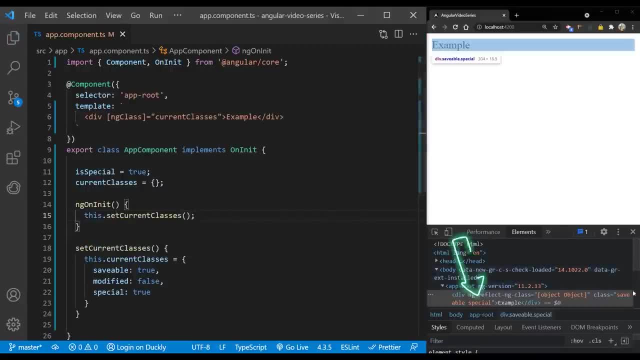 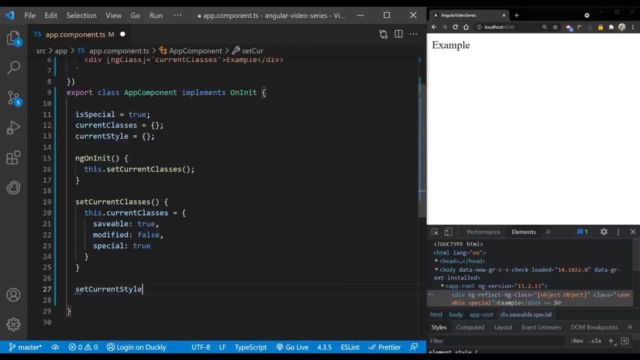 To select a component, add ng cross fashioned. Actually, you can divide it by its std status. Now, now we try to do the same thing. It is difficult to ship style of the element and set for ng class. If your element has a true std status, set the std status. 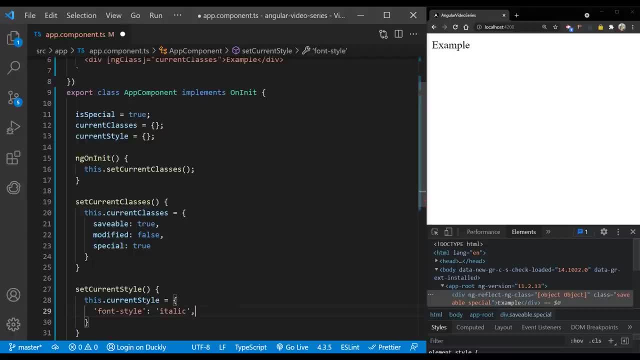 In the following example: setCurrentCני styles when you assign it to a component class. So nG société is set to tag element slash std. Now let's talk about ng style. You can use ng style to set multiple inline styles simultaneously, based on the state of the component. 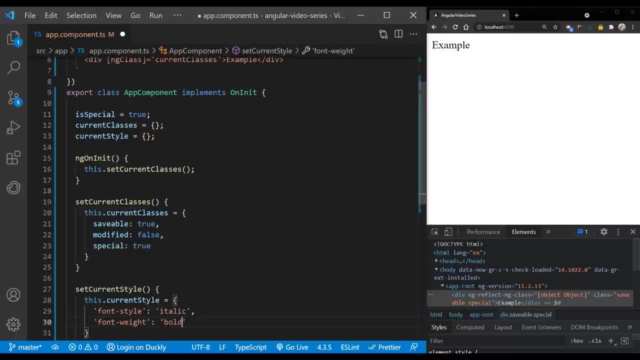 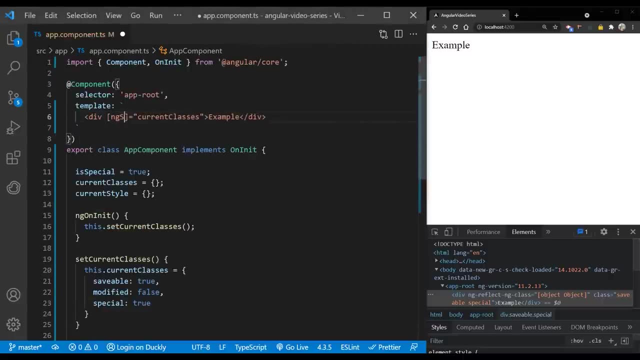 To use ng style: add the method to component class. Add empty object: currentStyle styles. with an object that defines three styles. To set element styles: add an ng style property binding to current styles. For this use case, Angular applies the styles upon initializations. 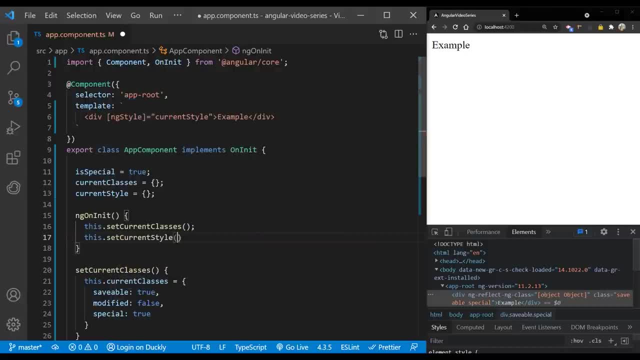 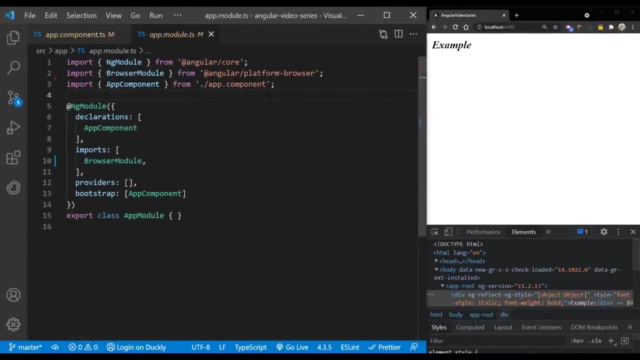 And in case of changes. to do this, the full example called set current styles, initially with ng on in it. And the last one in today's video is ng model. you can use the ng model directive to display a data property and update that property when the user make changes. Import forms. 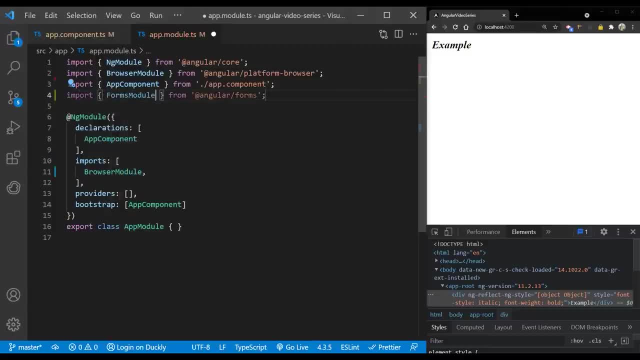 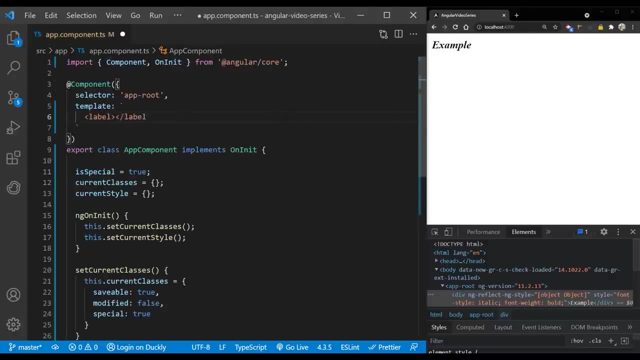 module and add it to ng modules import list. I'll create a label and an input for this example. Add an ng model binding of an HTML form element and set it equal to the property Here, its name. Now, if you define property inside of our component class, 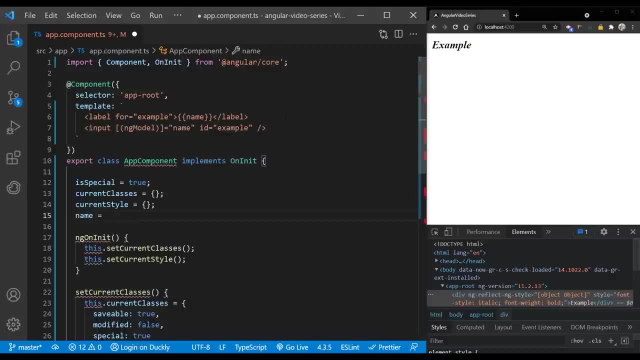 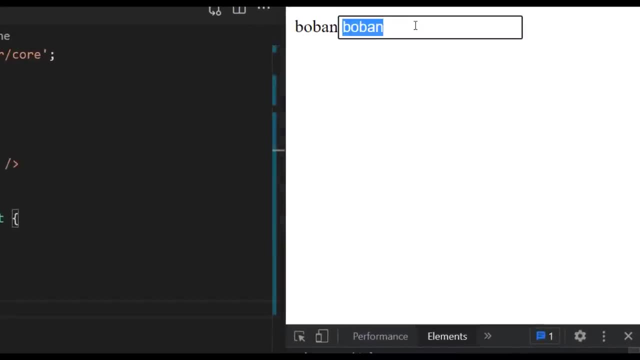 you can see how ng model directive adds two way data binding to our input. This ng model syntax can only set a data bound property. When you write an Angular component, you don't need a value. actually, You just need to define the value of the component. Now, if you define an Angular, 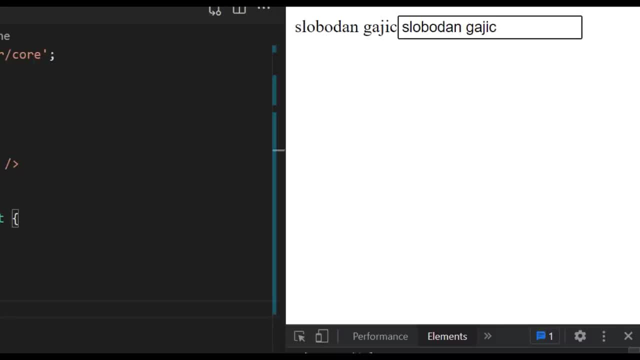 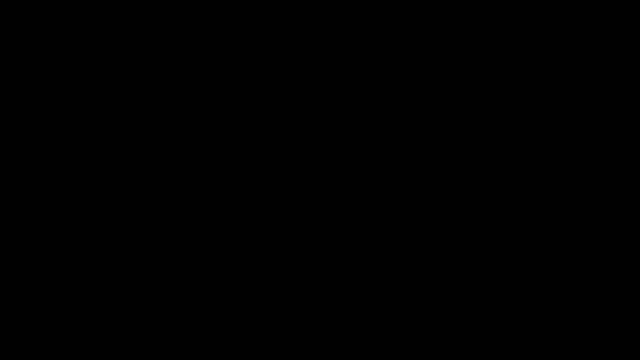 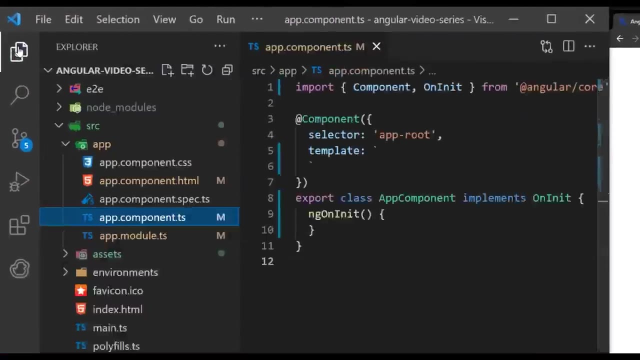 component. you don't need a value, actually, You just need to define the value of the component. And that's all for this section. In this section, we are continuing with Angular directives. Let's build attribute directive. Let's create a file: highlight dot. 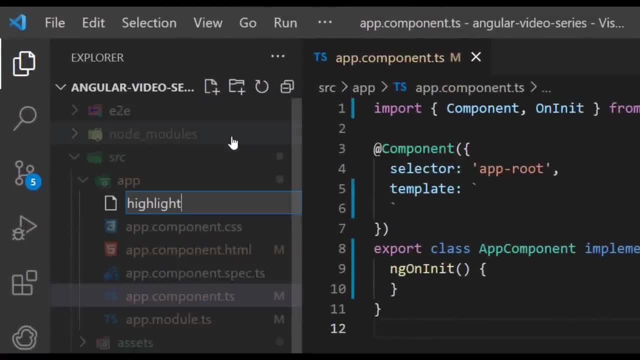 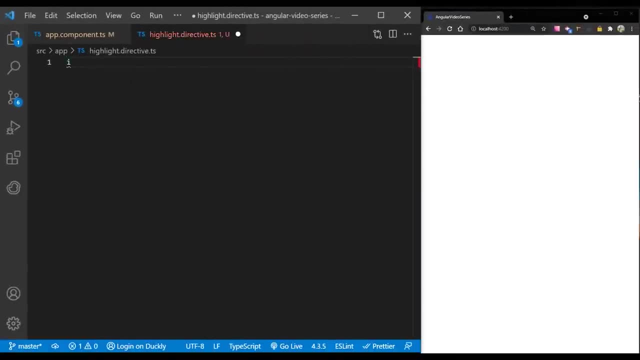 directive dot. yes, which is the convention that you always should follow. Next, import directive decorator from core and implement that decorator with selector property. For me, it's going to be app highlight. Next, we want to export our class And the last thing we want is to import that in our declarations array in app module. 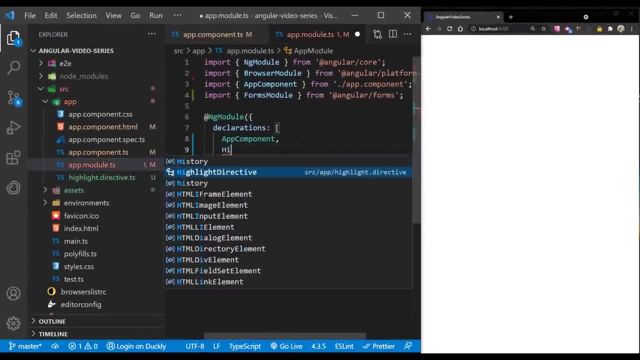 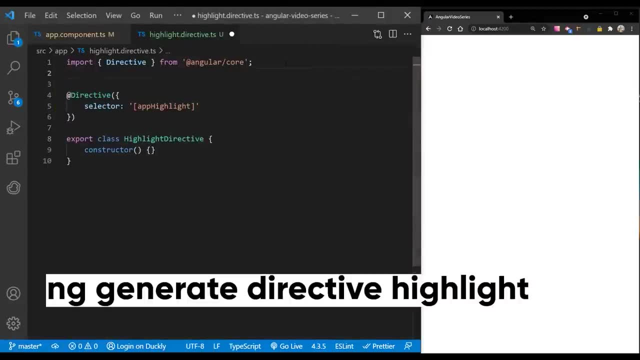 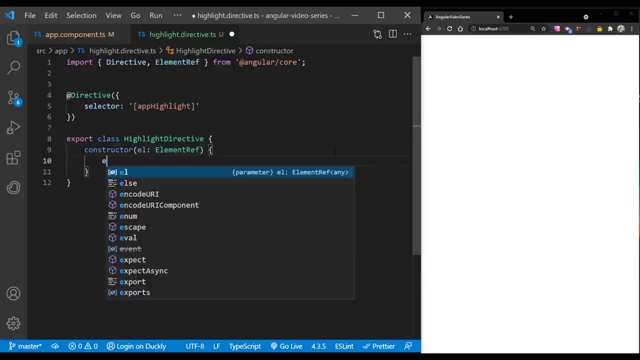 That's our directive boilerplate code, which you can also get with the command ng generate directive highlight: Import element ref from Angular core. element ref grants direct access to the host DOM element through its native element property And element ref in the directives constructor to inject a reference to host DOM element, the element to which you apply. 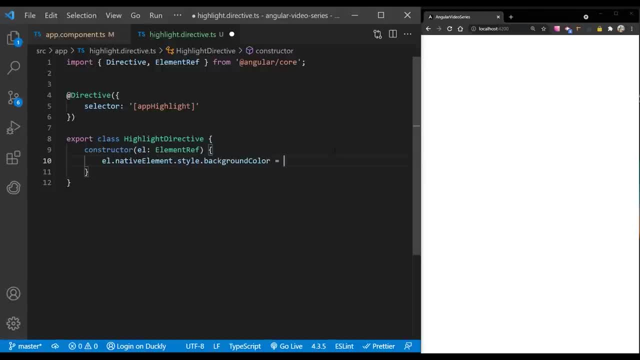 app highlight: Add logic to the highlight directive class that sets the background to yellow. To use the highlight directive, add a paragraph element to the HTML template with the directive as an attribute. Angular creates an instance of highlight directive class and injects in reference to the paragraph. 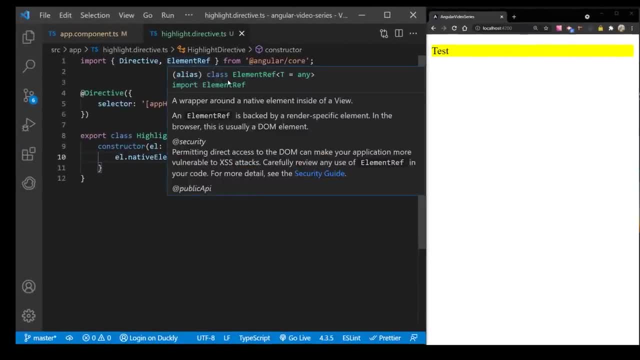 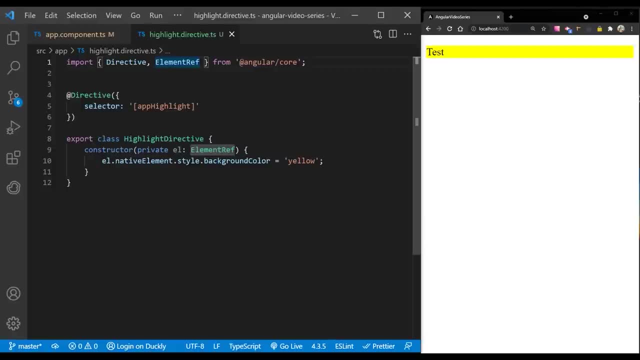 element into directives constructor, which has the P elements background style to yellow. Now let's see how to detect when a user mouses into or out of the element and to respond by setting or clearing the highlight color. Import host listener from Angular core. Add two event handlers that respond. 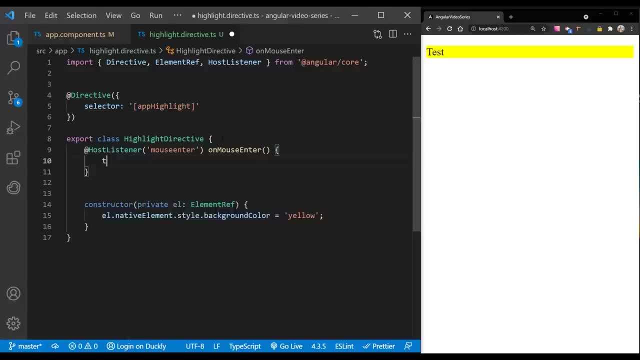 when the mouse enters or leaves each with the host listener decorator. With the host listener decorator you can subscribe to events of the DOM element that hosts and attribute directive. the paragraph in this case, The handlers delegate to a helper method highlight that sets the color on the host DOM element l. 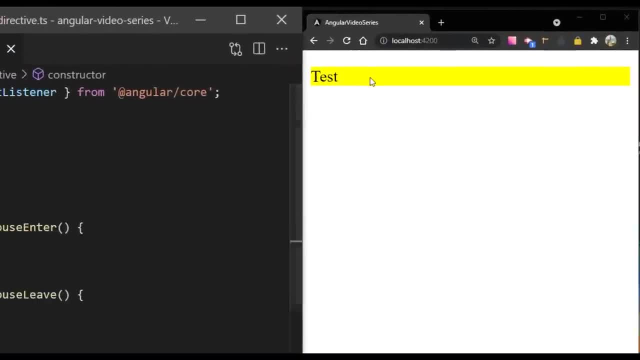 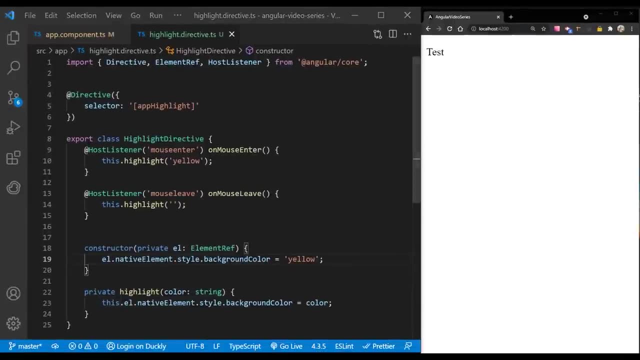 The background color appears when the pointer hovers over the paragraph element and disappears as the pointer moves out. Now let's see how we can make the directive dynamic to be able to use it at different places. For example, let's say that the pointer moves out of the paragraph element. 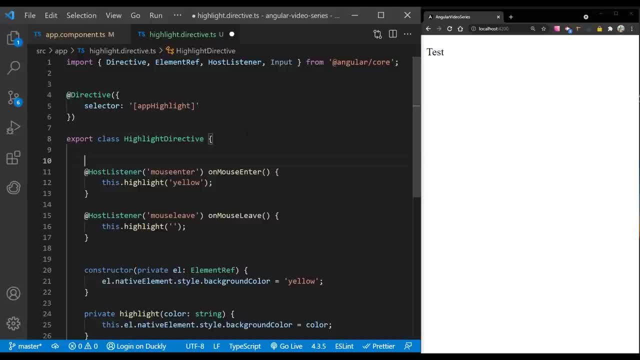 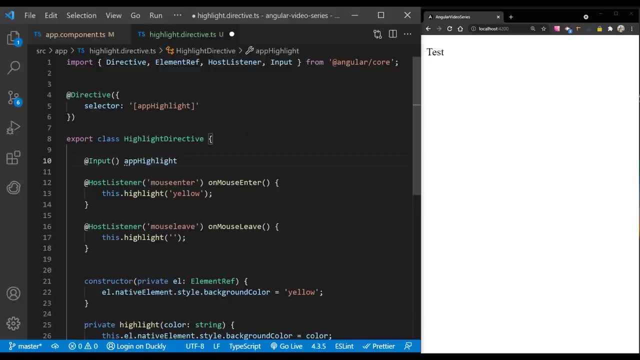 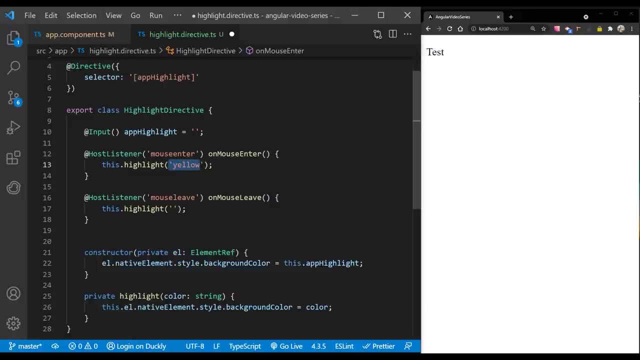 In the end we need to highlight the various types of input properties that we have added In highlight directive ts file import. input from Angular core: add an app highlight input property. the input decorator adds metadata to the class that makes the directive app highlight property available for binding. In app component he has add a color. 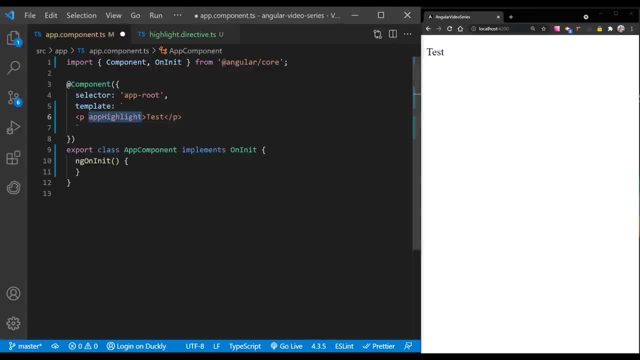 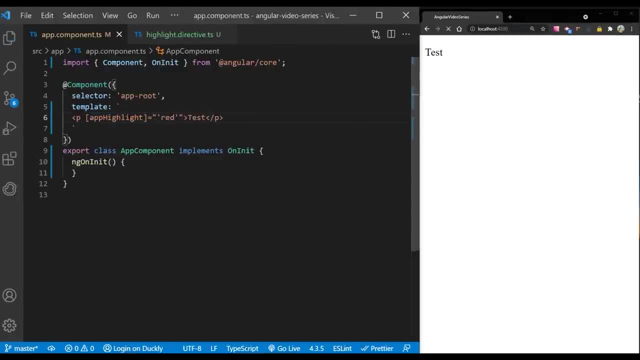 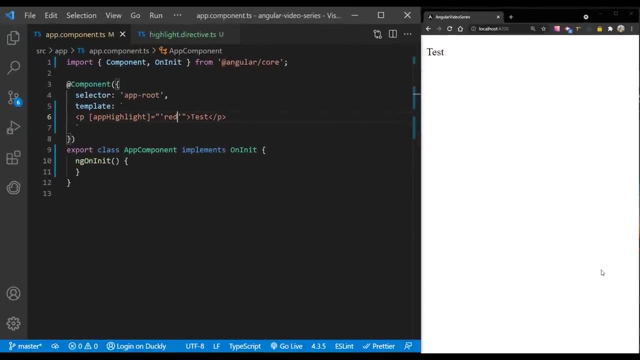 property to the app component To simultaneously apply the directive and the color use the property binding with the app highlight directive selector setting to equal to color. The app highlight attribute binding performs two tasks: applies the highlighting directive to the paragraph element and sets directive highlight color with the property binding, And that's all for this one. 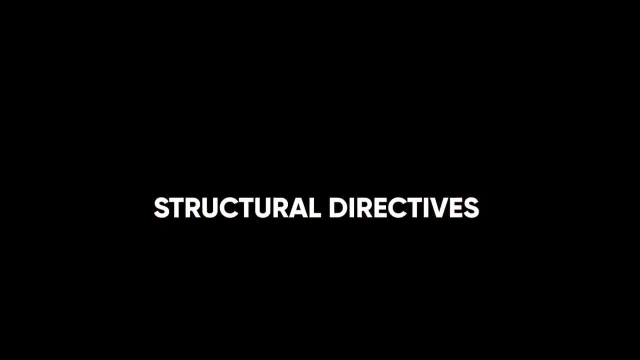 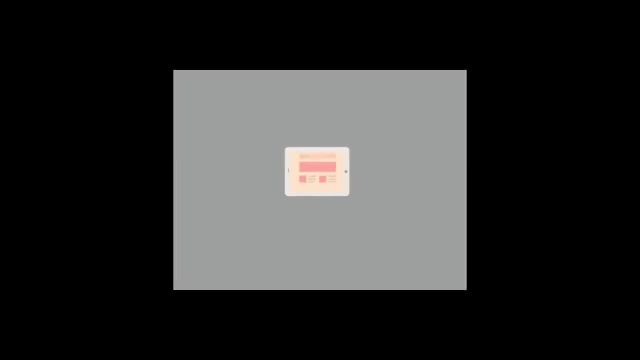 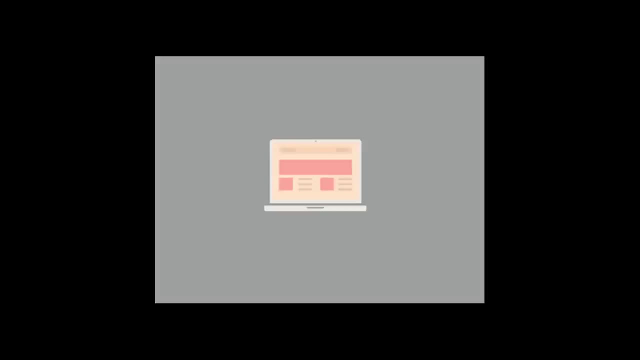 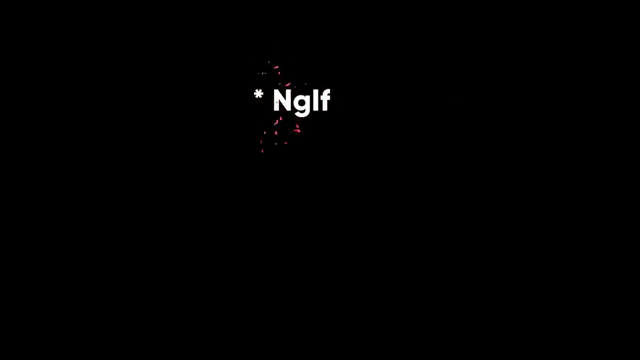 This is the last section about directives, So let's see what are structural directives. Structural directives are responsible for HTML layout. they shape or reshape the DOM structure, typically by adding, removing and manipulating the host elements to which they are attached. This section introduces the most common built in structural directives: ng if conditionally. 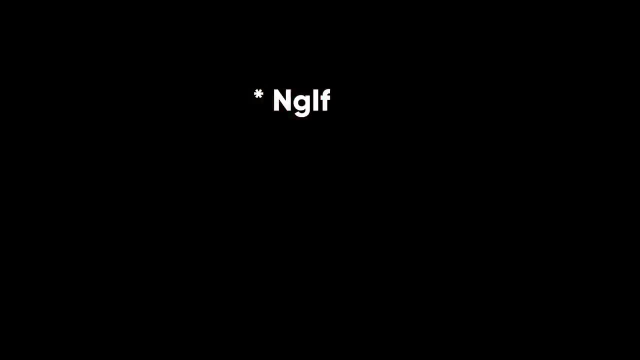 creates or disposes of sub use from the template ng for repeat a node for each item in a list ng switch, a set of directives that switch among alternative views. You can add or remove an element by applying an ng if directive to a host element. When ng if is false, Angular removes an. 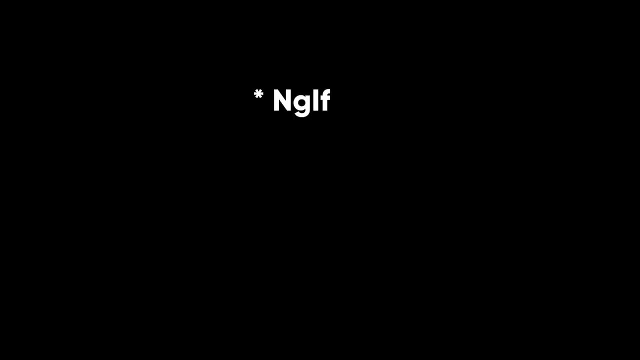 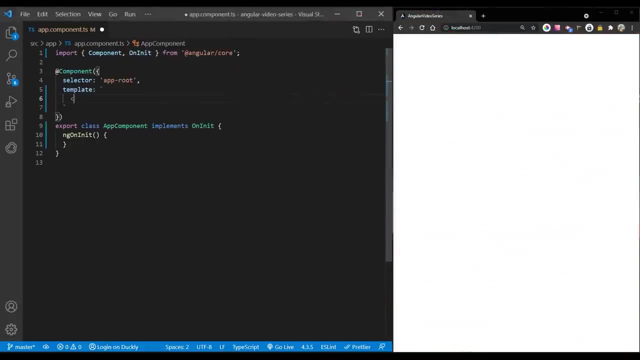 element and its descendants from the DOM Angular then disposes of their components, which frees up memory and resources To add or remove an element. bind ng if to a condition expression such as is active. in this example, When the is active, expression returns a true value. ng if adds the. 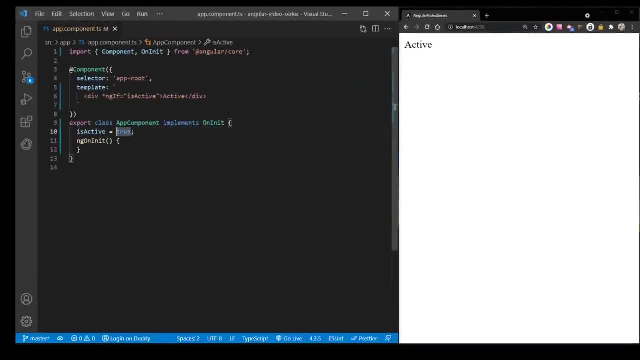 div to the DOM When the expression is false. ng if removes the div from the DOM. That's simple. right Now, let's talk about ng, for you can use the ng for directive to present a list of items. Let's create an array of objects with the name. 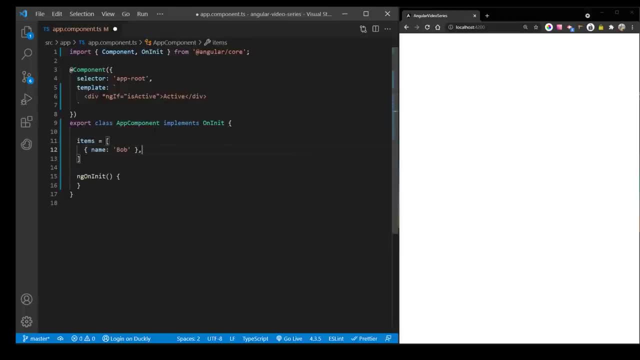 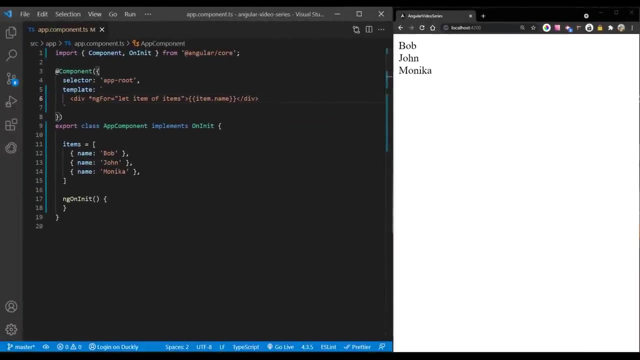 property in it. Define a block of HTML that determines how Angular renders a single item To list your items. assign the shorthand let item of items to ng for the string let item of items instructs Angular to do the following: Store each item in the items array in the local item looping variable. 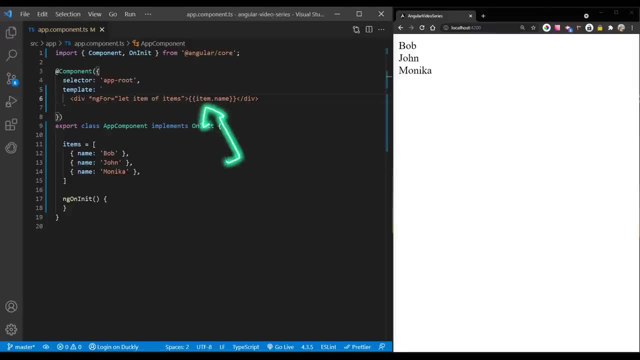 Make each item available to the template. HTML for each iteration Translate. let item of items into ng template around the host element. Repeat the ng template for each item in the list. By the way, you can get the index of ng for in a template input variable and use it in the template. 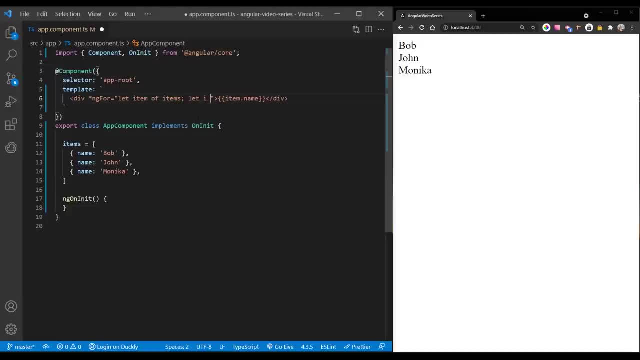 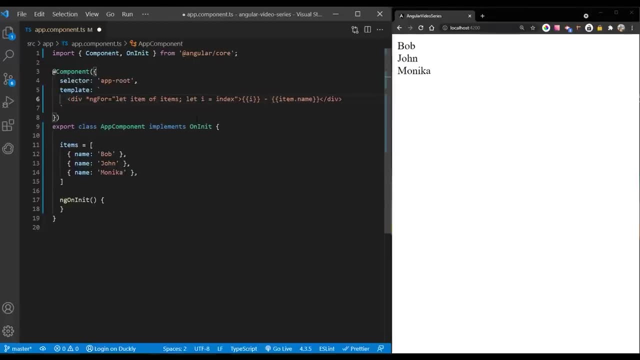 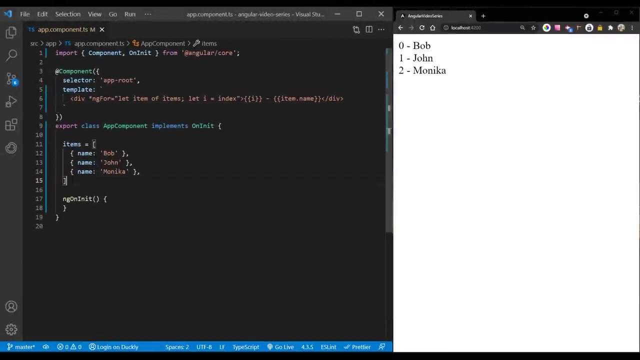 In the ng for add a semicolon and let i equals to index, to the shorthand. The following example: gets the index in a variable named i and displays it within the item name. And the last directive which we are going to talk about is switch, Like the JavaScript switch. 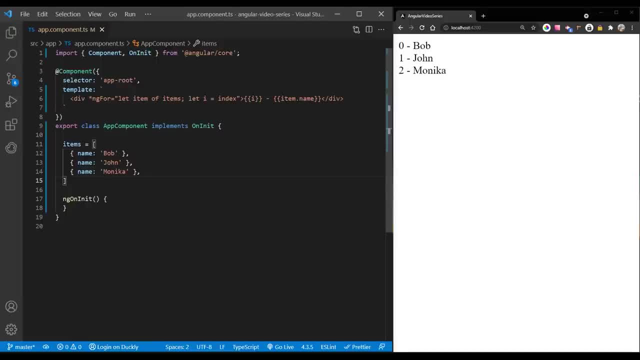 statement and just switch displays one element from among several possible elements Based on a switch condition. Angular puts only the selected element into the DOM. ng switch is a set of three directives. ng switch, an attribute directive that changes the behavior of its companion directives. 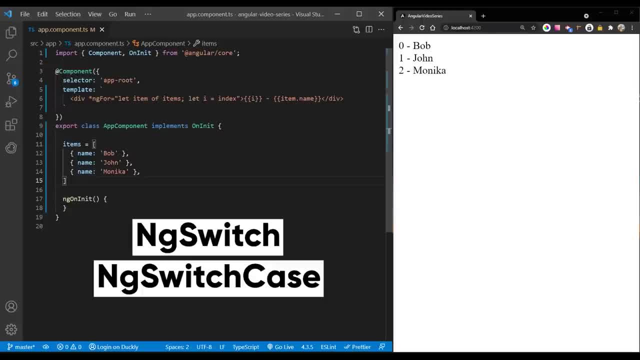 ng switch case- structural directive that adds its element to the DOM when its bound value equals to switch value and removes its bound value when it doesn't equal the switch value. ng switch default- structural directive that adds its element to the DOM when there is no selected ng switch case. I'll modify the items array to be just a single item. 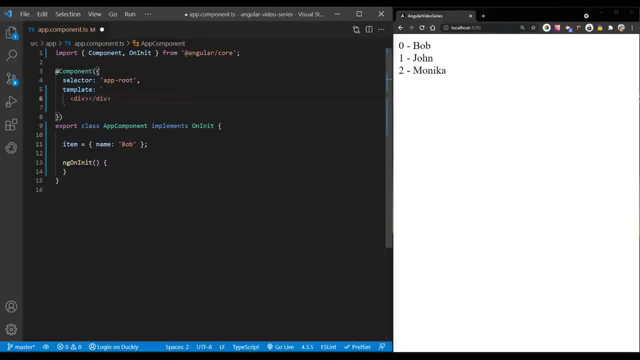 On an element such as a div add ng switch bound to an expression that returns the switch value, such as a name, Though the name value in this example is a string, the switch value can be of any type Bind to ng switch case and ng switch default on the elements for the cases. 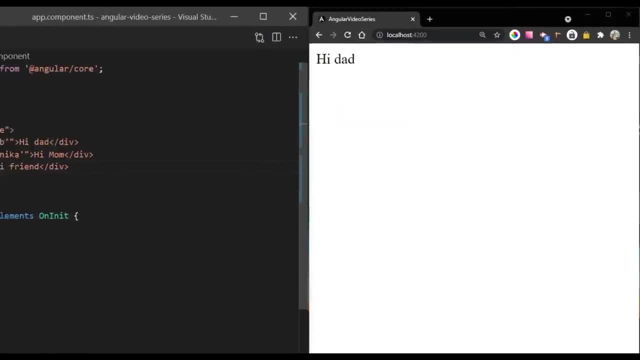 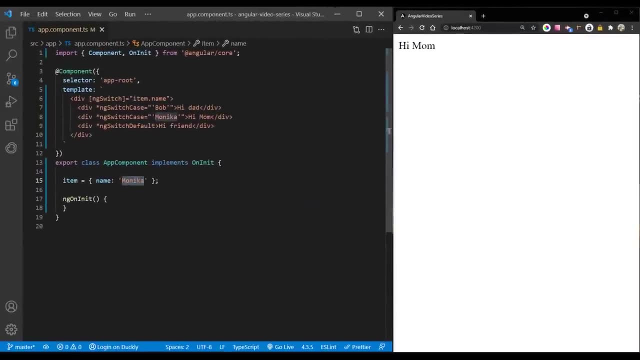 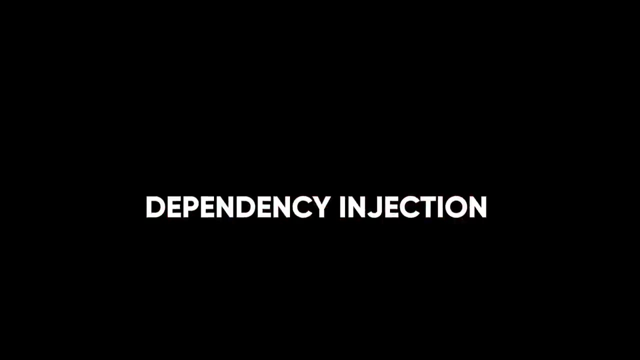 And now, depending on the value of the item, name rendering or the page changes. If it didn't provide a case for the name value, default will be executed. Next we are discussing dependency injection. Dependencies are services or objects that a class needs to perform its function. 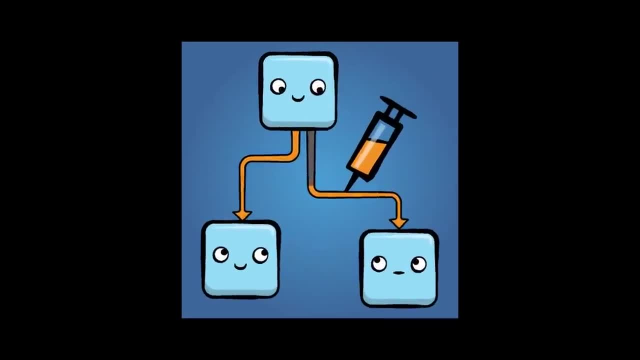 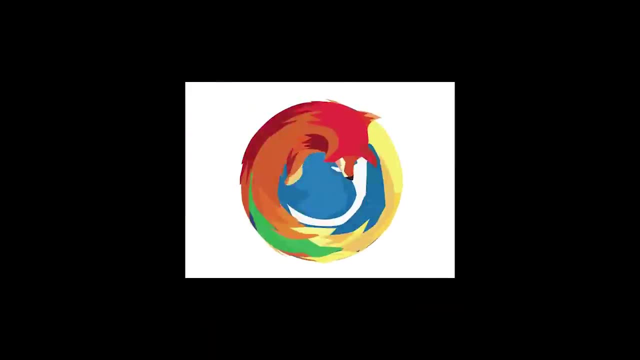 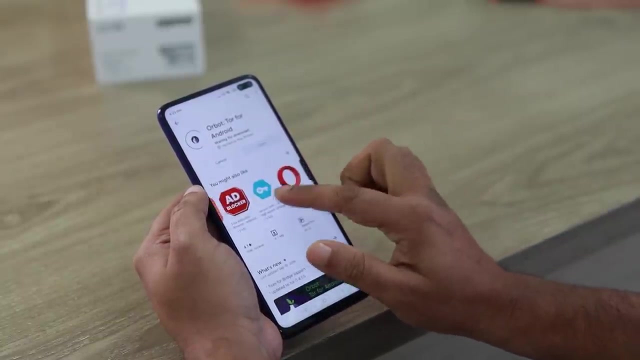 Dependency injection, or DI, is a design pattern in which a class requests dependencies from external sources rather than creating them. You can look at it as if you are adding an extension to your browser or adding an app to your phone. Once you add it, you provide yourself with new functionalities and features. 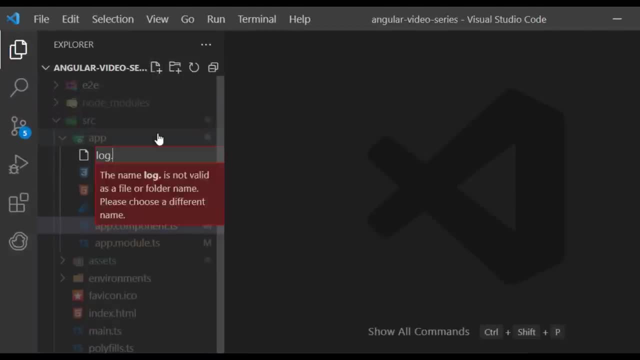 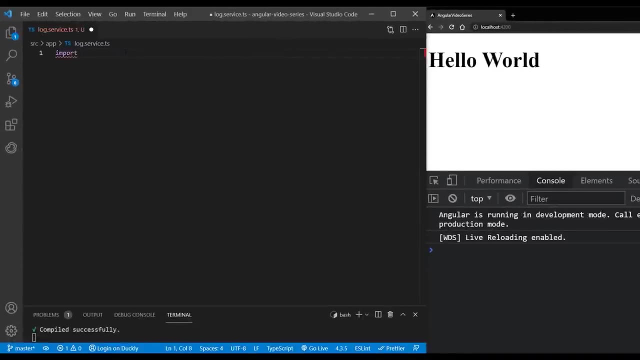 Let's create a service which we can inject in our components. Create a new file with the name logservicets- Import injectable decorator from Angular core and then add a classic pass and then, for provided in metadata, add root value. 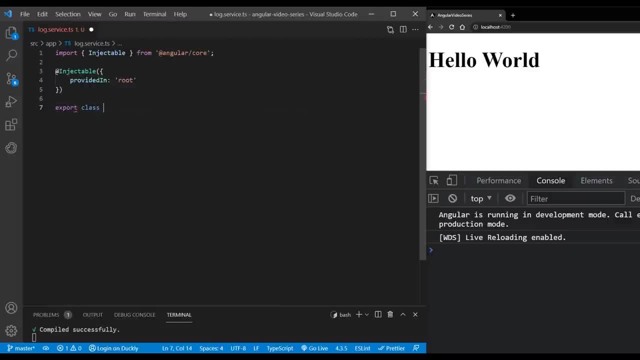 Which means that we are going to provide the service in the root of the application and that it is visible throughout the application. Export our log service class and inside of this service we want to add our logMessage method, which will just log past messages. 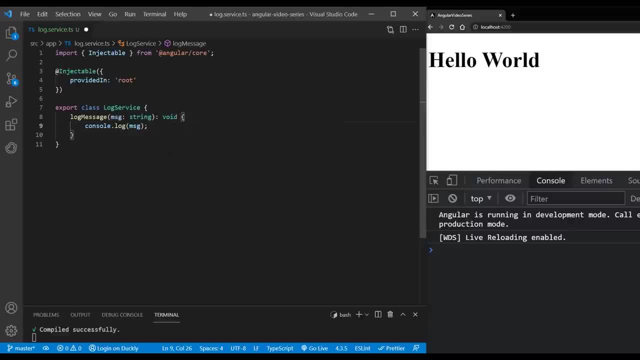 And then add a pass method which will just add past messages. For clarity and metadata. let's create a service that will provide, in the root of the application, clarity and maintainability. it is recommended that you define components and services in separate files. Now inject our log service into the app module file in providers array Injecting service. 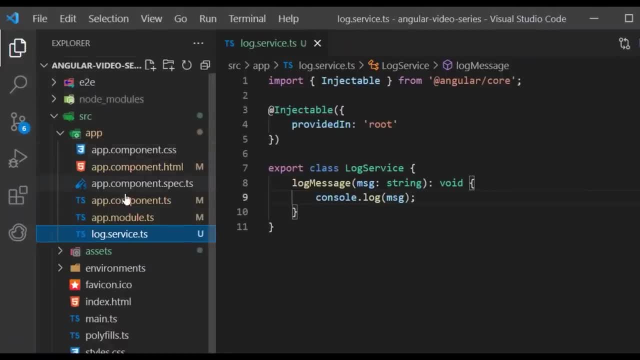 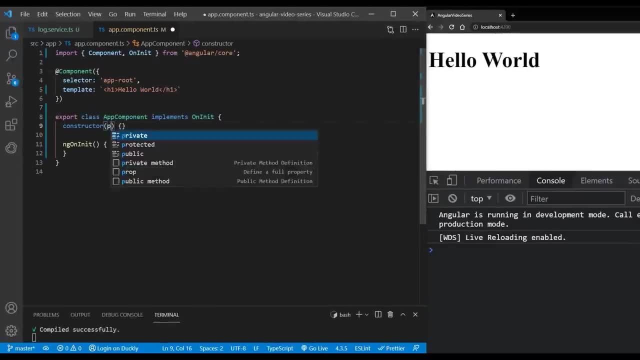 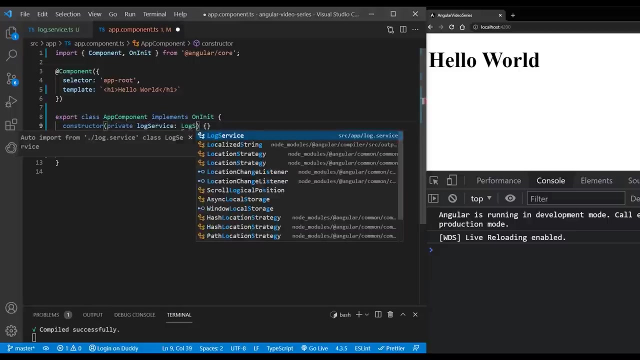 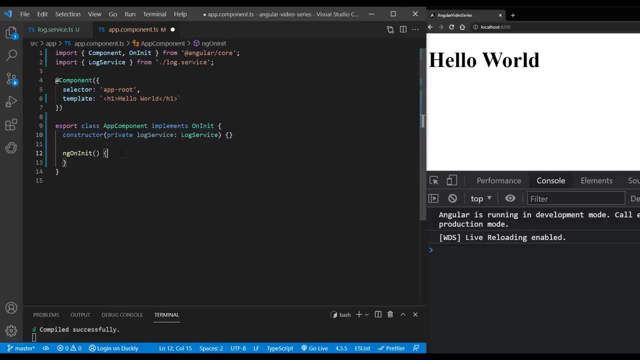 results in making them visible to a component. To inject a dependency in components constructor supply, a constructor argument with dependency type. The following example specifies the log service, the app component constructor. the type of log service is log service. Now we can reference our log service in our component and call our method from it. 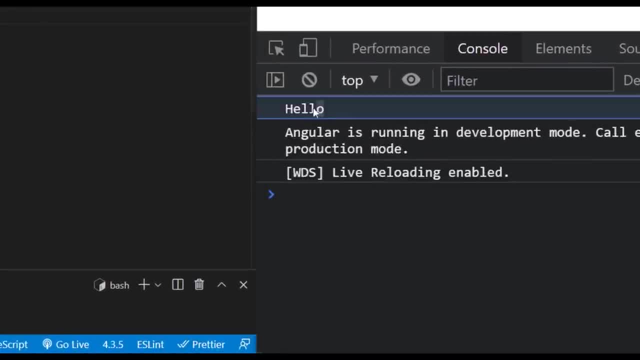 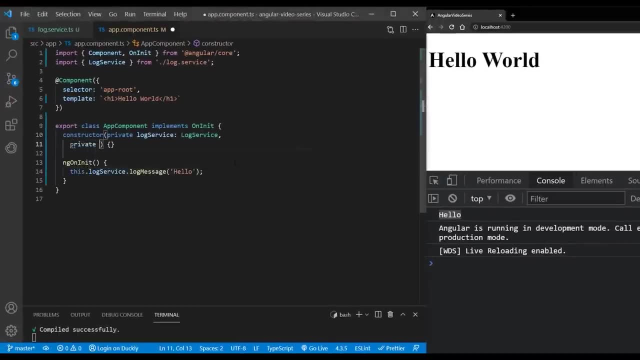 We should pass our message And, as you can see, it's being executed as expected. we can use this approach to inject third party libraries and other modules that are used in the app component constructor. So let's inject render to module which is used for custom rendering and updating the DOM import. 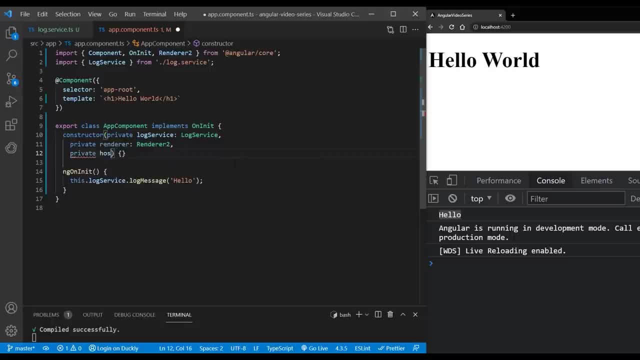 renderer to from Angular core and inject it inside the constructor. Also, we will need element ref which we can use for referencing our DOM elements or the host component. in our case Now inside the ng on init lifecycle, called the set style method of the renderer and set the color of host native. 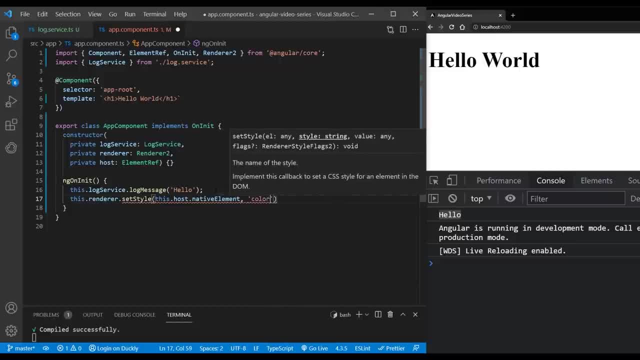 element And we can also use the renderer as a reference for the host component in our case, and we can also use the renderer as a reference for the host native element. to read: This method changes the color of our components text And, as you can see, 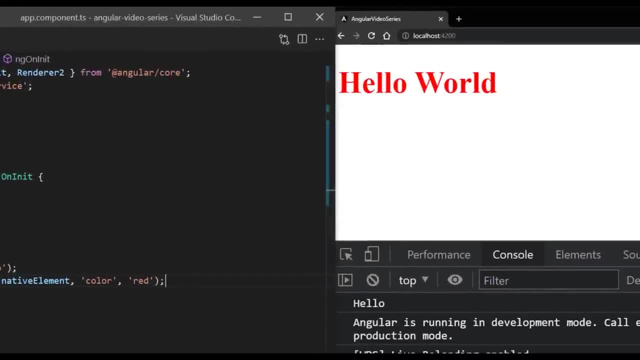 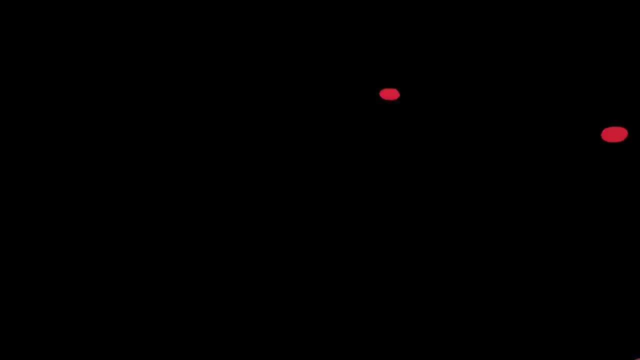 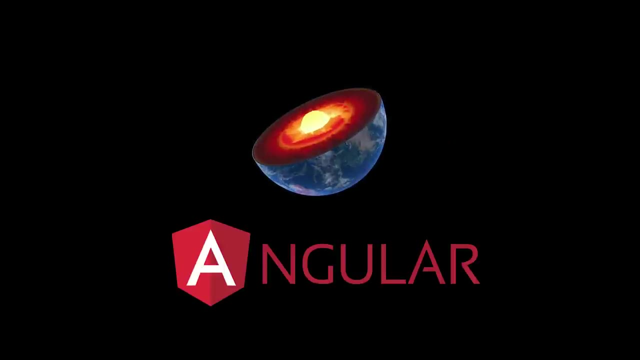 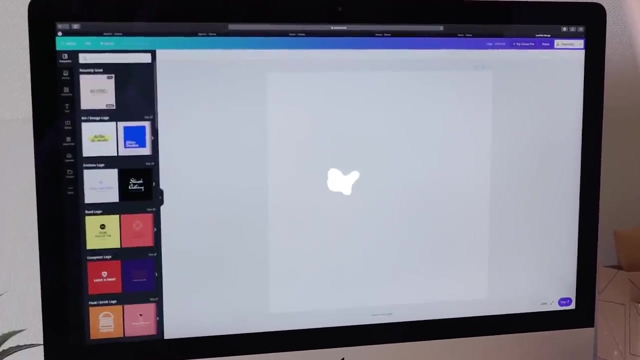 with the dependency injection, we get access to more features and methods. That's all there is to it. Next is very important topic: routing. The Angular router is a core part of Angular platform. It enables developers to build single page applications with multiple views and allow navigation between these views. We can compare routing of our 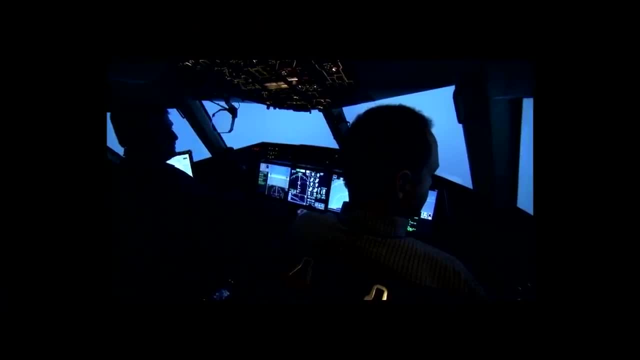 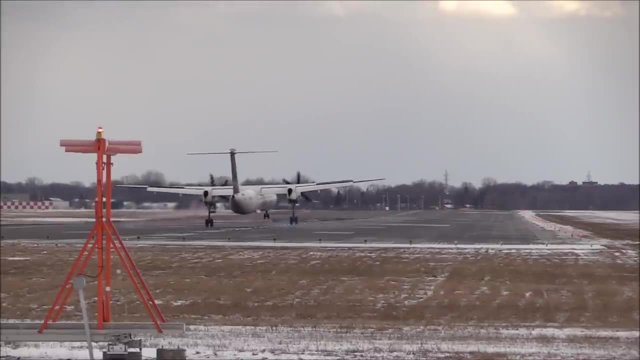 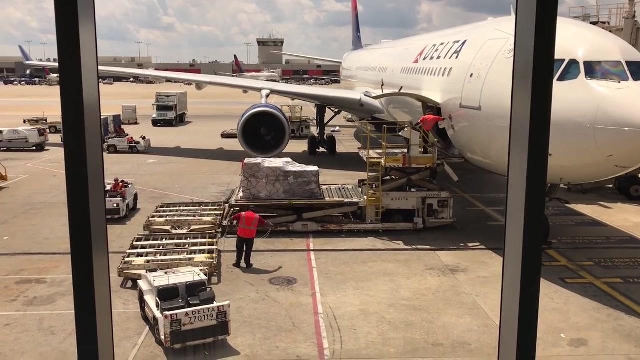 applications with navigating a plane. Pilot sets the flight coordinates- in our case route path- and the plane lands on the desired location or desired page in our app. Oftentimes, planes carries goods or cargo and routes carry per arms info and data. 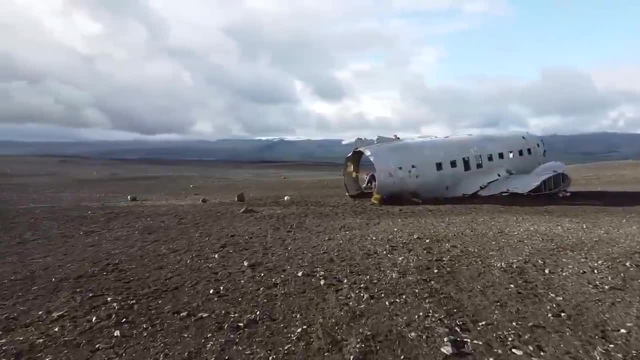 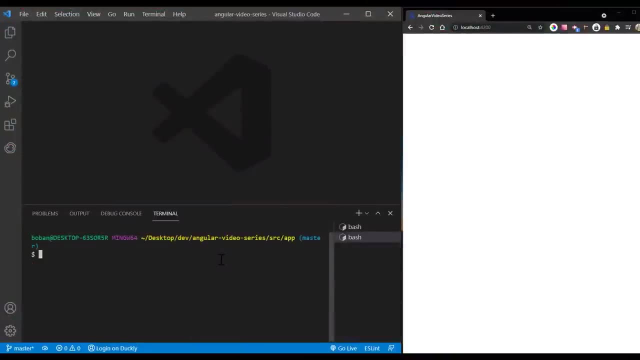 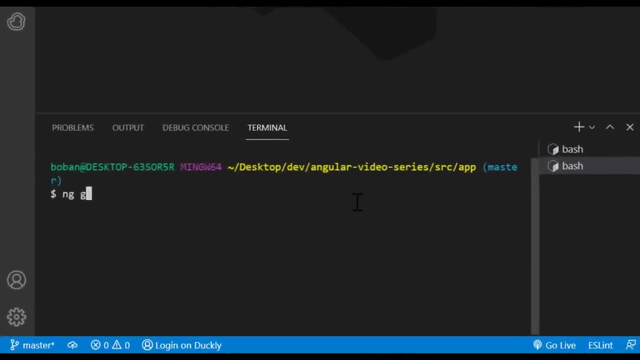 And unfortunately some planes do get crashed or lost And for all. sometimes we get a lot of data times. we get 404.. To use the Angular router, an application needs to have at least two components so that it can navigate from one to other. To create a component using the CLI, enter the 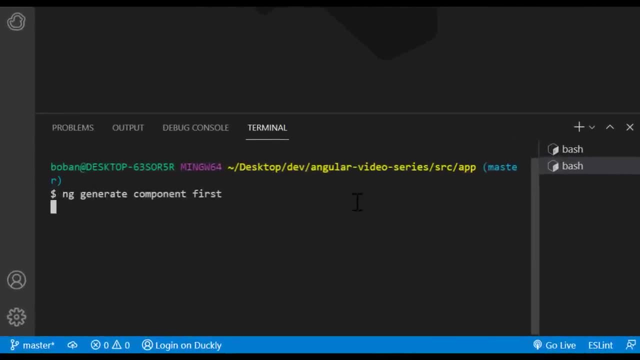 following at the command line, where first is the name of your component: ng generate component. first. Repeat this step for a second component, but give it a different name. Here the new name is second. This guide works with a CLI generated Angular application. If you are working manually, 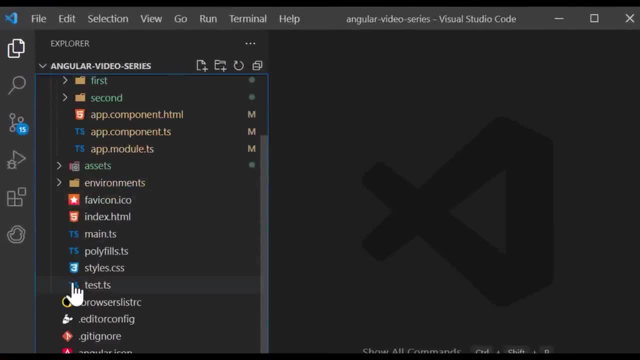 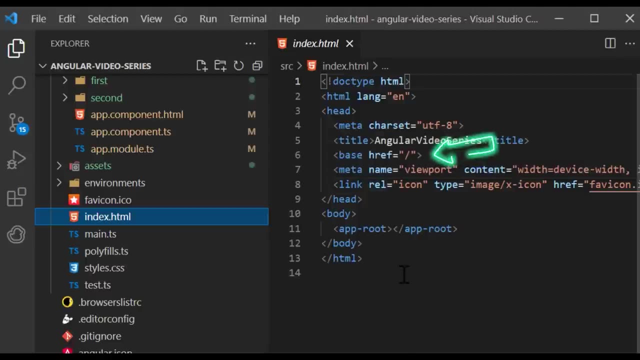 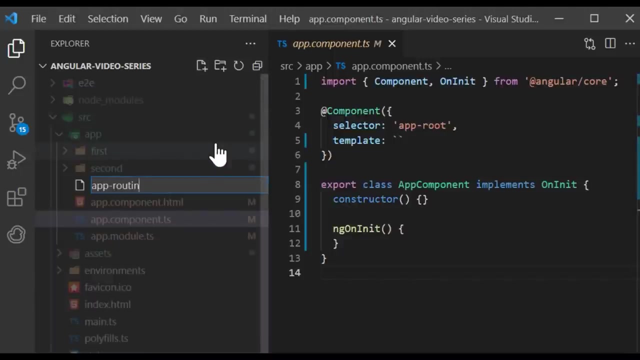 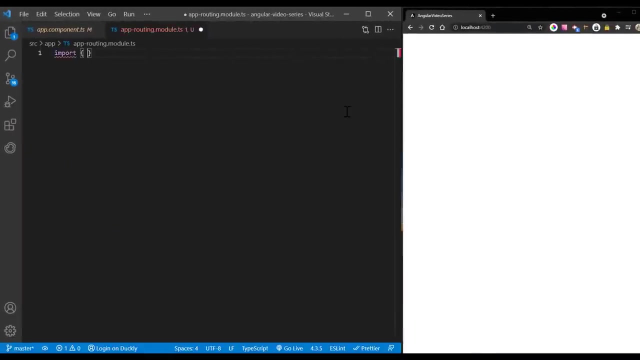 make sure that you have base href with slash in the head of your index HTML file. This assumes that the app folder is the application route and that uses slash. create a new module for routing. name it: app dash routing dot module. Define const routes, which is type of routes. Here we will define our paths and components. 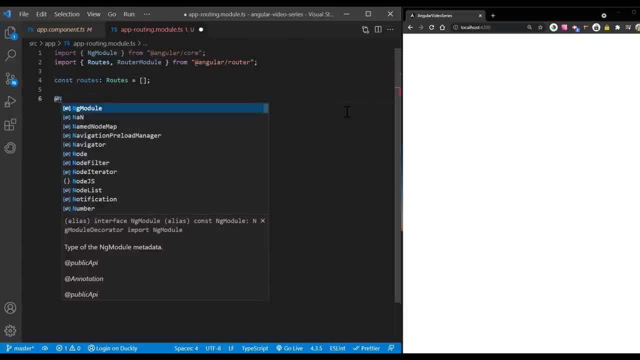 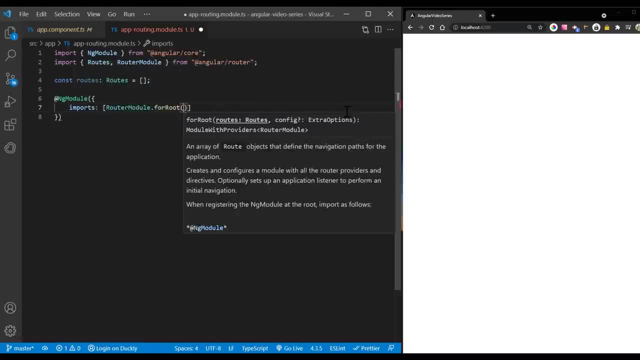 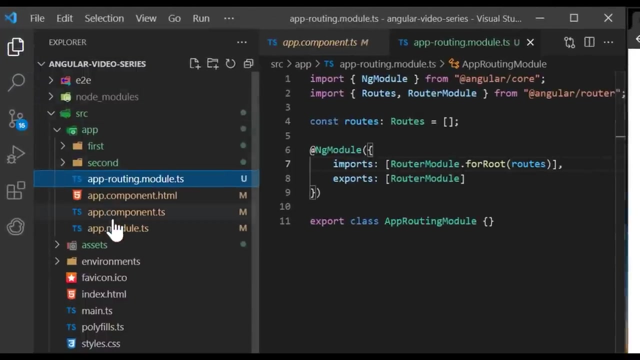 Inside ng module imports array. add router module and call for root module with routes passed as argument. Then export your router module so it can be imported into the root module At the end. define the app routing module class. Import the app routing module into app module and add it to the imports array. 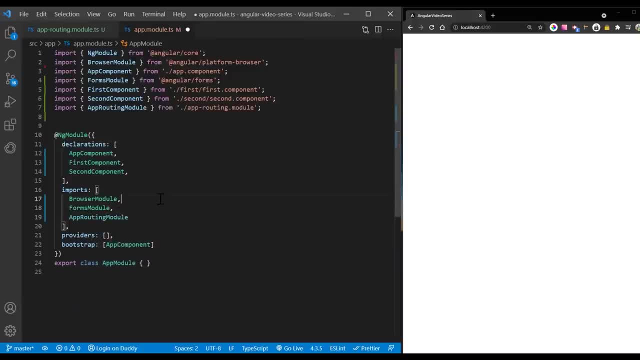 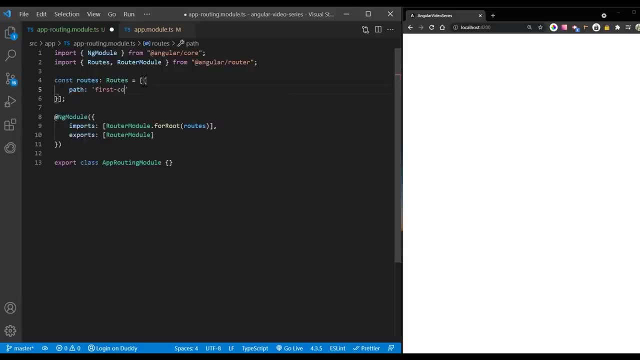 Now define your routes in your routes array. Each route in this array is a JavaScript object that contains two properties: The first property path defines the URL, and the second property path defines the URL, and the third property path defines the URL For the route. the second property component defines the component that Angular should use. 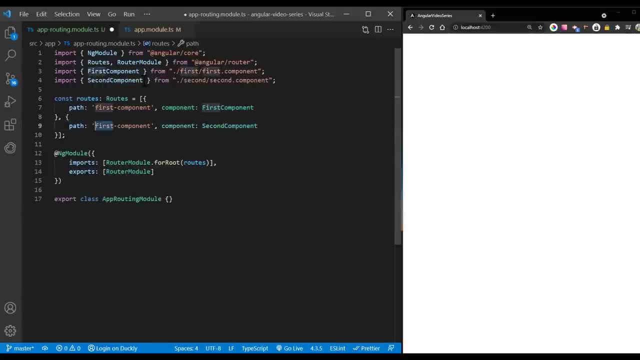 for the corresponding path. Now that you have defined your routes, you can add them to your application. First, add links to the two components. Assign the anchor tag that you want to add the route to the router link attribute. Set the value of the attribute to the component to show when a user clicks on each link. 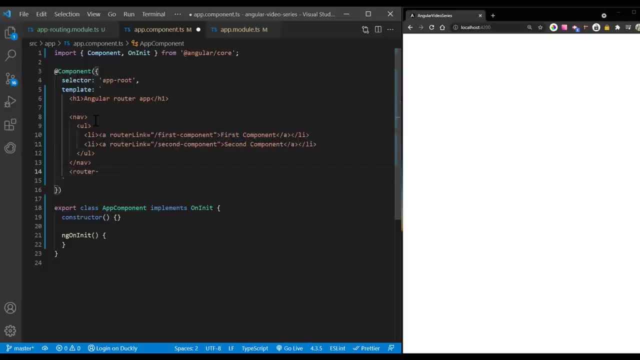 Next, update your component to show when the user clicks on each link. Next, add the clылas class component, for example, the route department template, to include router outlet. This element informs Angular to update the application view with the component for the. 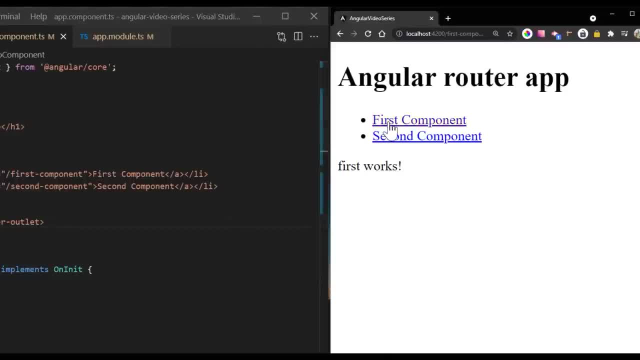 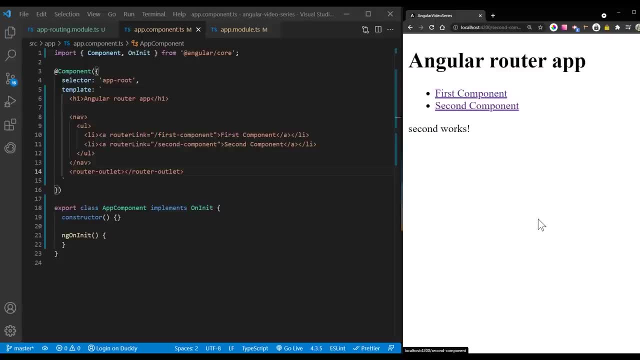 selected route. You can add router link active attribute if you want to style active link. One note: the order of routes is important because the router uses a first match wins strategy when matching routes, So more specific routes should be placed above less specific routes. 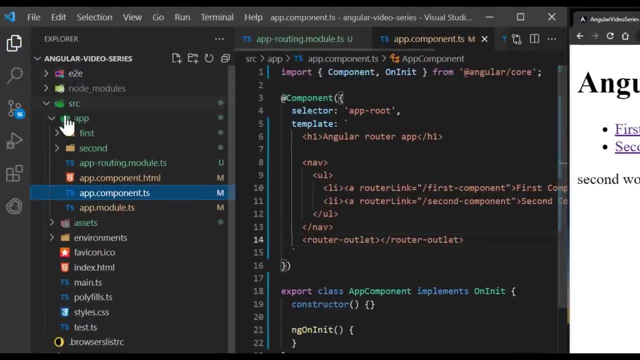 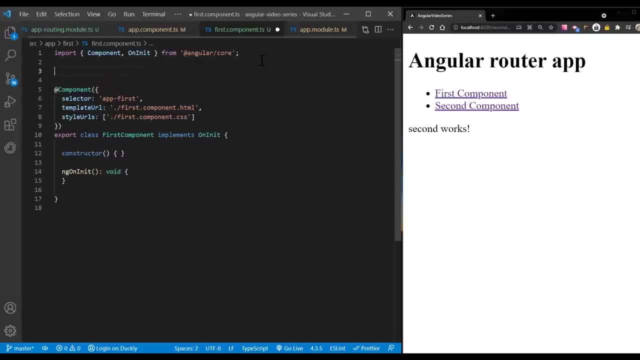 Often, as a user navigates your application, you want to pass information from one component to another. To do so, you use the activated route interface. First, import router, activated route and parameter map to your component. Inject an instance of activated route by adding it to your applications constructor. 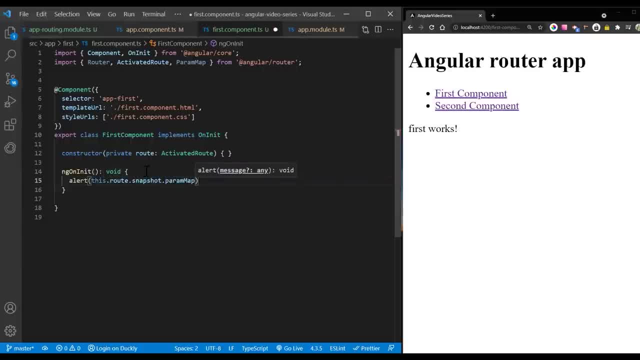 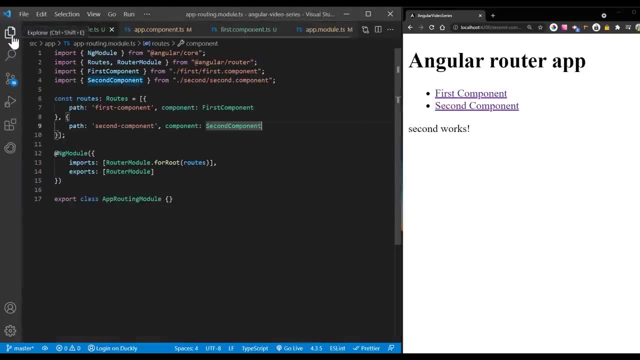 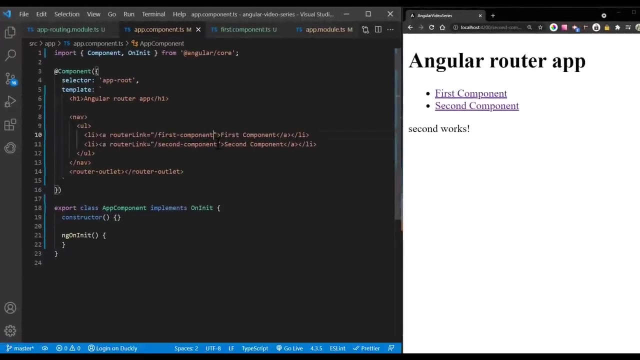 Apply the ngOnInit method to access the activated route and track the ID parameter. Now we need to adjust our routes to pass the ID param as well. In path add semicolon and name of your parameter, And then we can add ID values to our links. 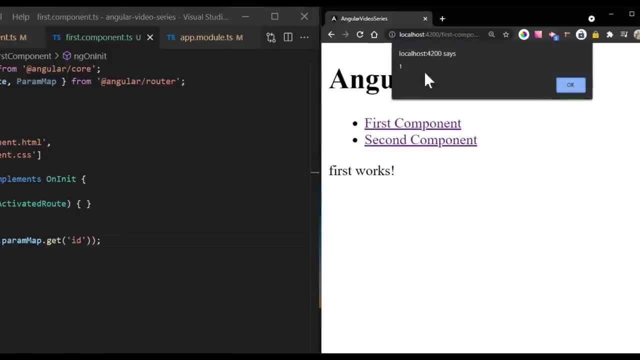 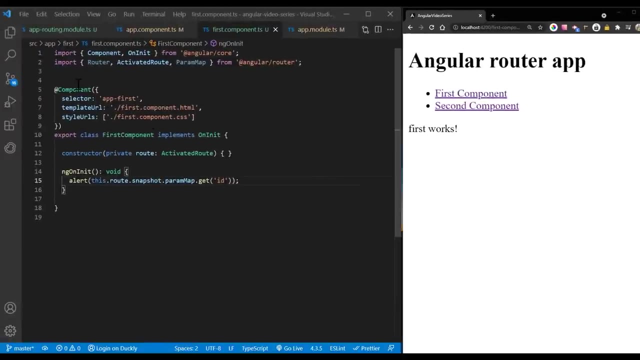 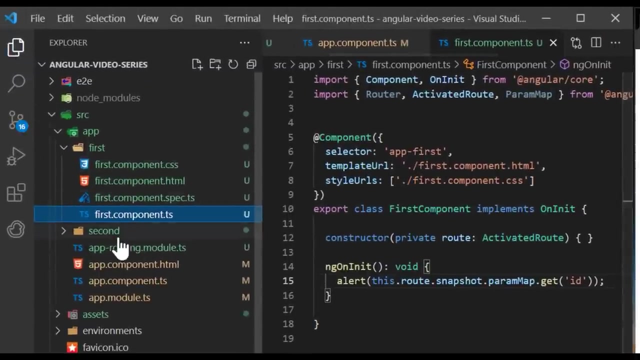 That's how you pass and retrieve data from one component to another. A well functioning application should gracefully handle when user attempts to navigate to a part of your application that doesn't exist. To add this functionality to your application, you set up a wildcard route. 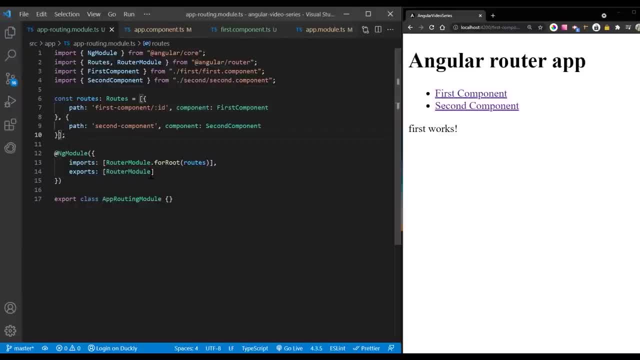 The Angular route selects this route anytime the requested URL doesn't match any router paths. To set up a wildcard route, Add the following code to your routes definition For the component property: you can define any component in your application. Common choices include an application specific page: not found component. 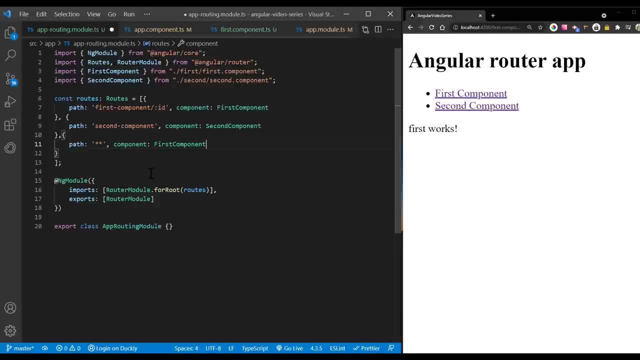 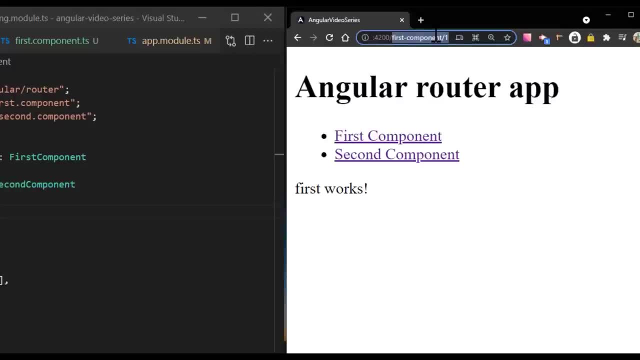 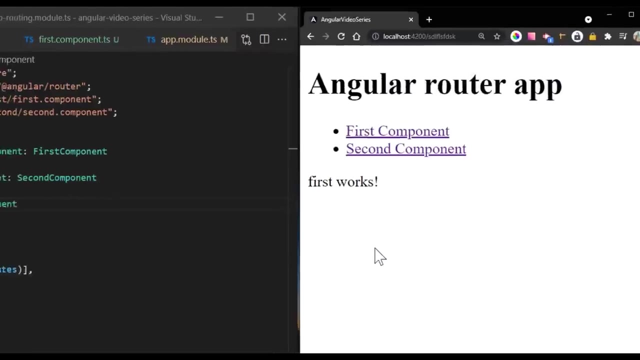 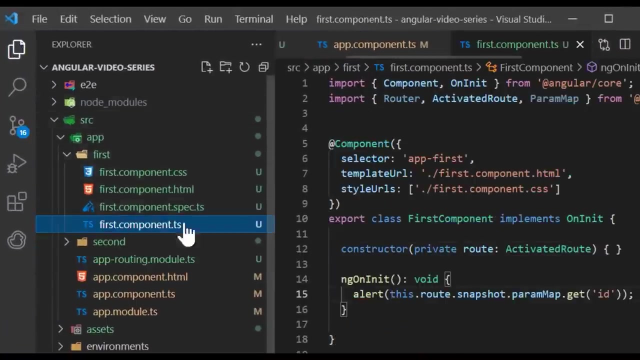 But here I'm just redirecting to the first component. And now if you navigate to any random path, it will always give us first component. As your application grows more complex, you may want to create routes that are relative to the component other than your route component. 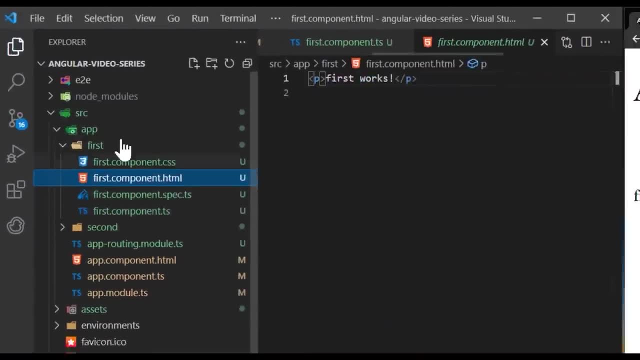 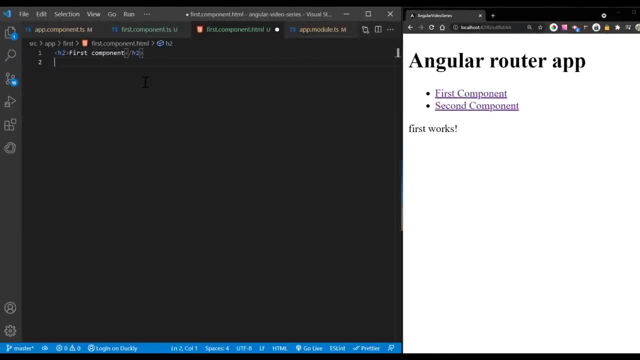 These types of nested routes are called child routes. This means you're adding a second router outlet to your app, because it is in addition to the router outlet in app component. In this example there are two additional child components, child A and child B. Here 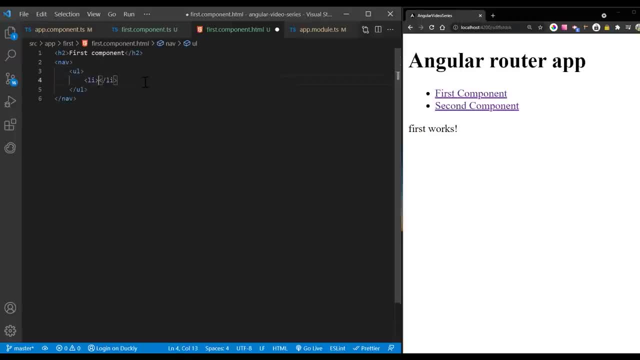 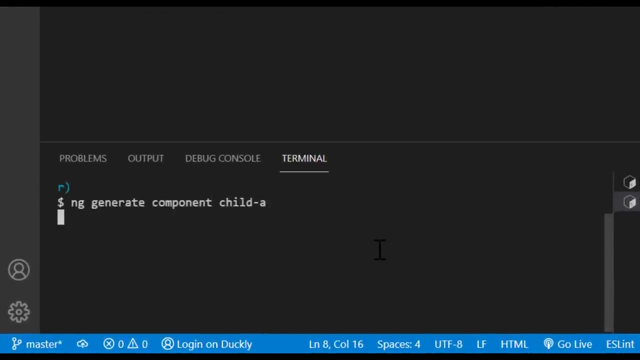 first component has its own nav And a second router outlet in addition to the one in app component. Also, I'm going to create two child routes with the router links of child A and child B And give it a second router link. Now I'll create two additional component with Angular CLI and name their child a component. 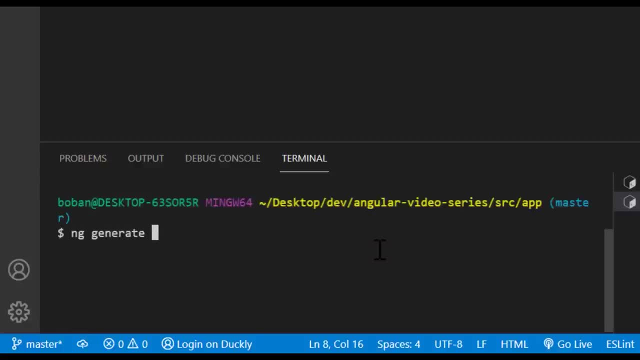 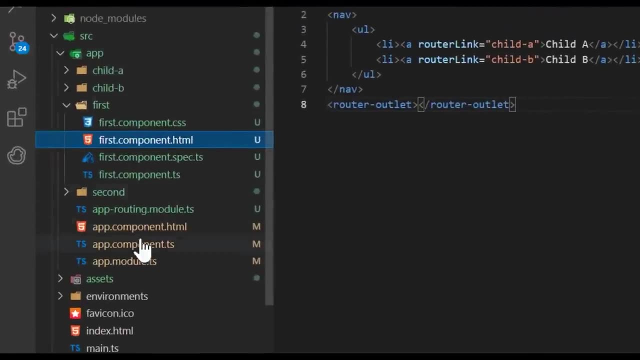 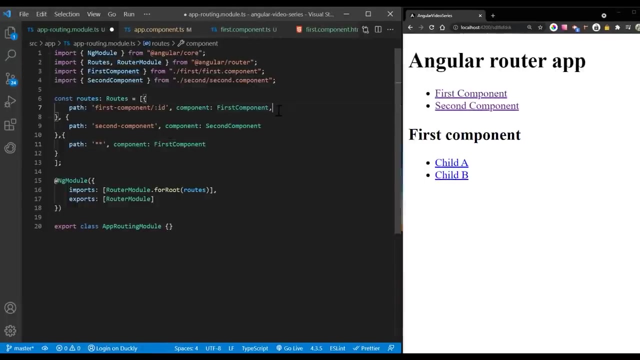 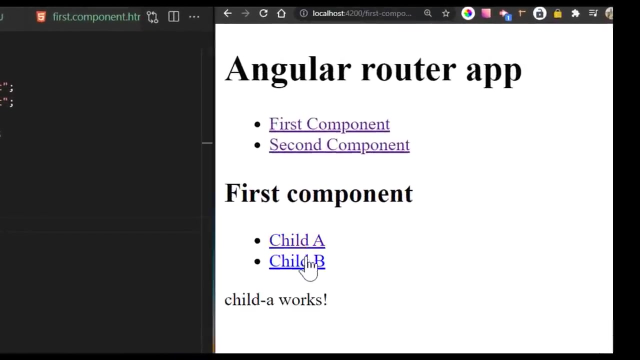 A child route is like any other route in that it needs both a path and a component. The one difference is that you place child routes in a children array within the parent layout. Now, if you navigate to any of child routes, we get the corresponding child component. 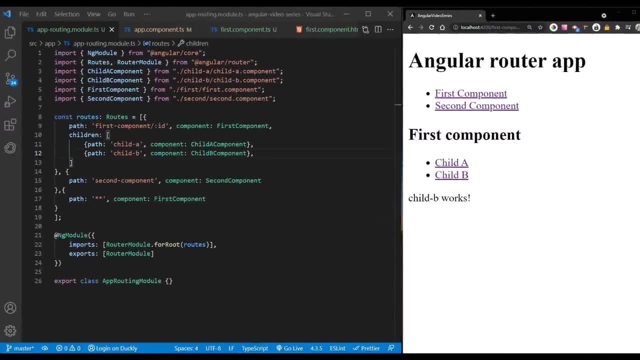 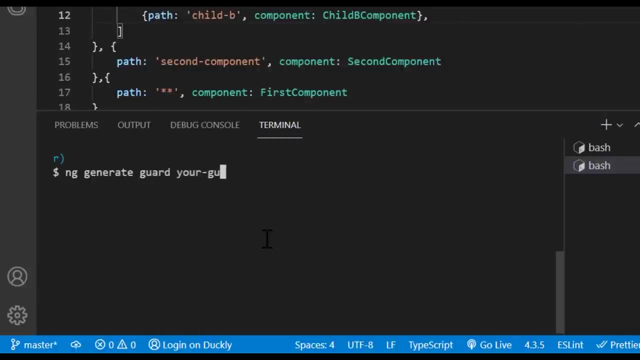 Use route guards to prevent users from navigating to parts of an application without authorization. The following route guards are available in Angular: can activate connect to a child. can deactivate Resolved- Resolved. Scotland. can load. create a service for your guard. angina generate guard your guard. 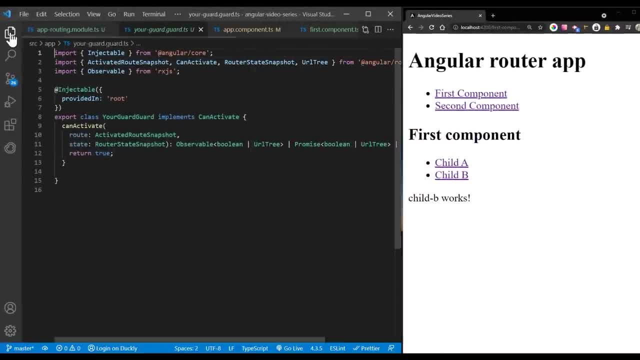 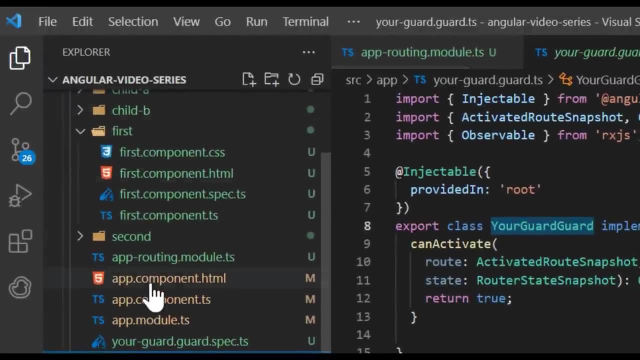 in your guard class, implement the guard you want to use. the following example uses can activate to guard the route. Now, depending on your logic, it can return true or false. Usually it's checks it. The user is logged in or does he have privileges to access the page? In your routing module, use the appropriate property. 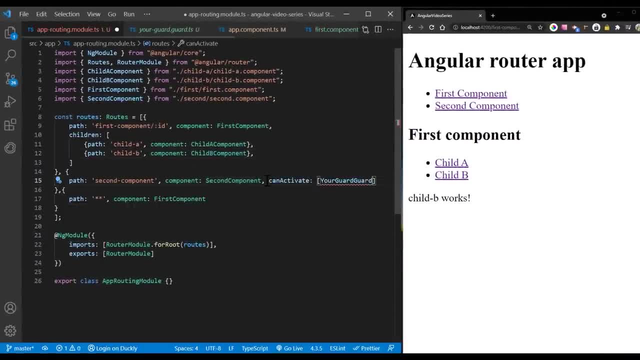 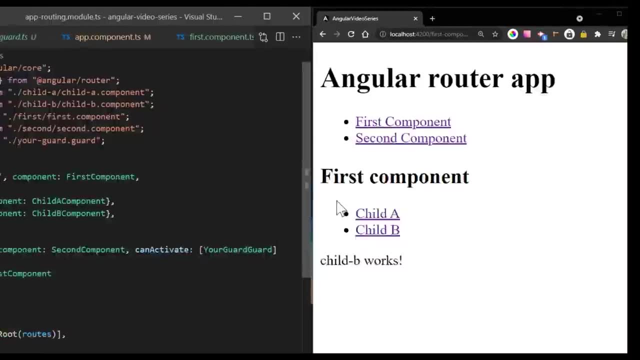 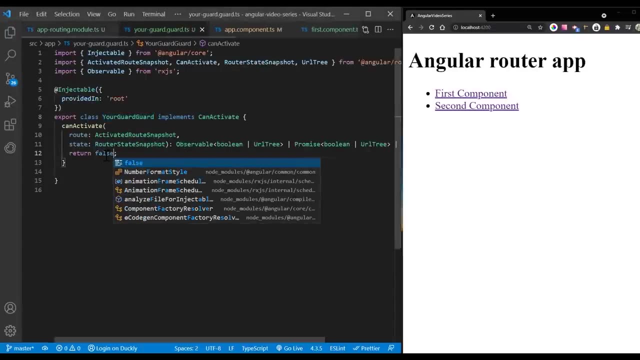 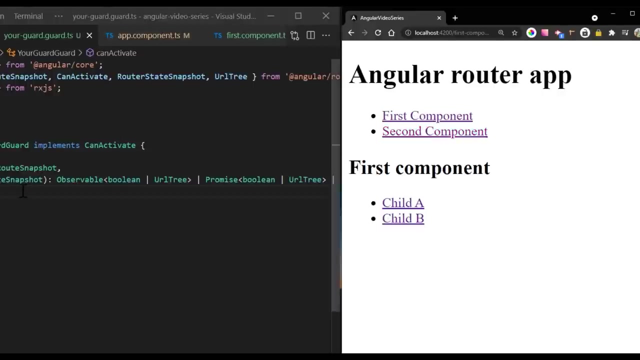 in your routes. configuration here can activate, tells the router to mediate navigation to this particular route. Now we set the guard to false, we can't access the route, Otherwise we can. And that's all for routing for this section. After this one we are covering one even more important concept. 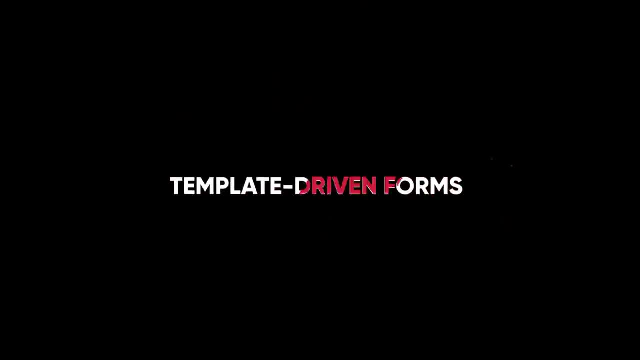 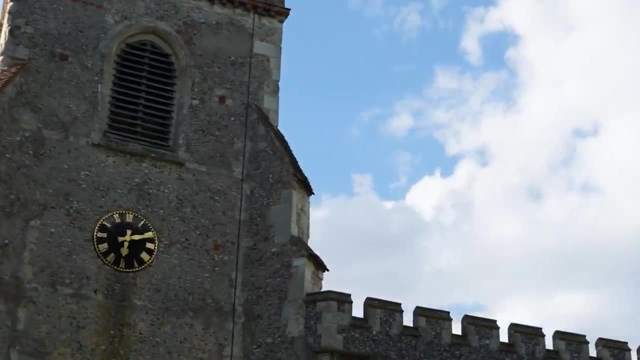 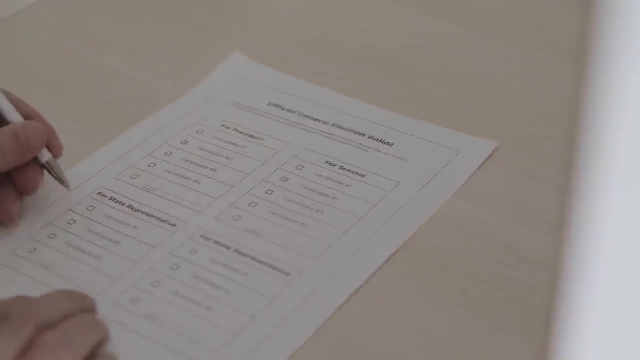 and that is Angular forms. Let's start off with template driven forms. I know it sounds impossible, but there were times when there was no internet or even computer, So in those times we had to fill out good old paper forms when we wanted to visit a doctor. 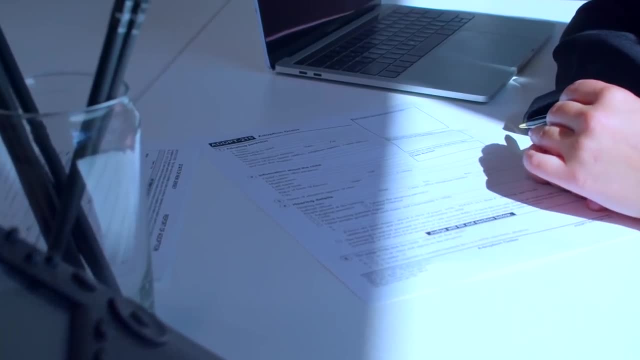 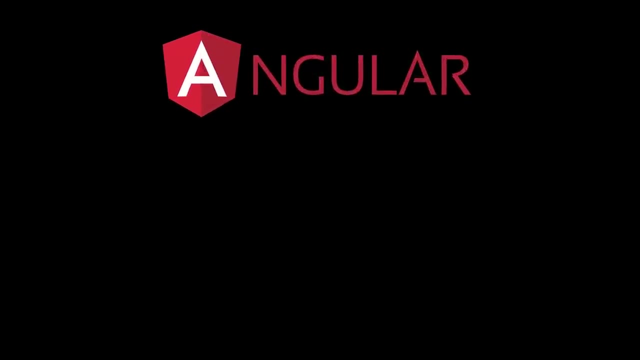 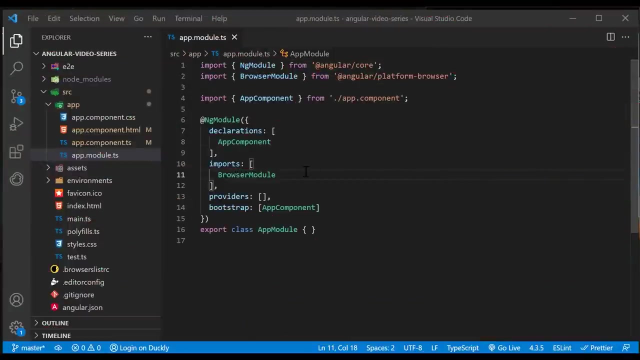 or to apply for various personal documents. So web forms are nothing different, except they're digital Angular supports to design approaches for interactive forms. Template driven forms are suitable for small or simple forms, while reactive forms are more scalable and suitable for complex forms. This tutorial shows you how to build a form from scratch. First, 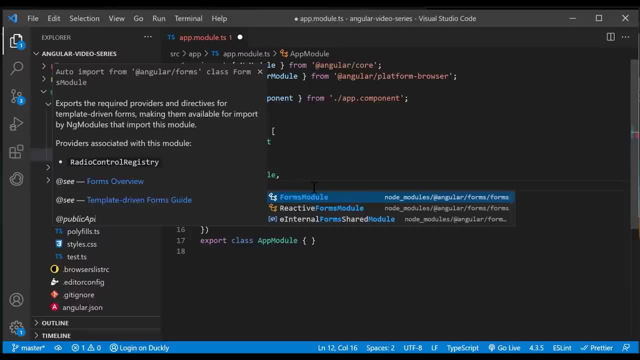 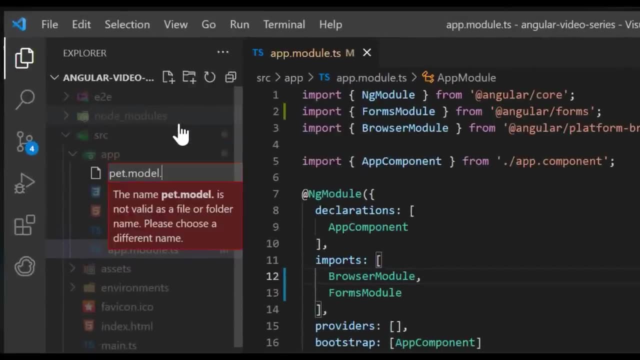 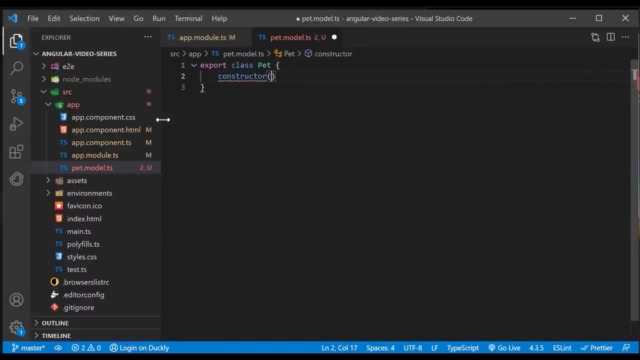 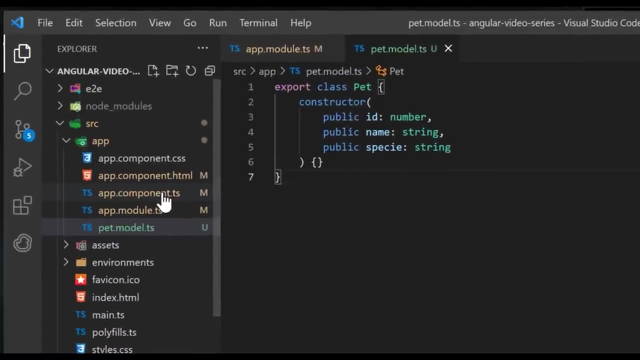 import forms module in your app root module. Let's first build our form. Let's import our class, which defines a data model reflected in our form. I will have three properties: ID, name and specie. Now let's import our class in the app component. 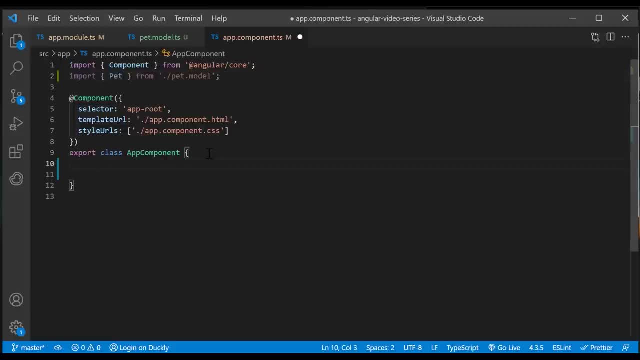 Define species in species array. Now create a model from the pet class and pass the values for our pet. Here we're using dummy data, but in your real app you would use a service to get the data from the API and to save it. 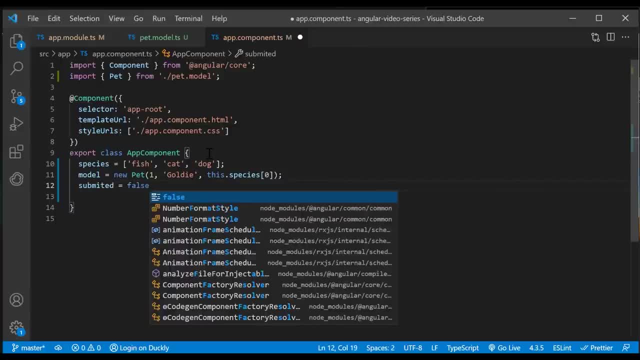 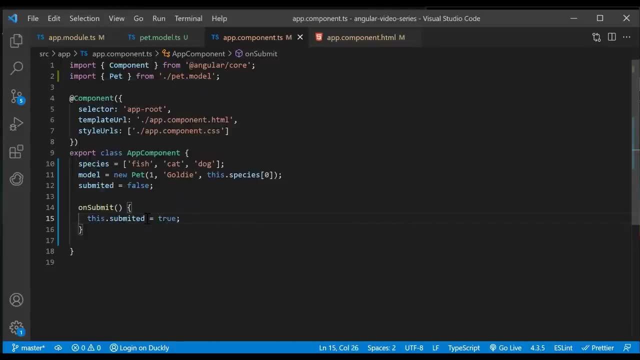 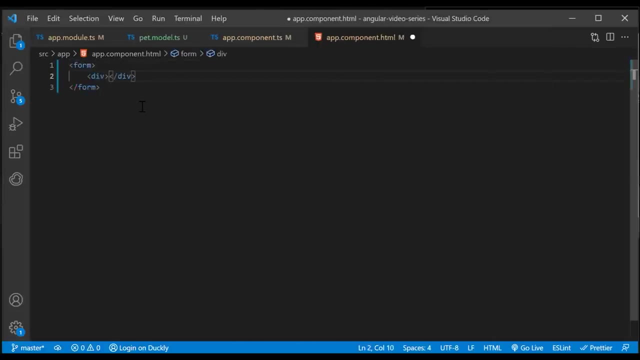 Also, let's add submitted property. This will change depending on the state of the form and on submit method. Next, in our HTML file, we will create a form that reflects our data model. Create a form and inside it two divs for two fields. First will be name input. 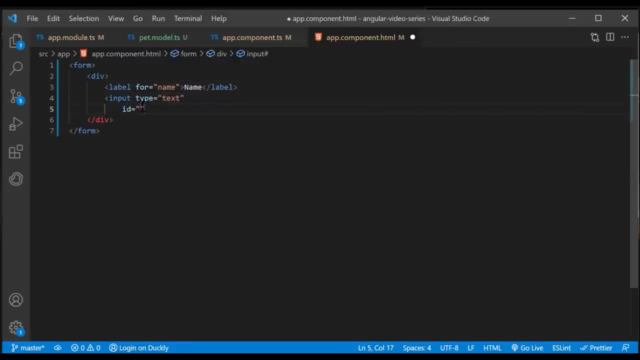 And I'm adding label and required attribute to our input. And the second one will be a select which will loop through an array of species to show all the values from the array. Same as for input: I'm adding label for our select And also I will add the required attribute. 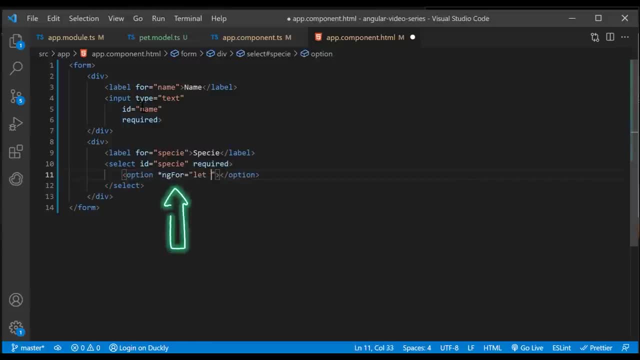 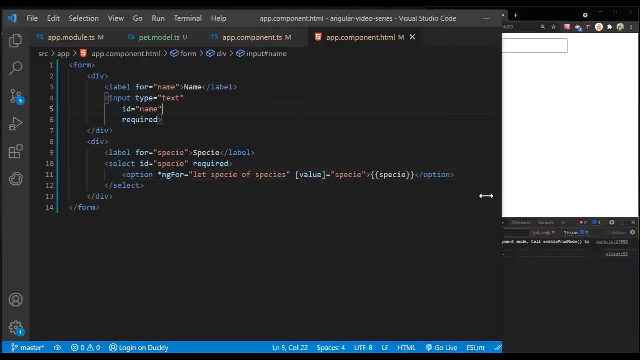 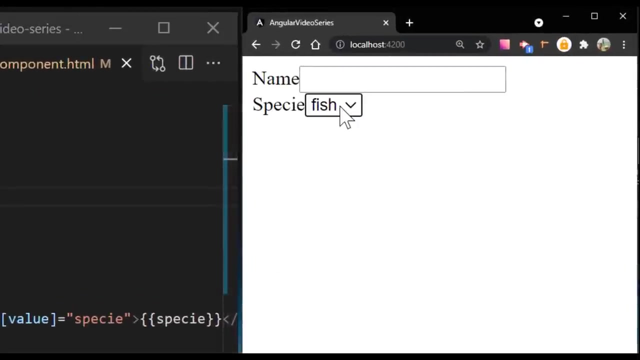 Then I will use ng for to load through all the values and display them. If you run the application right now, you see the list of species in the selection control. the input elements are not yet bound to data values or events, So they are still blank and have no behavior. 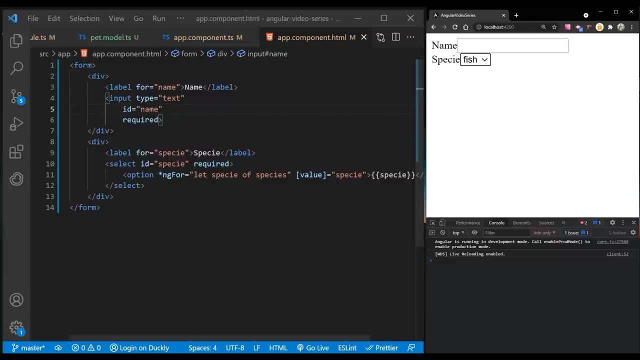 The next step is to bind the input controls to the corresponding pet properties with two way data by name, so that they respond to the user input by updating the data model and also respond to programmatic changes in the data by updating the display. The ng model directive declared in the 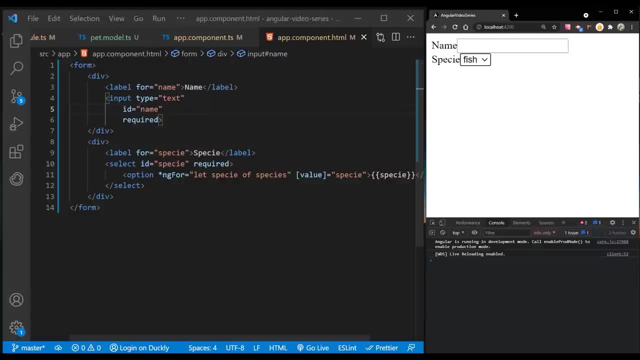 forms module lets you bind controls in your template driven form to properties in your data model. Add the ng model directive using two way data binding syntax: for the name use model dot name. And for species use model dot- specie value. When you use ng model on an element, you must define: 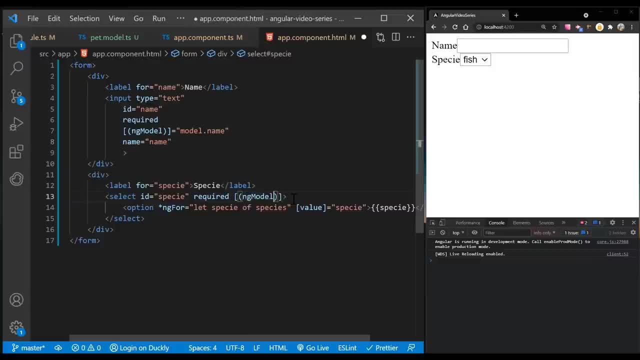 a name attribute for that element. Angular uses the assigned name to register the element with the ng form directive attached to the parent form element. So in order to register our form, add a template reference variable with a value of ng form. The pet form template variable is now a. 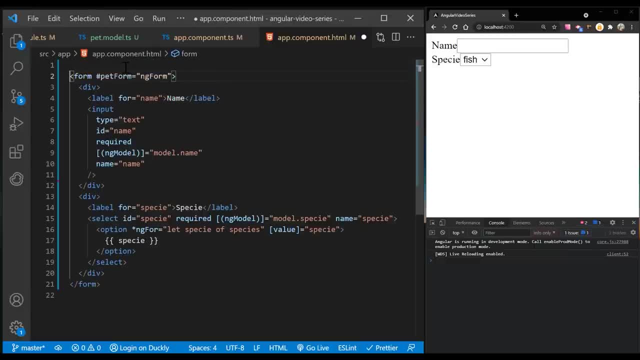 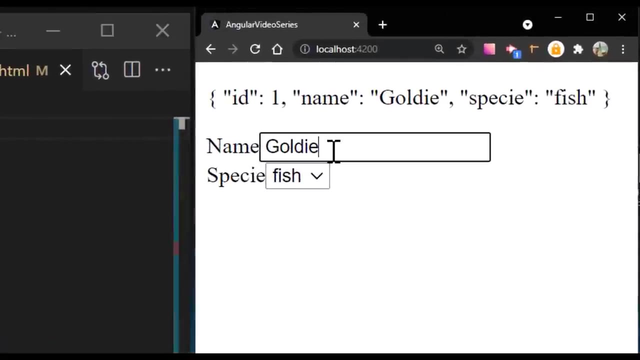 reference to the ng form variable. The pet form template variable is now a reference to the ng form directive instance that governs the form as a whole. In order to test our application, place the model object in our template with a JSON pipe. Now, if you update your form films, you will see that model is being updated. 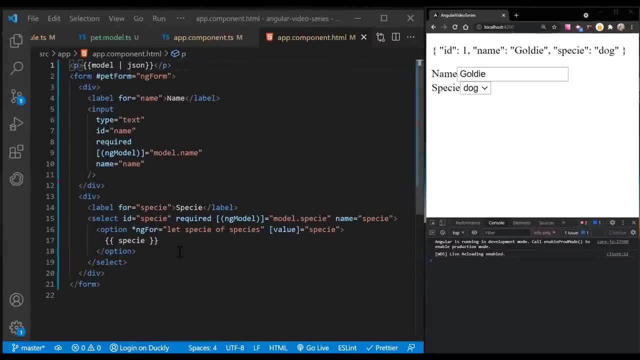 Now the user should be able to submit this form after filling it. Create a submit button on the bottom. The submit button at the bottom of the form does nothing on its own, But it does trigger a form submit event because of its type. submit To respond to this. 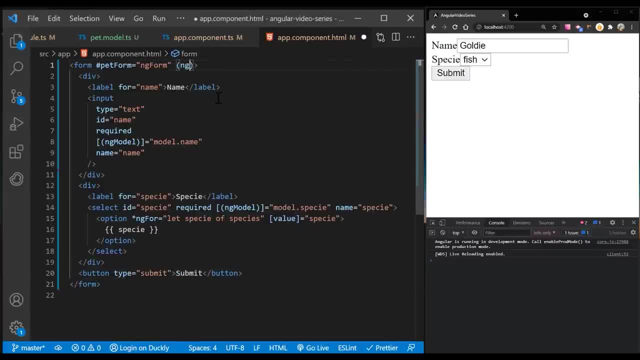 event. take the following steps: Bind the forms ng. submit event property to the pet form component. on submit method: Use the template reference variable Pet form to access the form that contains the submit button and create an event binding. You will bind the form property that indicates its overall validity to the submit buttons disabled. 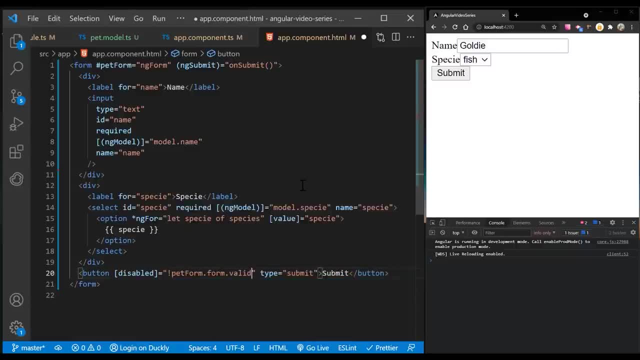 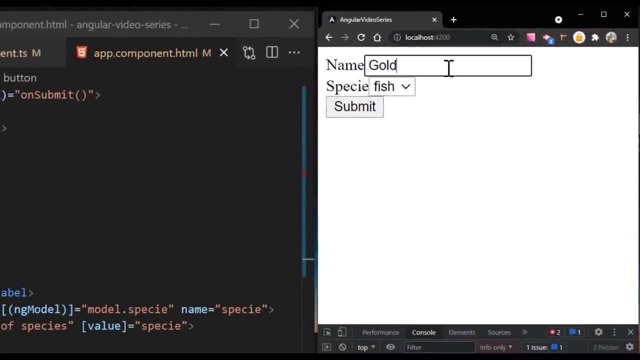 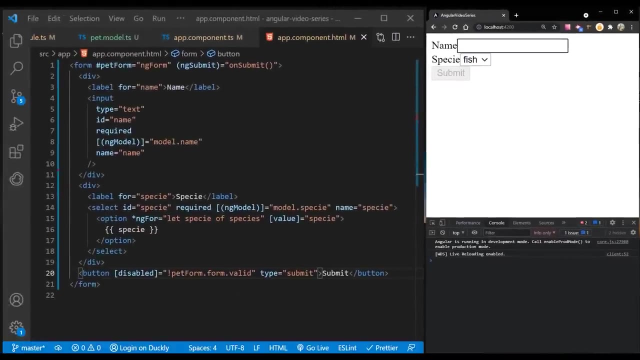 property. Run the application now. Notice that the button is enabled, although it doesn't do anything useful yet. Delete the name value. This violates the required rule, so it disables the submit button. To show a response to form submission, you can hide the data entry area and display something. 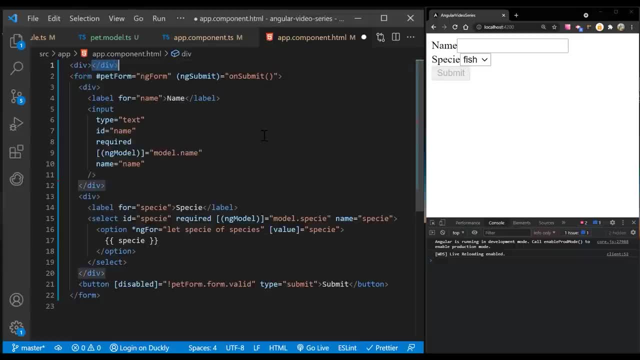 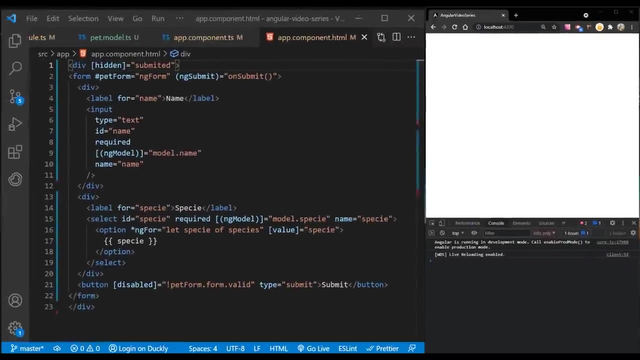 else in its place. Wrap the entire form in a div and bind its hidden property to the app component. submitted property. The main form is visible from the start because the submitted property is false until you submit the form, as this fragment from the app component shows. To show a response to form submission, you can hide the data entry area and display something else in its place. Wrap the entire form in a div and bind its hidden property to the app component submitted property. The main form is visible from the start because the submitted property is false until you submit the form, as this fragment from the app component shows. 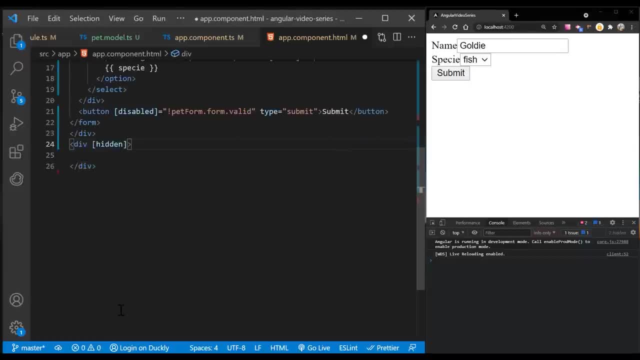 To show a response to form submission, you can hide the data entry area and display something else in its place. Wrap the entire form in a div and bind its hidden property to the app component submitted property. To show something else while the form is in submitted state, add the following HTML below: 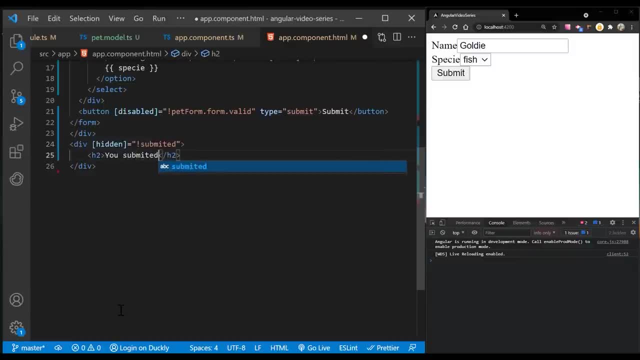 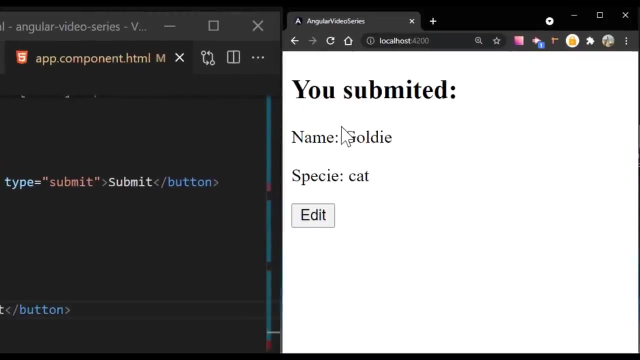 the new div wrapper, Add the properties that you updated and the Edit button if the user wants to update the fields again. And now let's preview how it works. That's all about template driven forms. Now, in the next section, we're going to see how we can take more control of our forms. 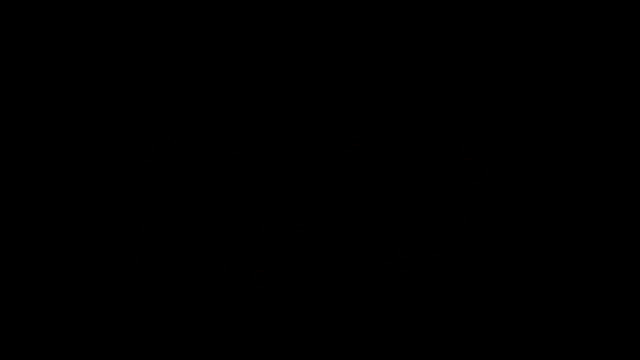 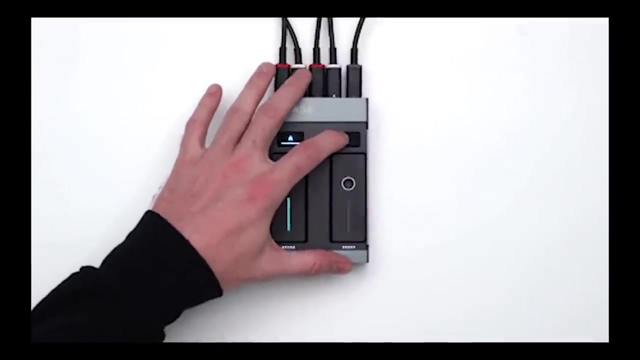 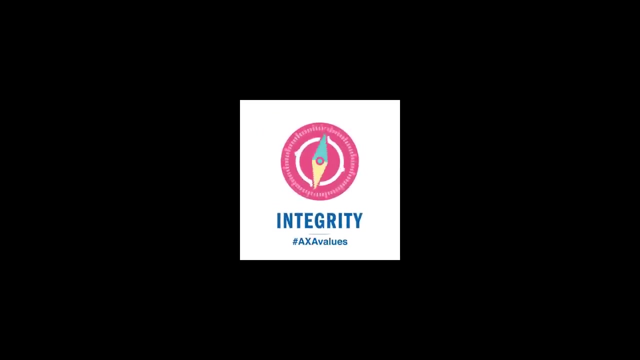 and how to create them. Create reactive forms. Reactive forms provide a model driven approach to handling form inputs whose values change over time. Each change to the form state returns a new state which maintains the integrity of the model between changes. Let's add basic form control. 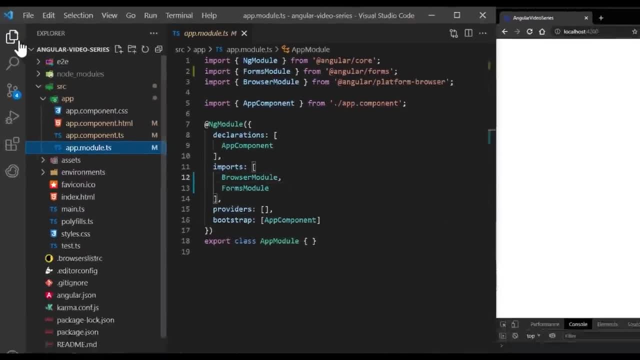 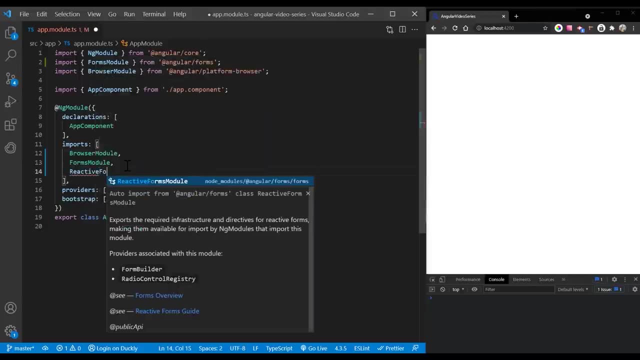 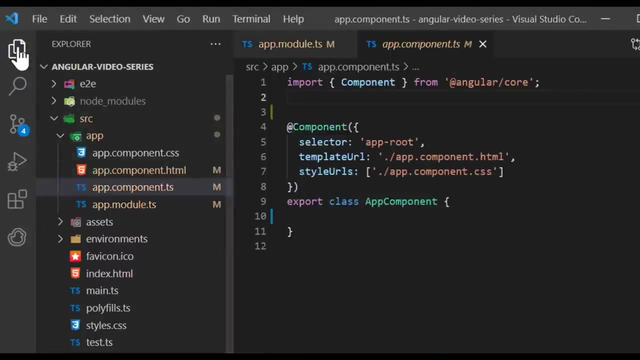 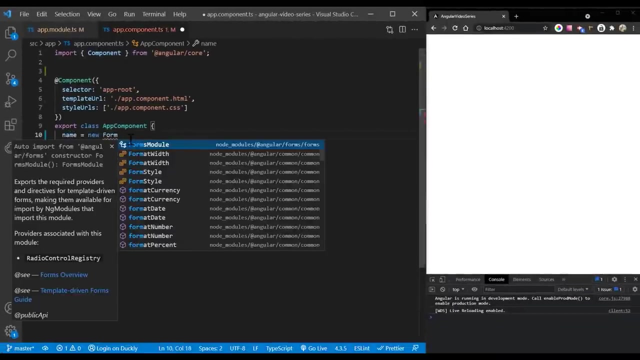 To use reactive form controls. import reactive forms module from Angular forms package and add it to your ng modules. import array To register a single form control. import a form control class and create a new instance of form control to save as a class property. 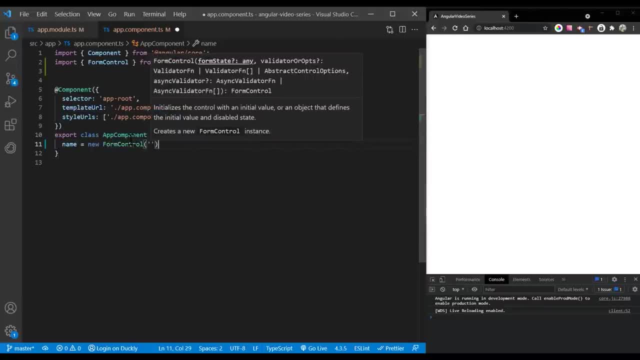 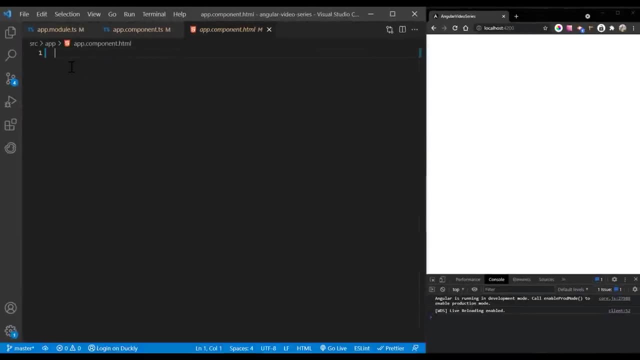 Use the constructor of form control to set its initial value, which, in this case, is an empty string. By creating these controls in your component class, you get immediate access to listen for, update and validate the state of the form. To save the class property, use the constructor of form control to set its initial value. 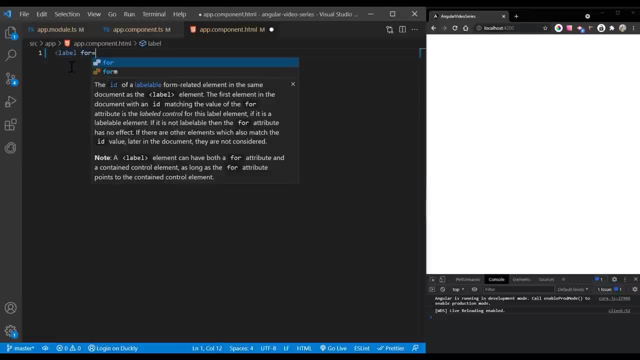 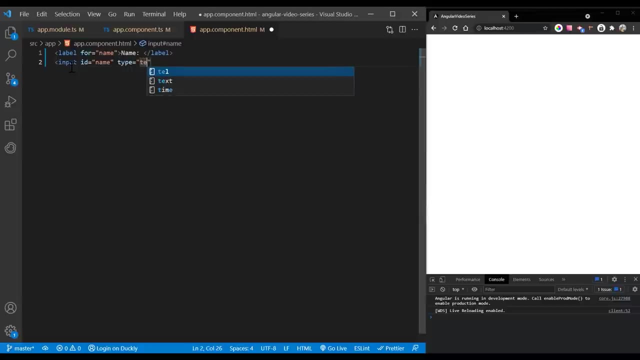 which in this case is an empty string. the form input: After you create a control in the component class, you must associate it with a form control element in the template. Update the template with the form control using the form control binding provided by form control directive, which is also included in the reactive forms. 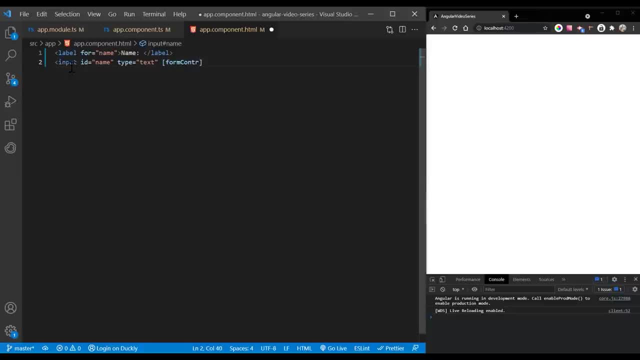 module Using the template binding syntax. the form control is now registered to the name input element in the template. you can display the value in the following ways: Through the value changes observable, where you can listen for changes in the forms value in the template. using async pipe. 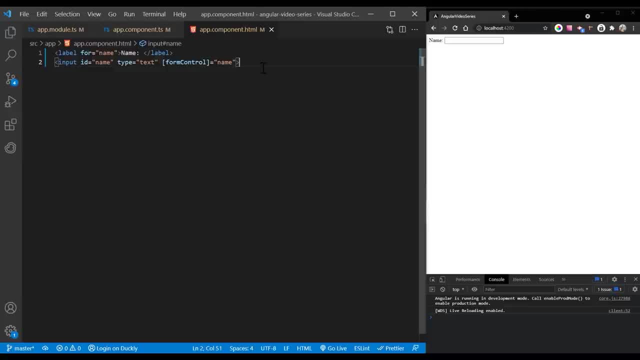 or in the component class, using the subscribe method or with the value property, which gives you a snapshot of the current value. The following example shows you how to display the current value using interpolation in the template. The displayed value is displayed in the template. 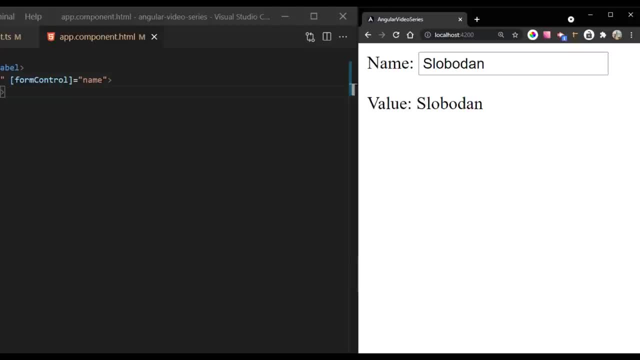 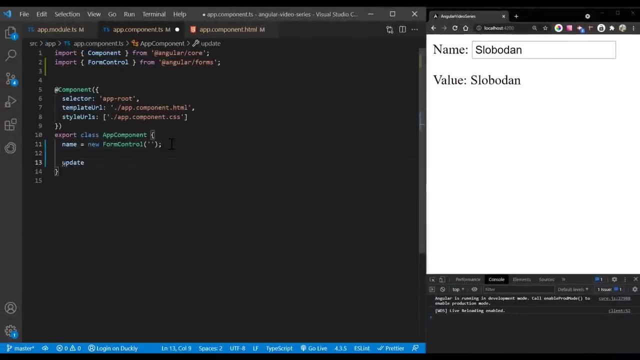 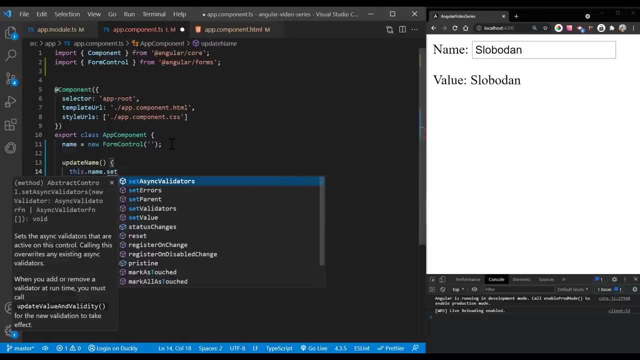 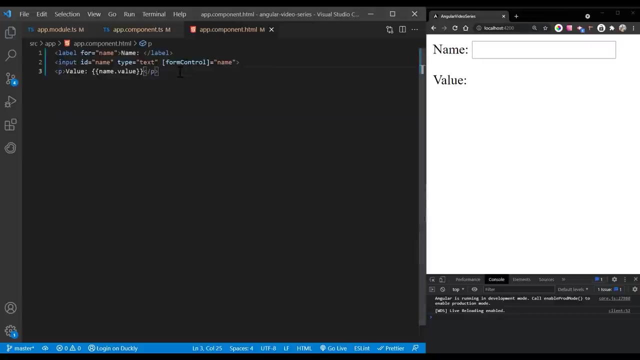 The value changes as you update the form control element. Reactive forms have methods to change the controls value programmatically, which gives you the flexibility to update the value without user interaction. The following example adds a method to the component class to update the value of the control to Nancy using the set value method. Update the template with a button to simulate. 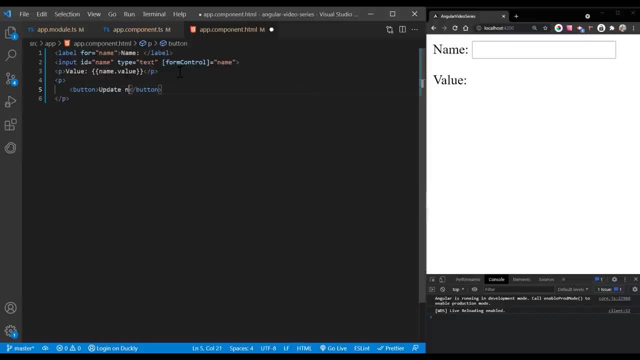 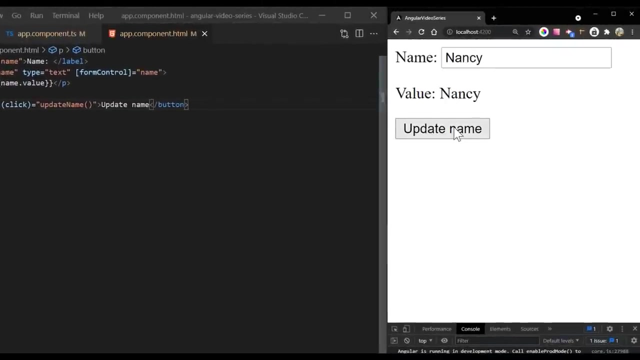 a name update. When you click the update name button, the value entered in the form control element is reflected as its current value. The form model is the source of truth for the control. So when you click the button, the value of the input is changed within the component class, overriding its current value. 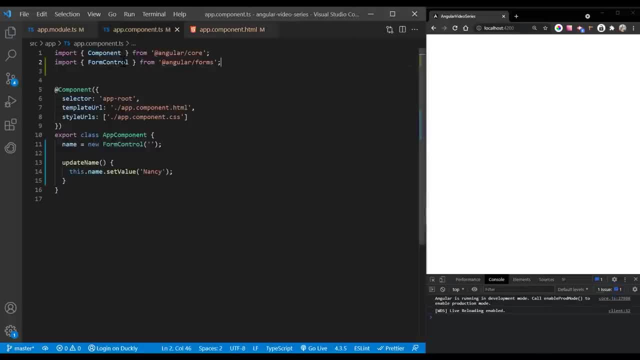 Forms typically contain several related controls. Reactive forms provide two ways of grouping multiple related controls into a single input form. First way of form group defines a form with a fixed set of controls that you can manage together. And second way of form array defines a dynamic form where you can add and remove controls. 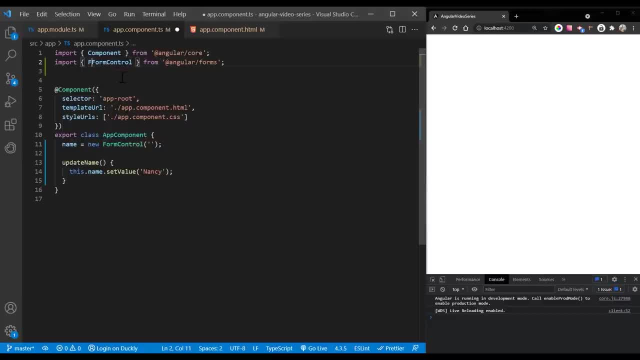 at runtime. Import the form group and form control classes from the Angular forms package. Create a property in the component class named profile form and set the property to a new form group instance. Create a property in the component class named profile form and set the property to a new form group instance. 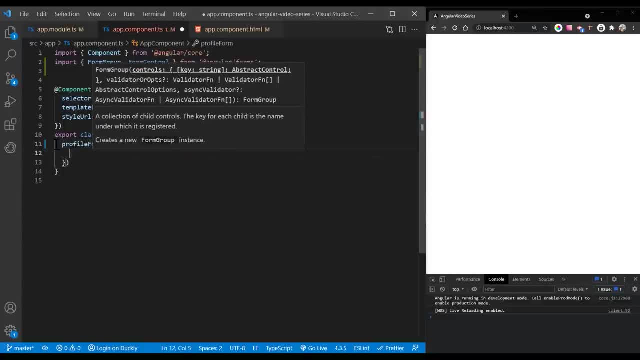 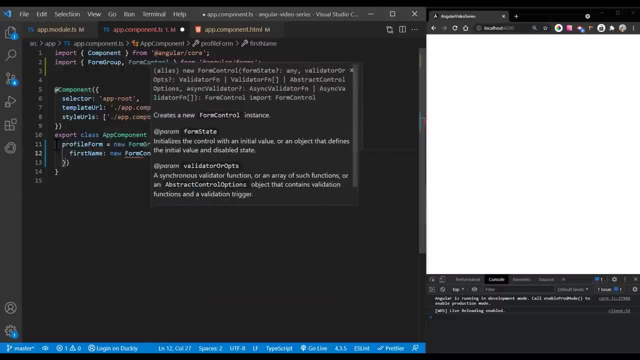 Create a property in the component class named profile form and set the property to a new form group instance. To initialize the form group. provide the constructor with an object of named keys mapped to their control For the profile form. add two form control instances with the names. 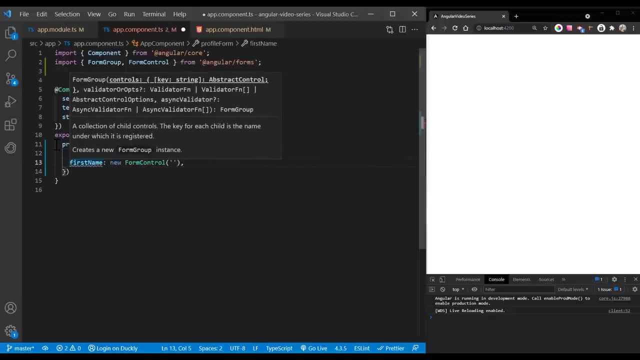 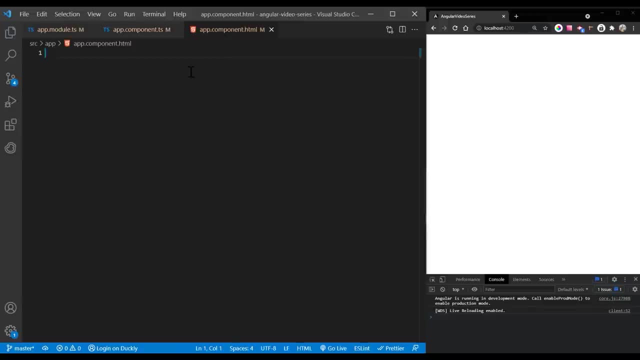 first name and last name. The individual form controls are now collected within a group. After you define a model, you must update the template to reflect the model. in the view, I am adding two inputs and two labels that match our model. The form control name input provided by the 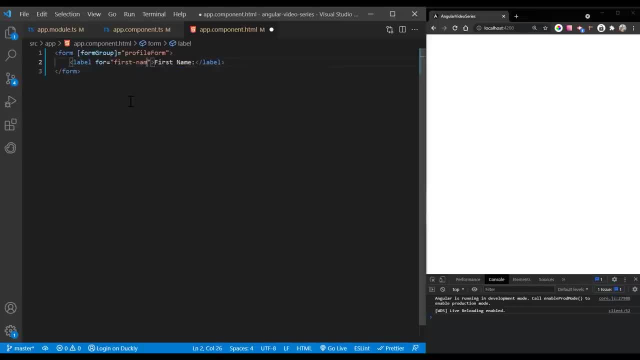 form control name directive binds each individual input to the form control defined in the form group. The form group directive listens for the submit event emitted by the form element and emits an ng submit event that you can bind to a callback function. Add an ng submit event listener to the form tag with the on submit callback method. 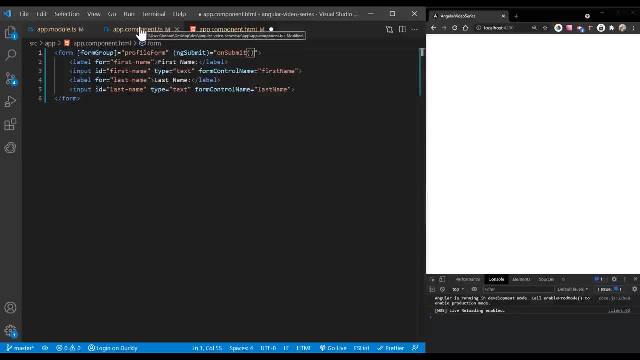 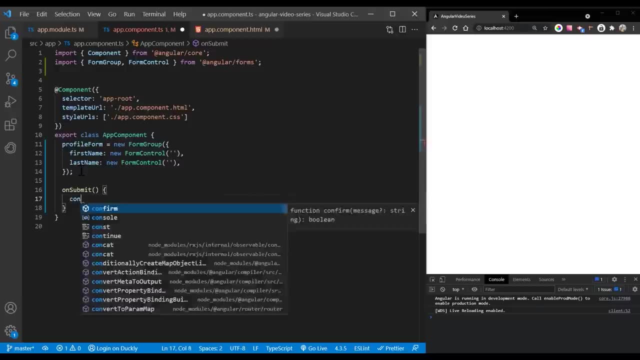 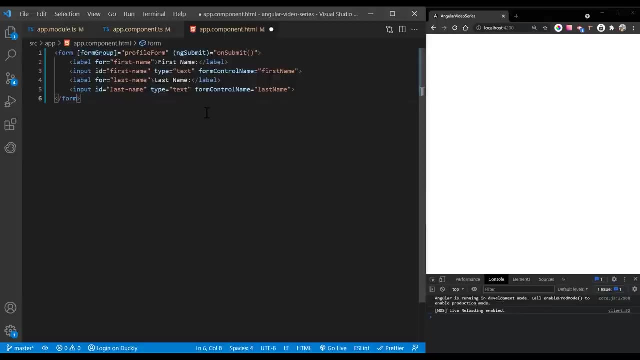 The on submit method captures the current value of profile form and the on submit method captures the current value of profile form. Here you will just log the form value. The submit event is emitted by the form tag using the native DOM event. You trigger the event by clicking a button with submit type. 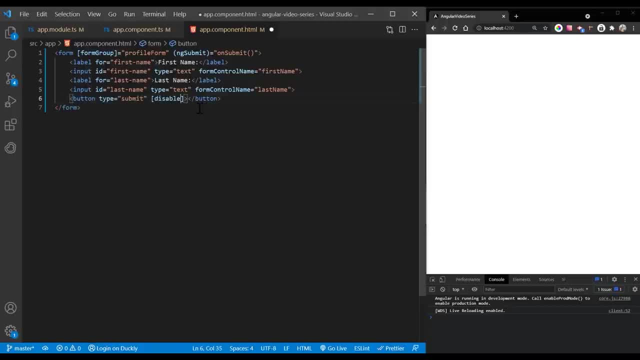 This allows the user to press the enter key to submit the completed form. Add a button to the bottom of the form to trigger the form submission. You can also add a button to the bottom of the form to trigger the form submission. And that's all for reactive forms. 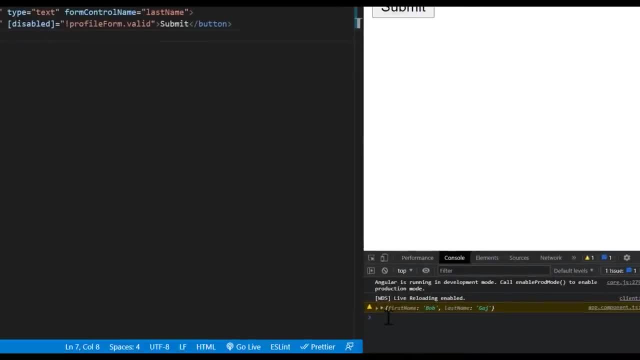 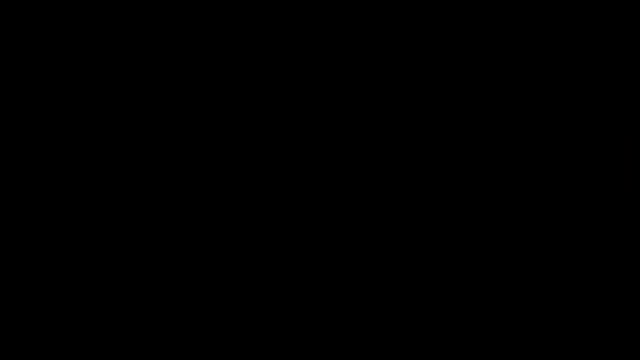 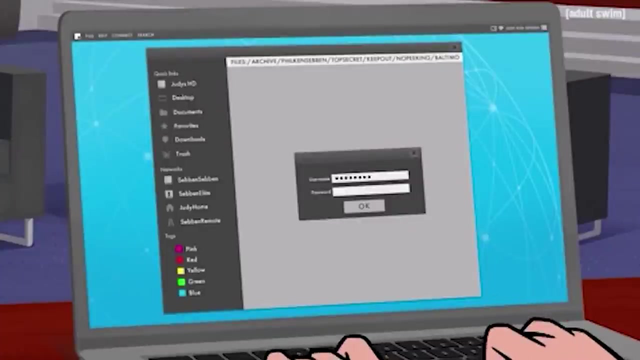 In the next section we are going to see how we can improve our forms, So in this section we are covering form validation. This tutorial will show you how to validate user input from the UI and display useful validation messages in both reactive and template driven forms. 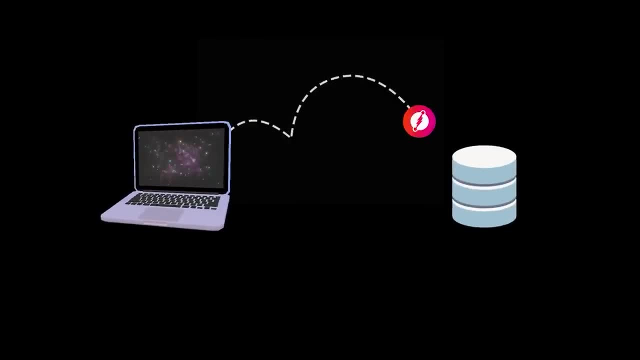 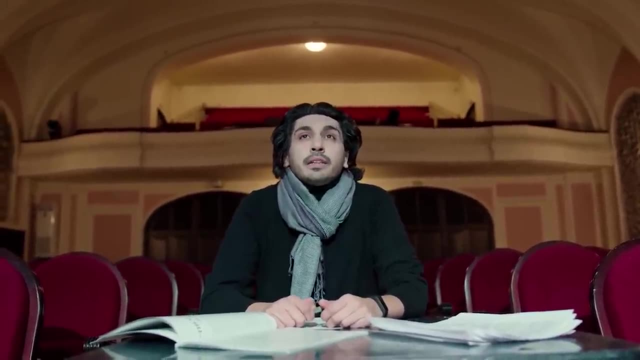 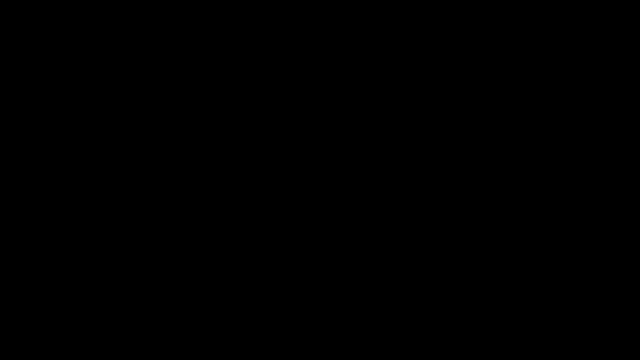 Anything that you want to store to your database needs to have multiple levels of validation, And I see validation the same as if you're at an audition or job interview- Something, or rather someone is presenting to you and you decide: will he pass or not. To add validation to a template driven form. 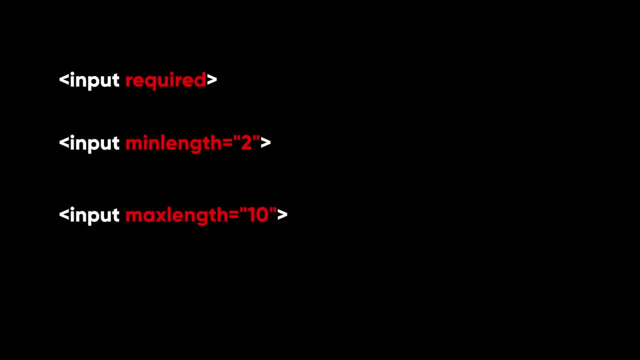 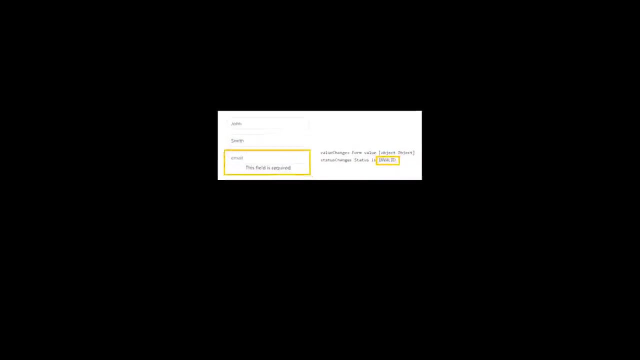 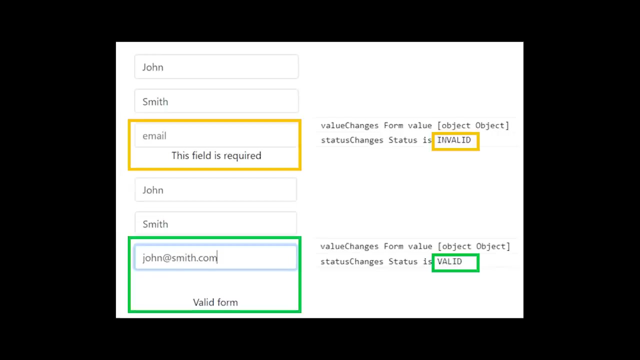 you add the same validation attributes as you would with native HTML form validation. Angular uses directives to match these attributes with validator functions in the framework. Every time the value of a form control changes, Angular runs validation and generates either a list of validation errors that results in an invalid status, or null, which results in a valid 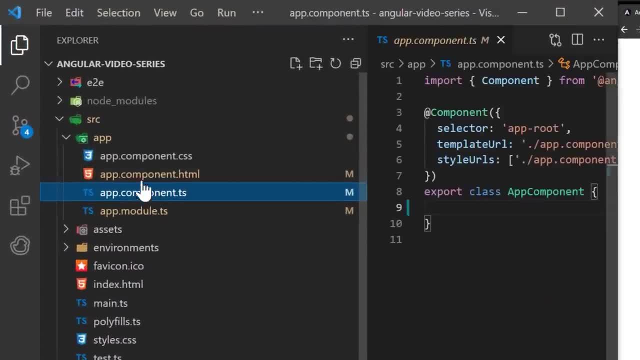 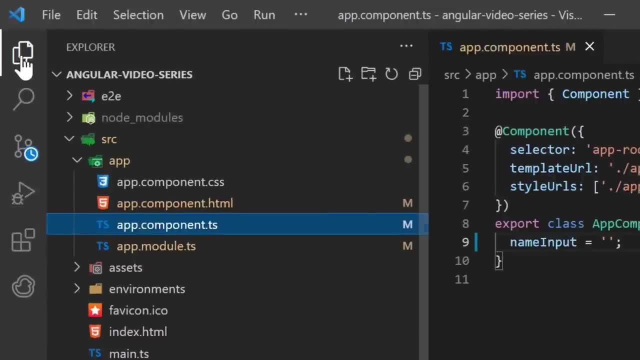 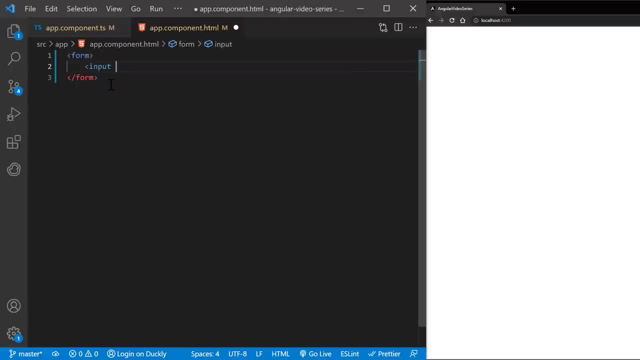 status. I'll create a name string field inside of our component class. Then in our HTML file I'll add an input text field with required attributes. In this case I'm going to attribute a min length of four. I'm binding name input property to ng model and I'm exporting ng model to a local variable called. 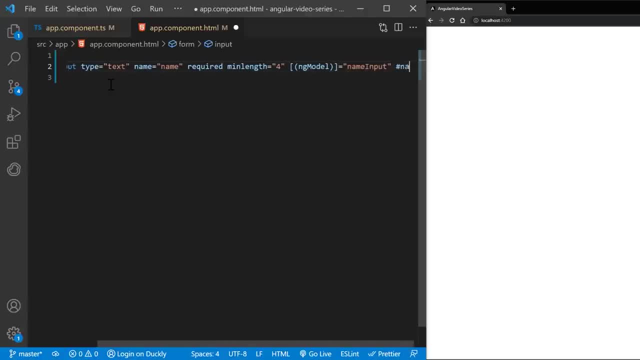 main ng model mirrors many of the properties of its underlying form control instance, So you can use this in template to check for control. And here we're going to add a description and a name for a past name View. Let's see how it works. 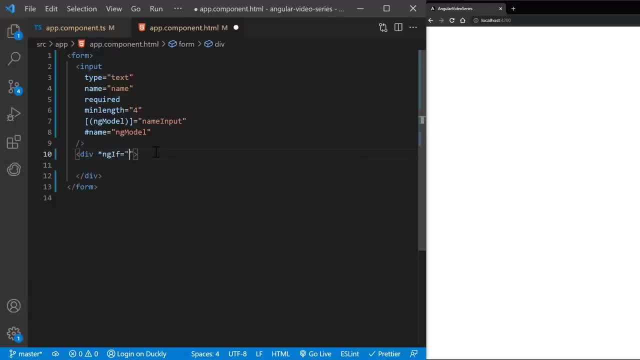 I'm going to create a new 900 text name. I'm going to name this one V And I'm going to assign it to the target function, depending on the value of the name- Let's say native 더를- and I'm going to assign it to the target function. 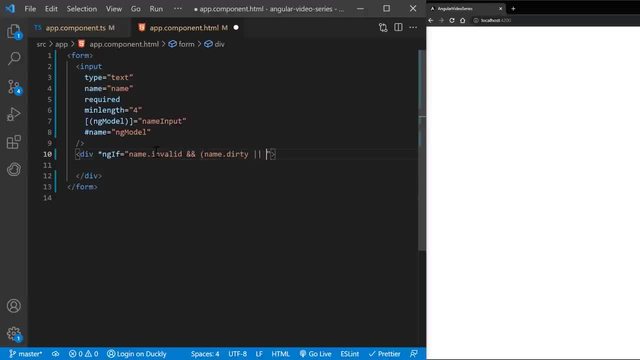 And I'm going to assign it to a typical target object. And let's define the daily data type which is given by the user. I'm going to assign the default value to the target object And in the background I'm going to add a data type. 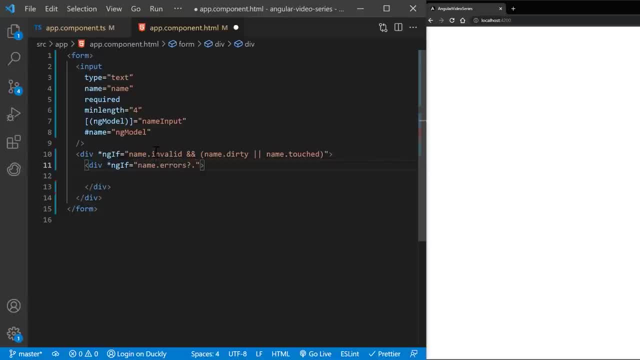 I'll assign a list of values, including port, if I'm going to add any data types. from this data type, I'm going to add a list of domestic values And I'm going to add a list of default values. Let's wait a moment. 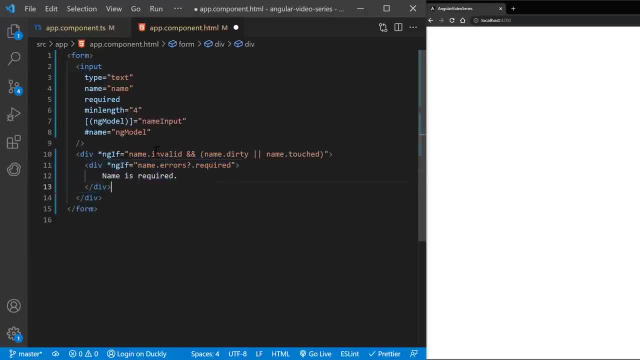 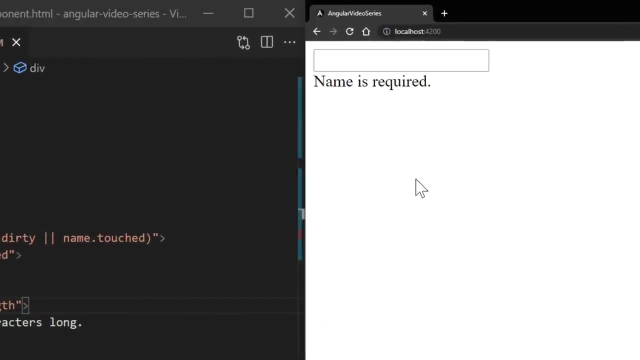 these are messages for acquired and min led. Now, if you type something and leave the field empty, we will get the validation error message, And the same goes if you enter value less than four characters long In a reactive form. the source of truth is a component class. 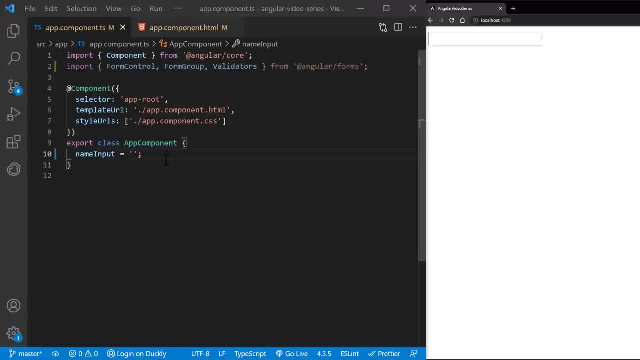 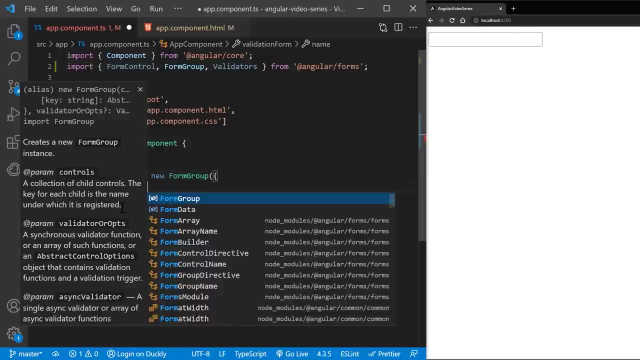 Instead of adding validators through attributes in the template, you add value data function directly to the form control model in the component class. The same built in. validators that are available as attributes in template driven forms, such as required and mainland, are all available to use as functions from the validator class. 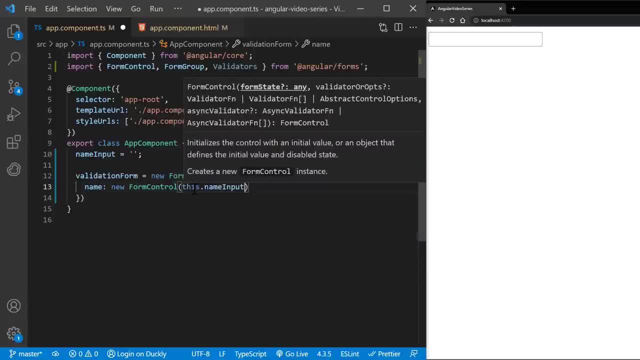 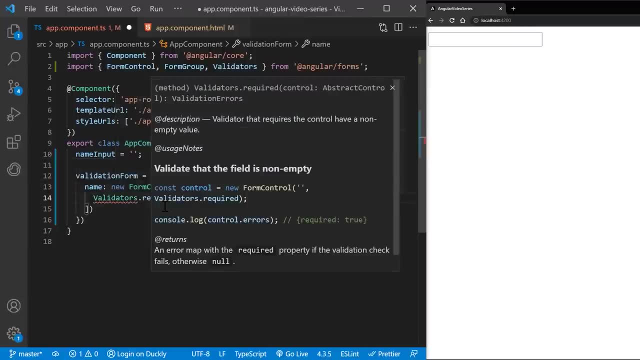 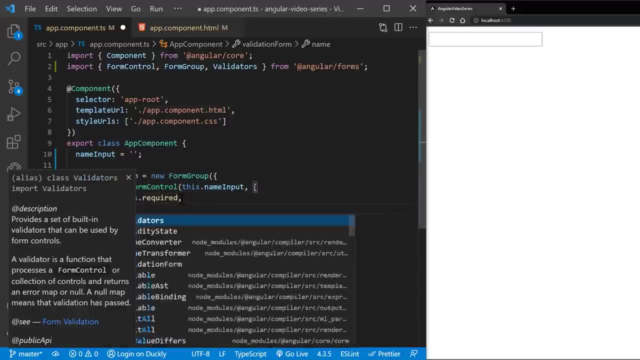 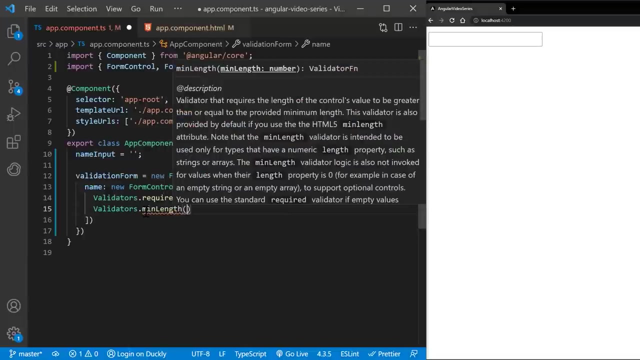 To update the validation form to be a reactive form, use some of the same built in validators. In this example, the name control sets up two built in validators: validators required and validators mainland. These validators are synchronous, so they're passed as the second argument. Notice that you can support multiple validators by passing the functions. 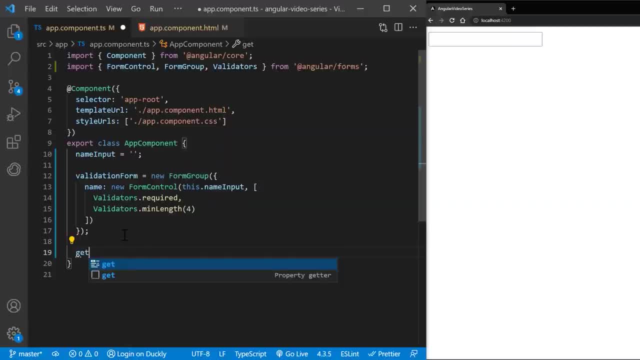 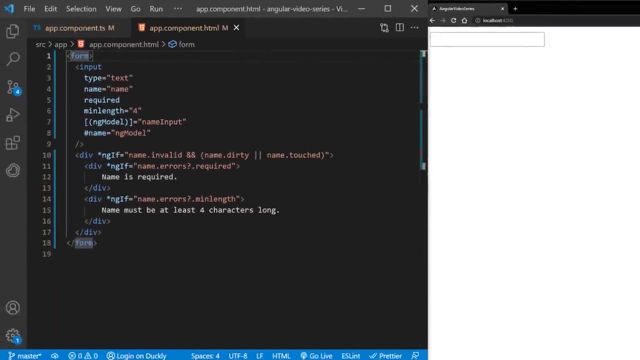 in as an array. This example also adds a getter method In a reactive form. you can always access any form control through the get method on its parent group, But sometimes it's useful to define getters as shorthand for the template In our template. add form group to our form. 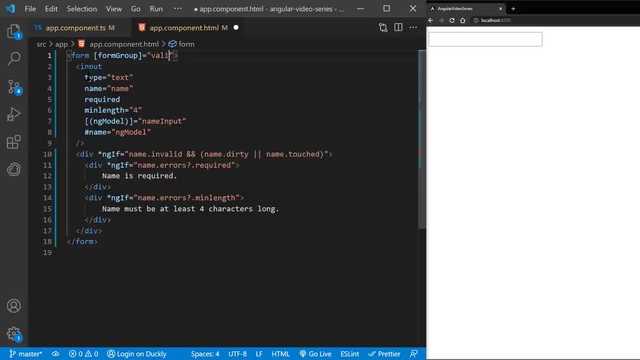 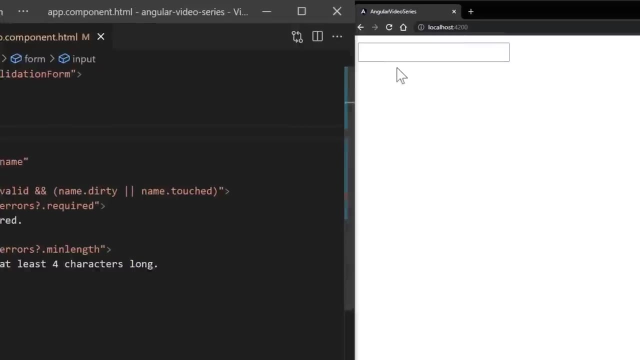 And now the only thing that we need to change in our template to make it reactive is to remove ng model and to bind our name control to form control name. This form differs from the template driven version in that it no longer exports any directives. 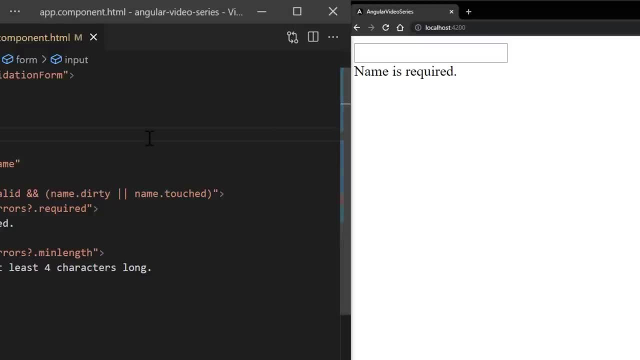 Instead, it uses the name getter defined in the component class. Notice that the required attribute is still present in the template. Although it's not necessary for validation, it should be retained for accessibility purpose. And now let's see how it works. 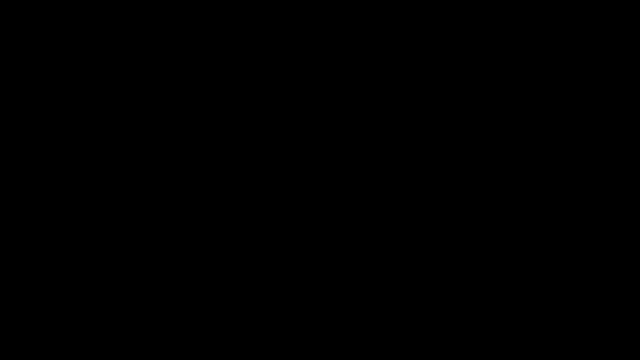 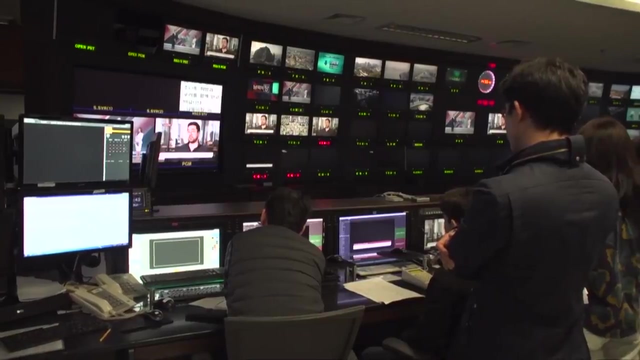 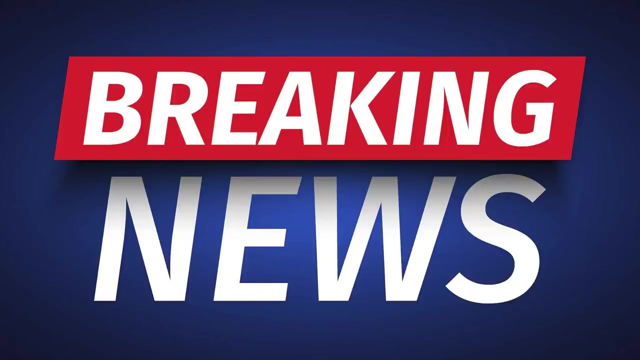 Let's see how it works. We finally came to the end of this long tutorial and we're gonna cover communication using HTTP client. Imagine that you're running a TV station or a newspaper, And what if you lose communication with your reporters? You would end up with a blank newspaper or no news to broadcast. 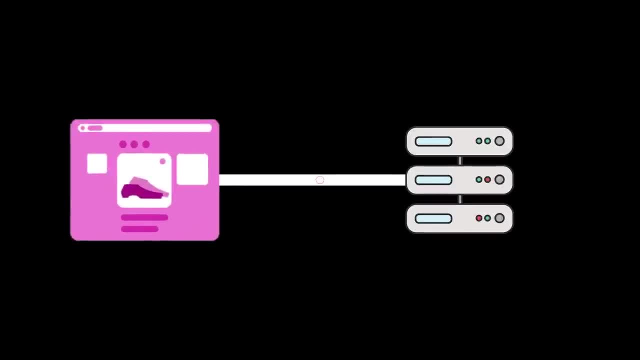 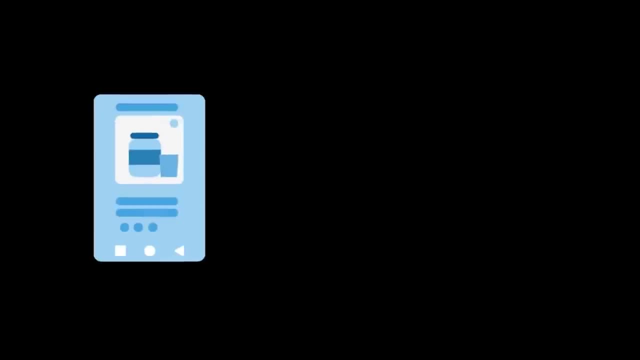 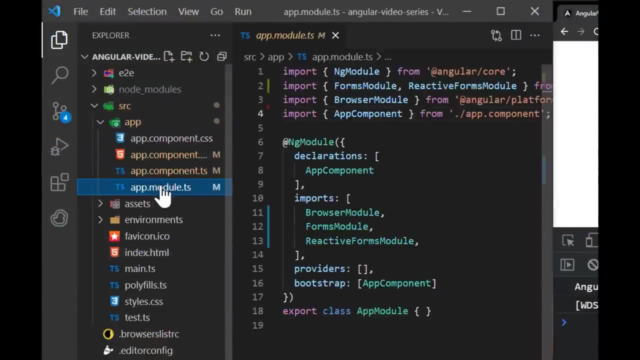 It's the same thing with web apps. Without backend communication, our apps would be dead. without information or instructions from the backend, Most front-end applications need to communicate with a server- H T P protocol- to download or upload data and access other backend services. 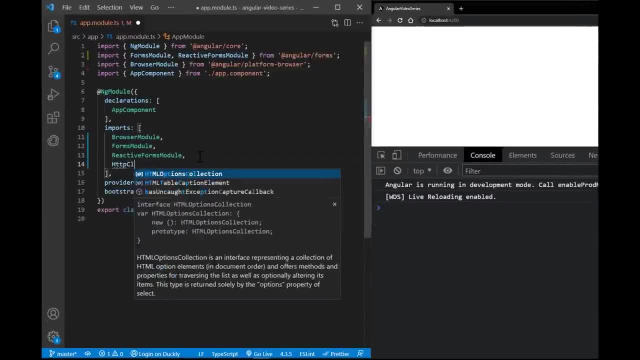 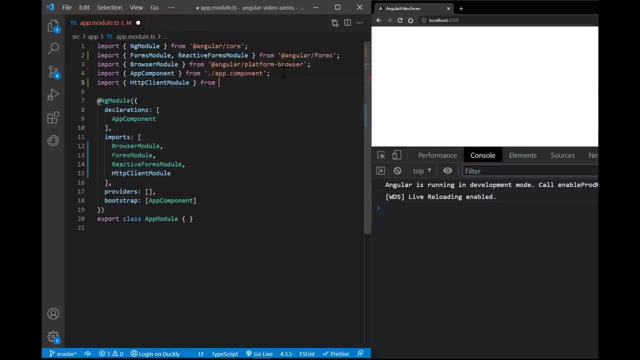 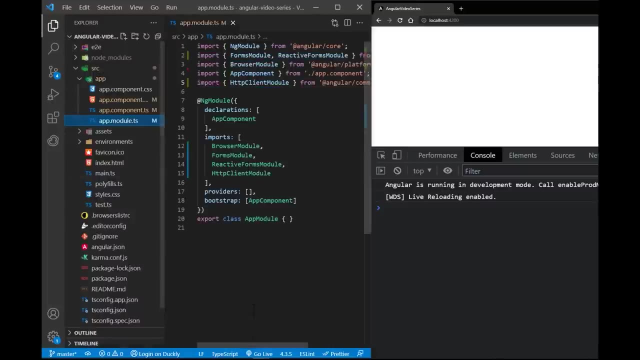 Before you can use HTP client, you need to import angular adv자를 client module. most apps do so in the root app module. eh, let's create data service. Most common use case is about ingesting an setup agent Ltd. 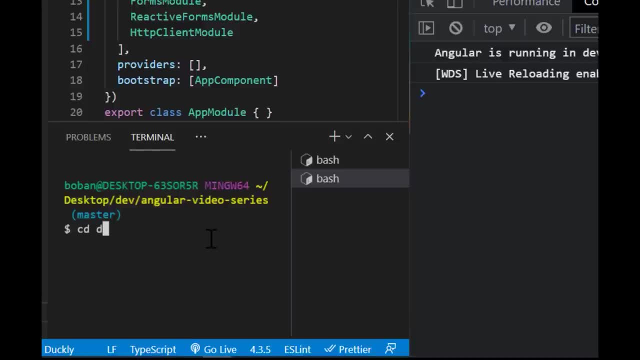 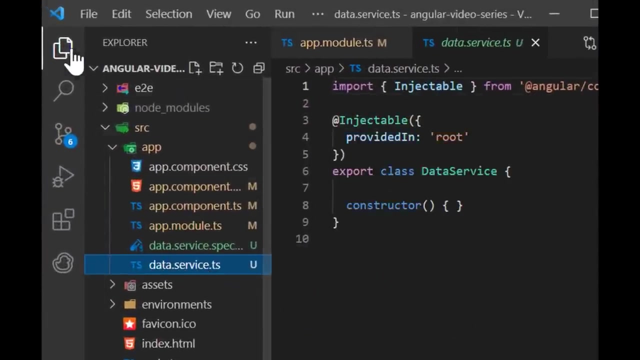 HTTP client into service and use it throughout the application. you can then inject HTTP client service as a dependency of an application class, as shown in this example. Now let's see how we can fetch data from a server. To do that, we're going to use HTTP client get method First inject. 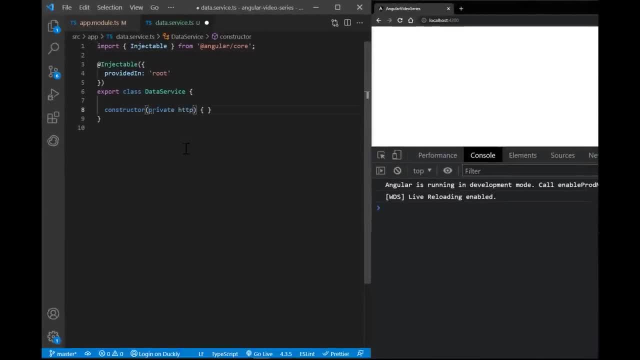 HTTP client into our service, Then create get data method And inside of this method we're gonna fetch our data. The get method takes two arguments: the endpoint URL from which to fetch and an option subject that you use to configure the request to add things like parameters to your 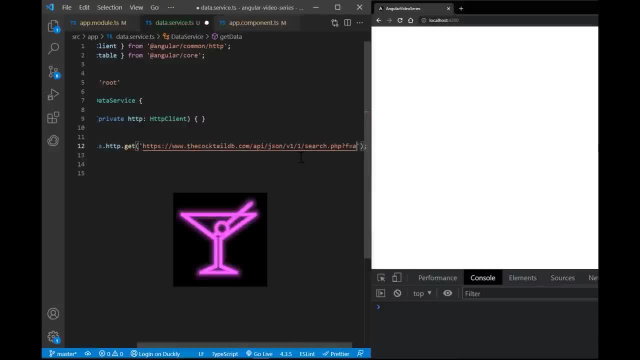 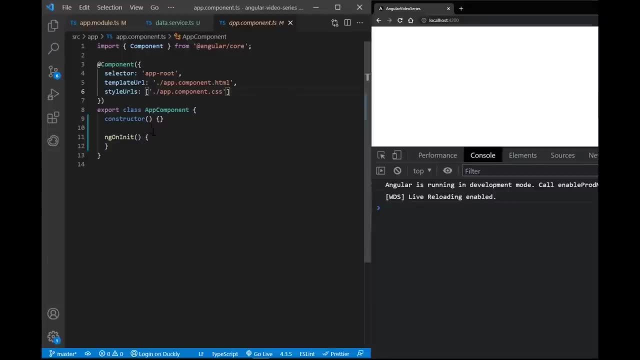 requests For this tutorial. I found a free cocktail API service. The link will be in the description box below. Enter the URL and no additional parameters are required in this case. Now in our app component, we inject the data service in the constructor. 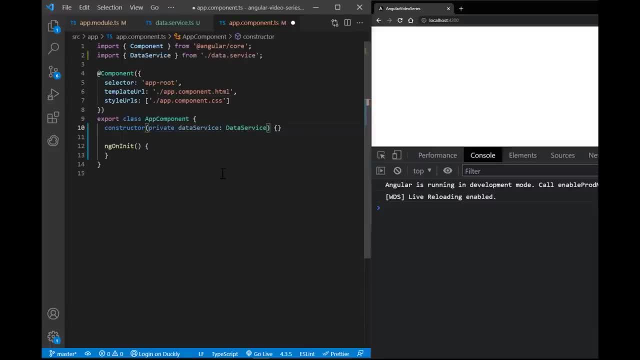 And inside of ng onInit method, let's call our get data method, Because the service method returns an observable. the component subscribes to the methods return value. I'll show you how to do that in a minute. I'll show you how to do that in a minute. 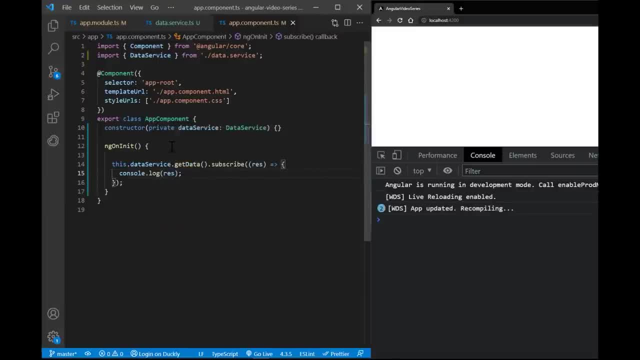 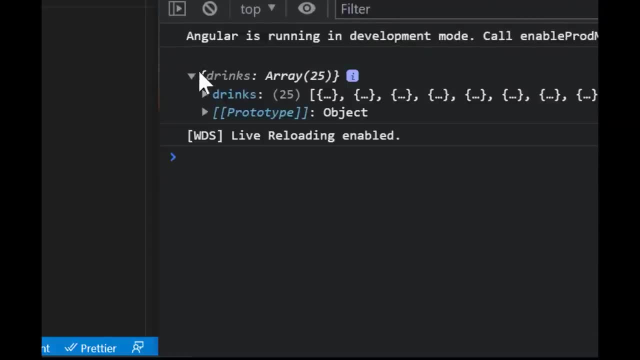 I'll show you how to do that in a minute. I'm just gonna console log it And that's how you get data from the server. In an ideal world, everything works as a magic. But we don't live in an ideal world, unfortunately. 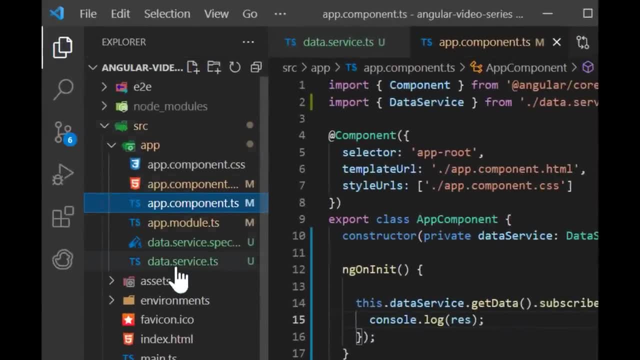 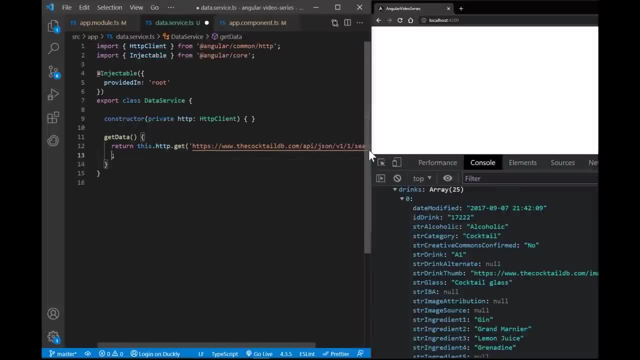 and we lose connection with API sometimes. So we need to handle errors when they come up. If the request fails on the server, HTTP client returns an error object instead of a successful response. Let's add a pipe in our get method and use catch error to catch it. 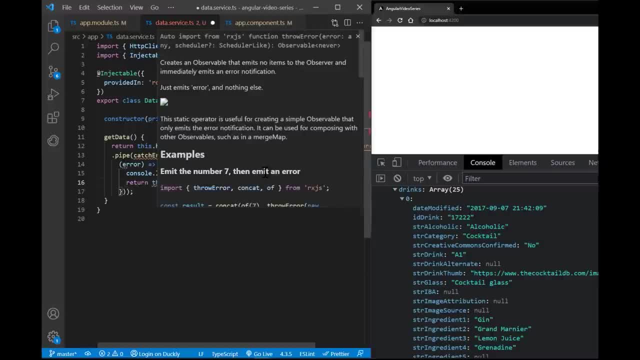 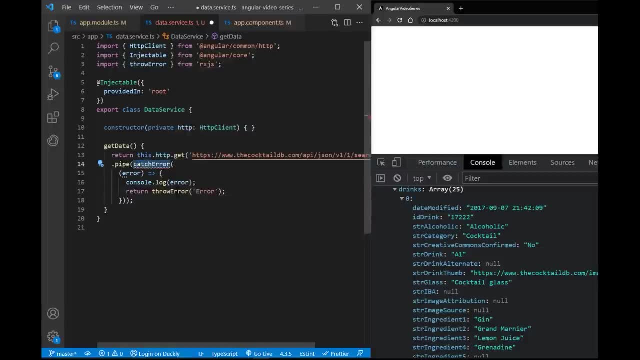 I'm gonna log the error for development purpose and return throw error with some message. This should be used in your application to show the user that his request has failed. Without notification, they wouldn't know what's happening. And don't forget to import missing packages. 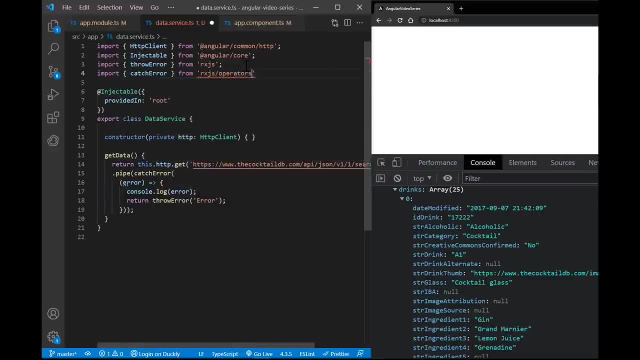 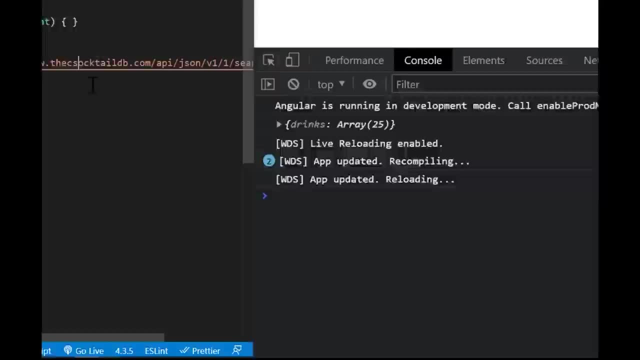 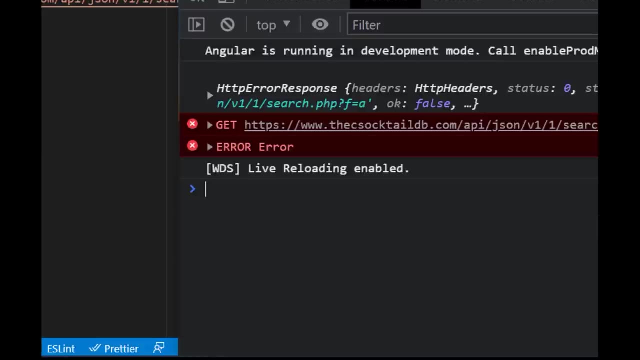 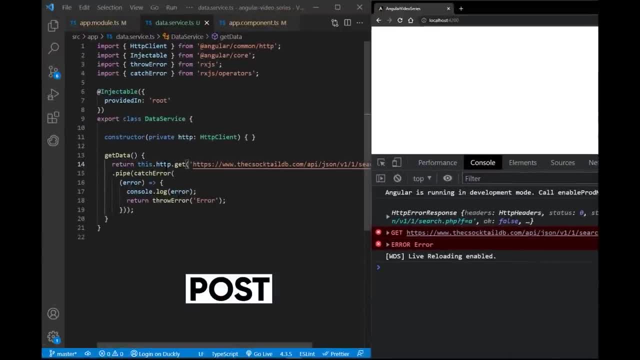 a post method for submitting data to server. For example, if you are submitting a form, we have delete request for deleting data from database, obviously a put request, which replaces a resource with updated data. Now most of the API's require an authentication key with their 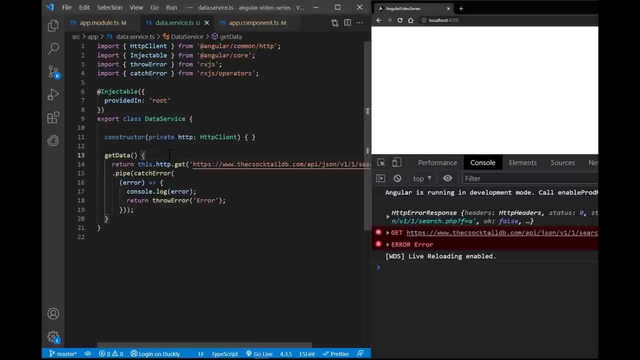 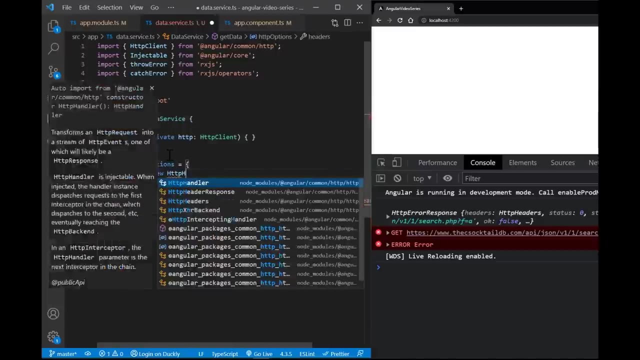 requests. So let's see how we can add that. I found this Lord of rings database which requires an auth key. Let's create HTTP options object with a headers property. This property will be a new HTTP header subject and we will pass two properties: content type as application. 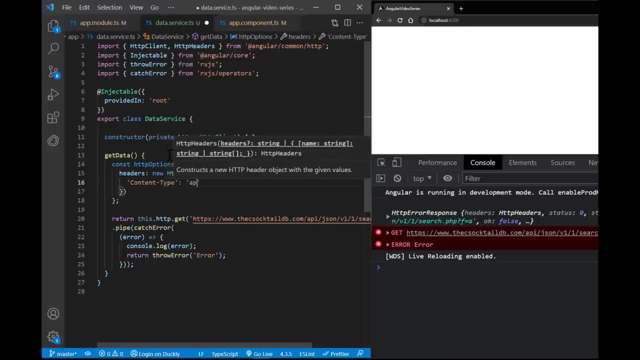 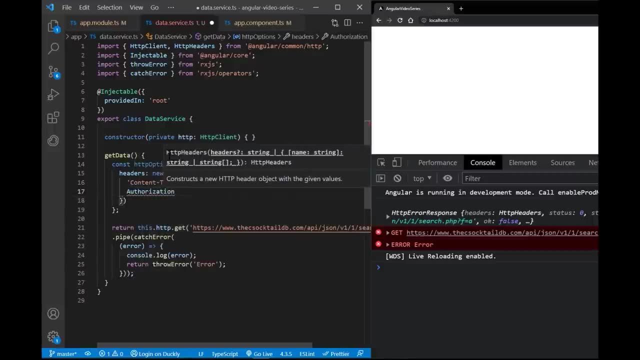 JSON, which means that we are using JSON as content And authorization where we enter our API key. barrier is type of authorization and followed by a key. In order to get your personal key you need to register. link is in the description box below. Now update the API endpoint. 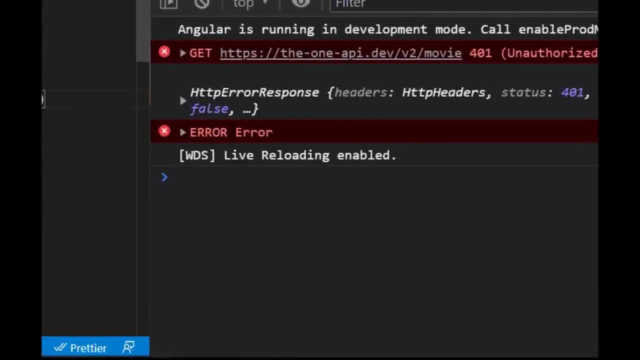 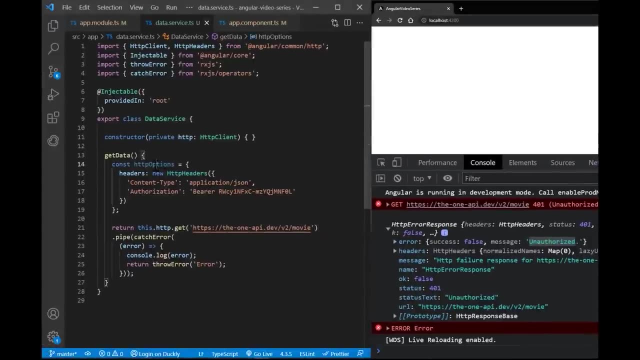 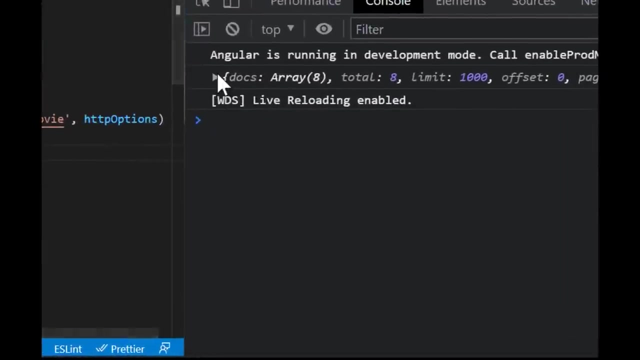 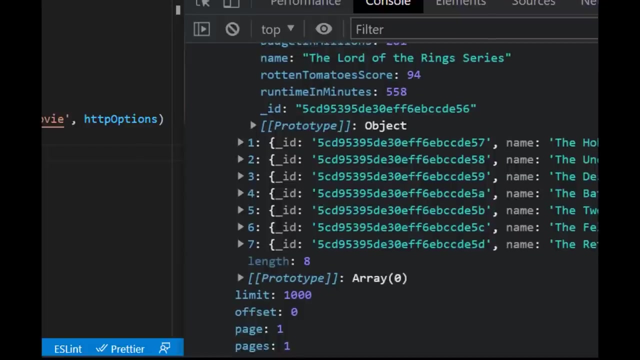 And if you try to call without passing HTTP options, you can see that we get an error. But if we add authorization, the request is successful. Congratulations, you watch all the way through the end. This was very long tutorial and I hope you learned a lot of new things. Also, don't forget to subscribe to free code camp And if